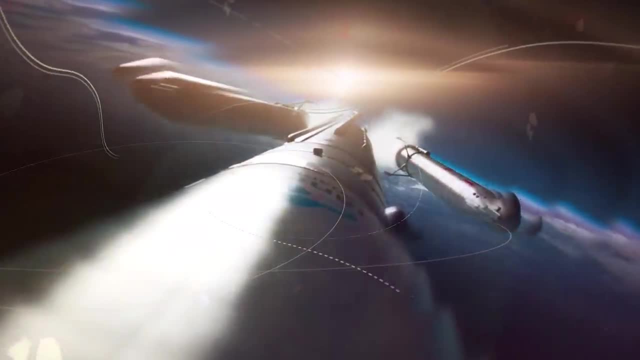 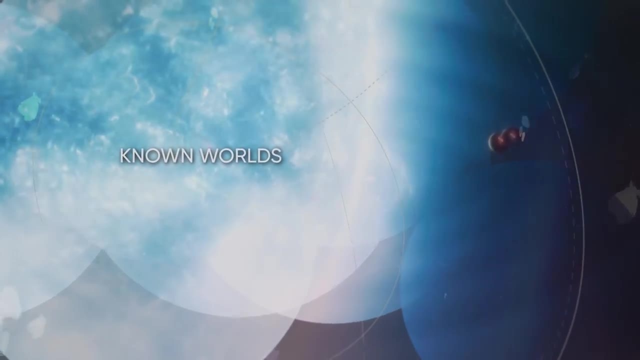 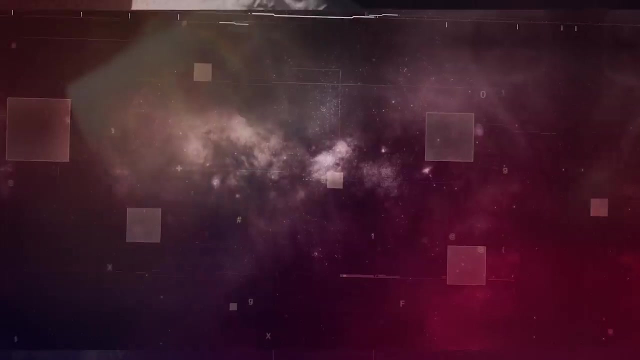 incredible, And even though humans cannot go beyond our native system at this point, we can still make a virtual dimension On our journey around the most remarkable of the worlds already known today. we will start off near the TESS Orbital Observatory, which enabled us to take a slightly deeper. 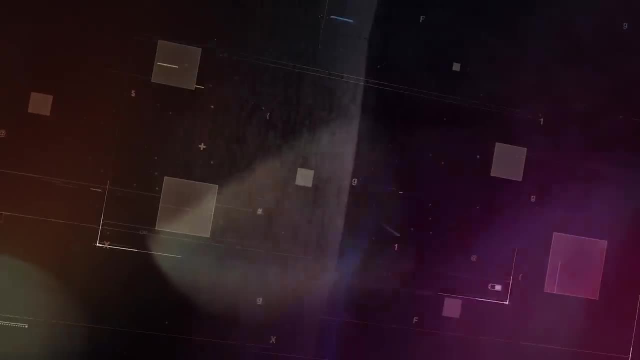 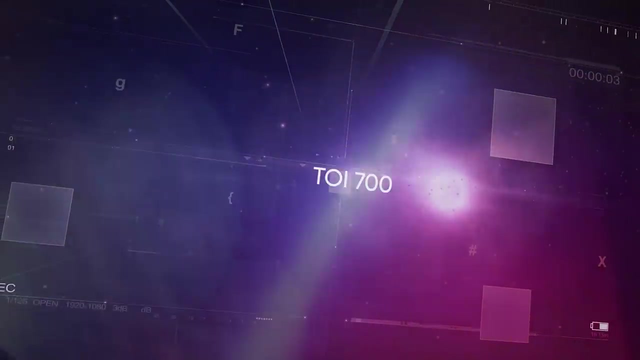 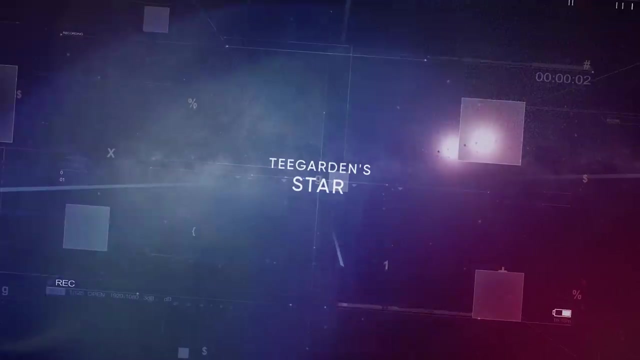 peek into the fascinating abyss of the cosmos With its help. we will visit the environs of the dim red dwarf TOI-700 to make acquaintance of its wonderful planets, potentially fit for life. After that, we will go to the Teegarden Star to observe the 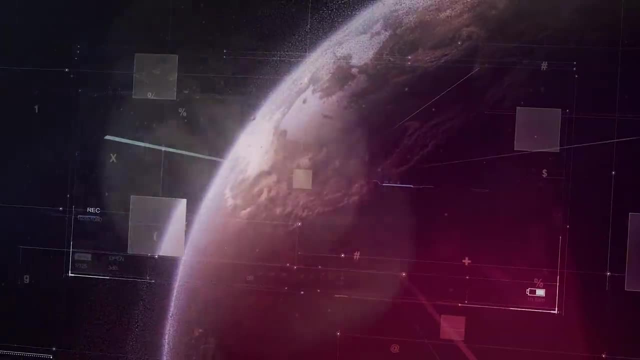 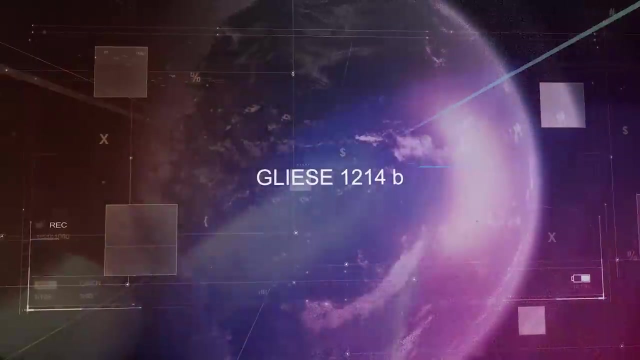 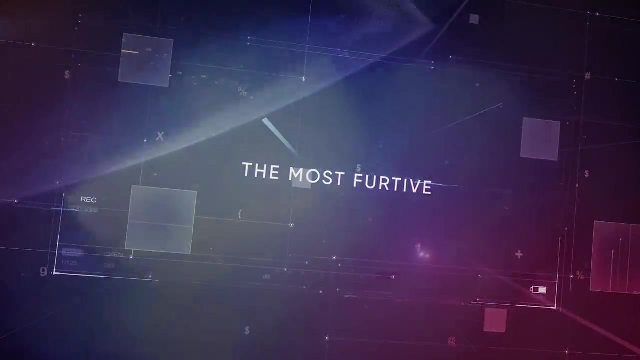 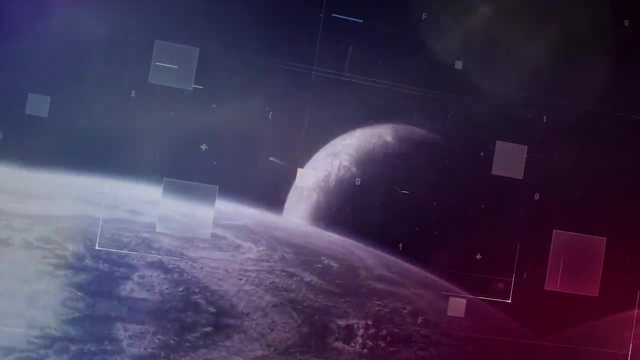 most Earth-like planet of all those discovered by now. Next in line is the bizarre world of Gliese 1214 b, which falls into the exceptionally rare category of ocean planets. Then we will reach two representatives of the most furtive and mysterious celestial objects — rogue planets Deprived of apparent stars' warmth. 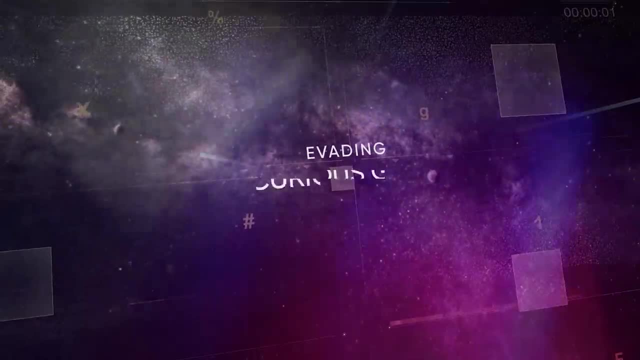 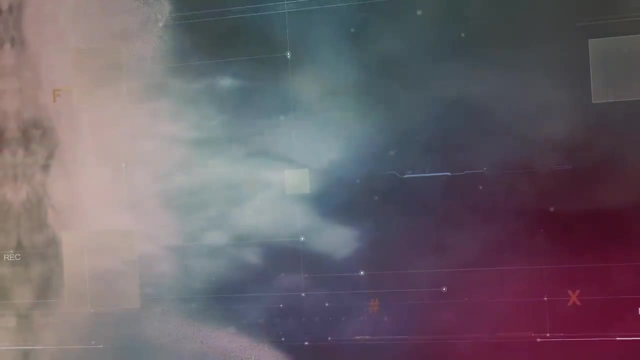 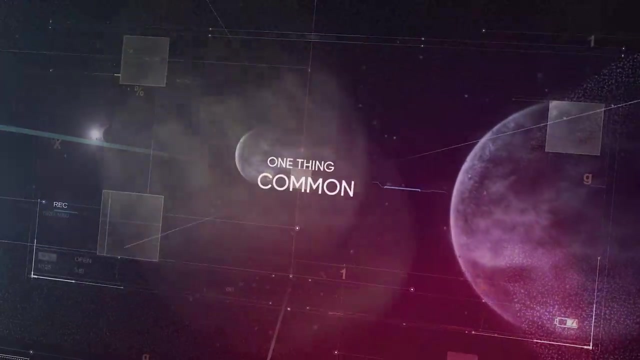 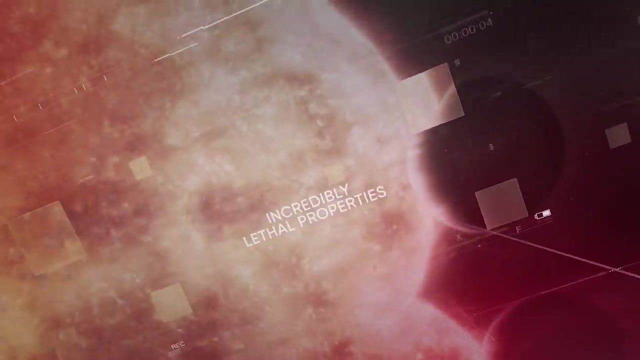 they roam the depths of space for billions of years, avoiding any chance of being discovered. After these dark and cold worlds, we will see a selection of various space objects which have one thing in common — their incredibly lethal properties, extreme temperatures, harmful radiation and a harsh environment. With all these combined, these planets are truly horrifying. 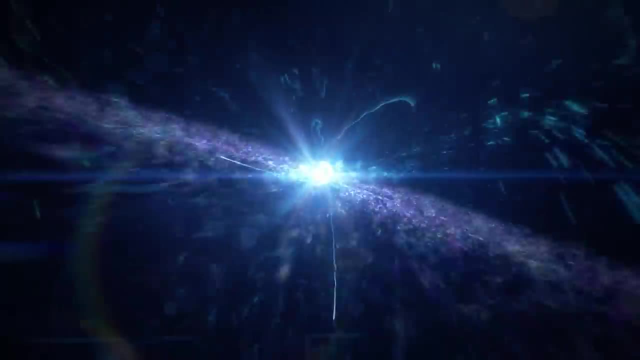 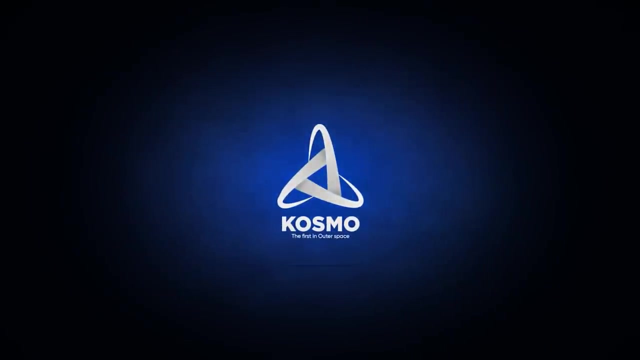 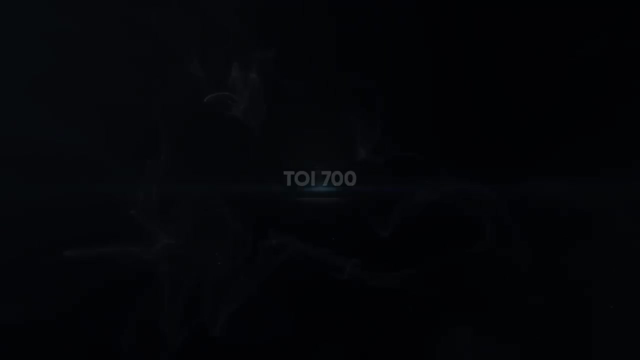 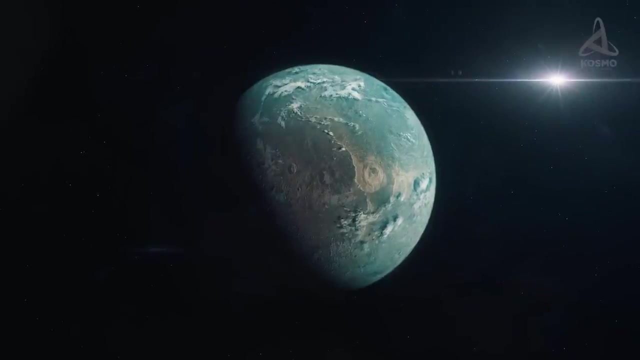 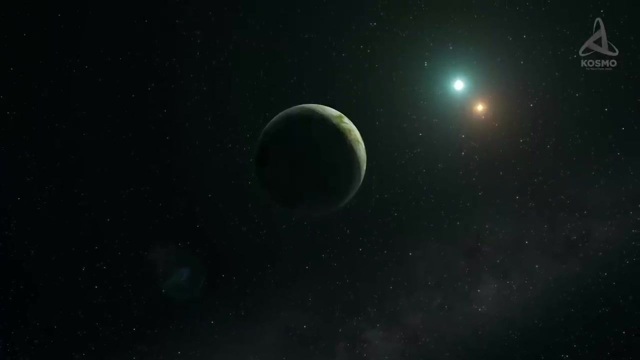 Let's get ready and we begin. Cosmo. The first exoplanets were discovered back in the late 1980s. Since then, the number of detected ones has increased hundredfold. According to statistics, from January 2021, over 4,000 planets in other systems have already been discovered. 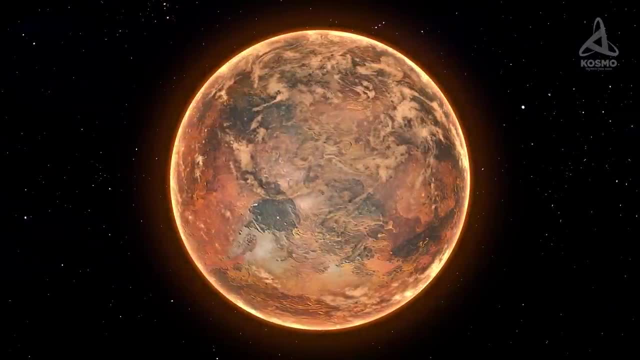 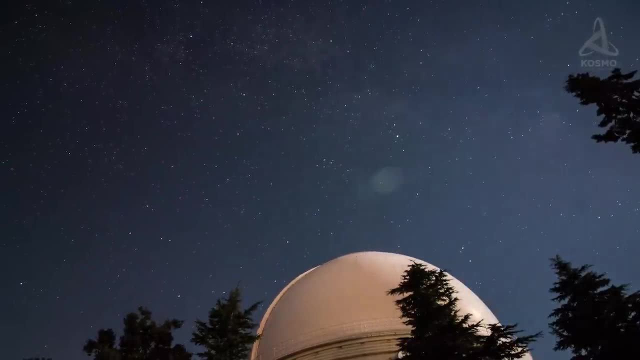 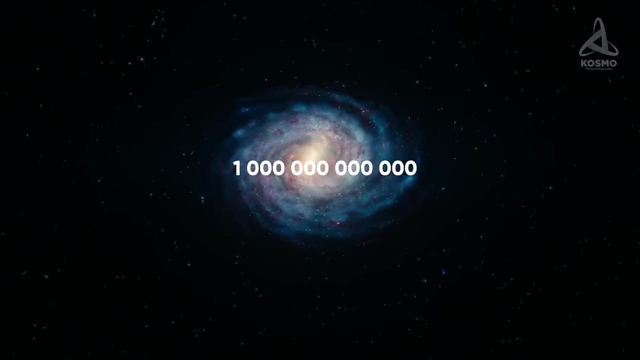 Apart from these, several thousand candidates likely to be given this status have been registered With sufficient evidence from Earth-based observatories. most of them are going to become officially confirmed exoplanets. The overall number of planets in our galaxy may supposedly be over one trillion. From 5 to 20% of these are close to our Earth in terms. 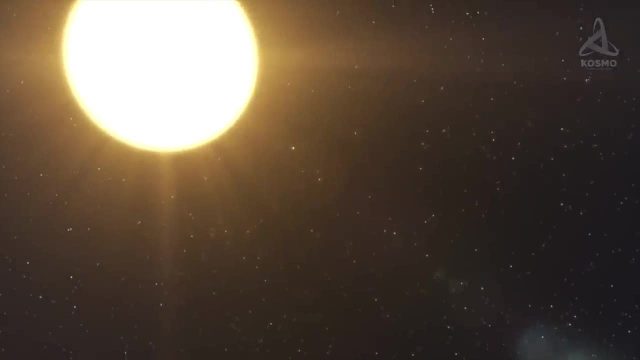 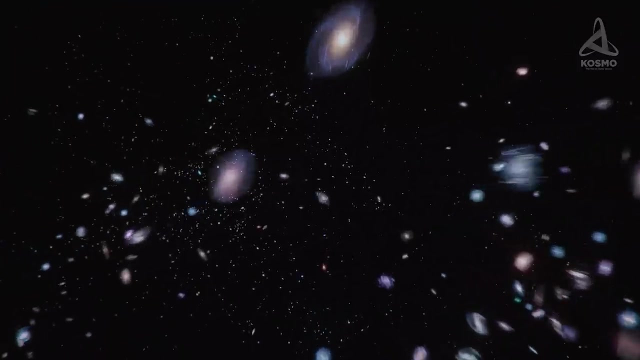 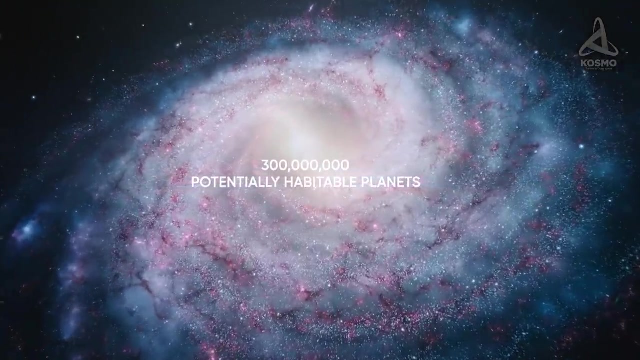 of their size and composition. Not all of them are in their host star's Goldilocks zones. that is, not all of them are habitable. Still, according to scientific estimates, there are not less than 300 million potentially habitable planets in the Milky Way. 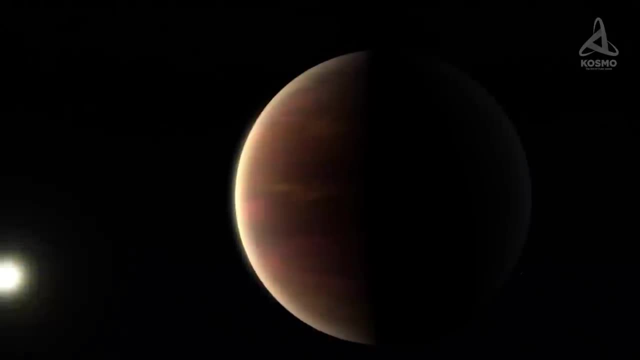 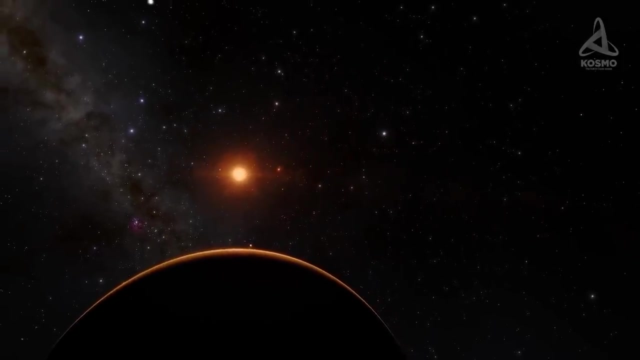 Exoplanets differ very much in terms of their environment. Their dimensions may be enormous, some even beating Jupiter, but there are also comparatively smaller ones, close to our Earth in size. Some of these bodies are hot, consumed with oceans of molten lava, whereas some of 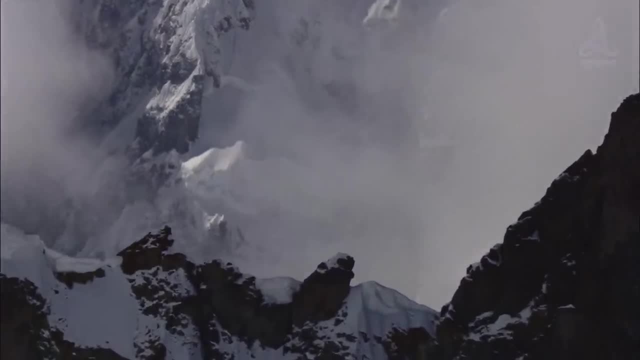 them are small and some are very small. Some of these bodies are very hot, consumed with oceans of molten lava, whereas others are encased in a shell of permanent ice. There are planets out there made entirely of oceans, with not a bit of dry land on them, while 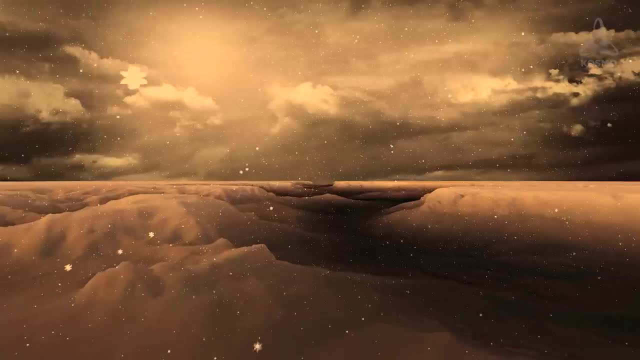 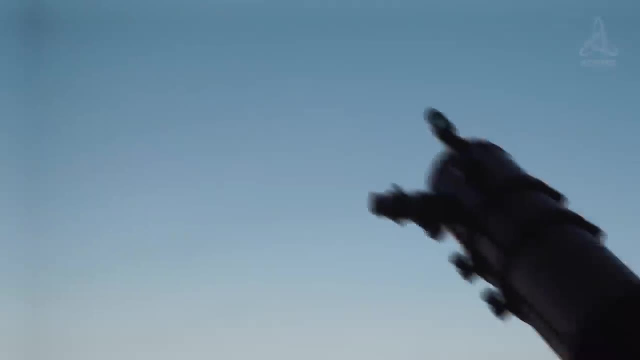 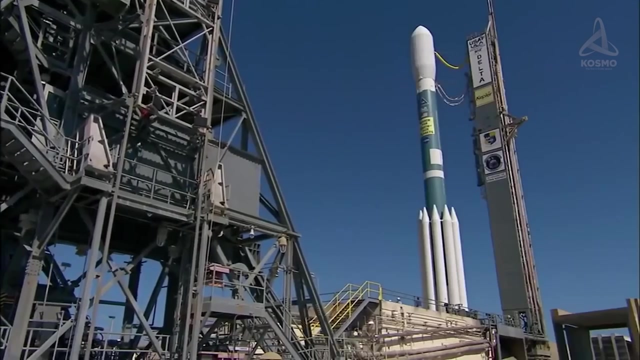 on others. sulfuric acid drains or diamond snow are a regular occurrence. Various techniques are used for discovering other worlds. As a rule, it is next to impossible to spot an exoplanet by simply looking through a telescope. That is why, in 2009,, Kepler was launched. 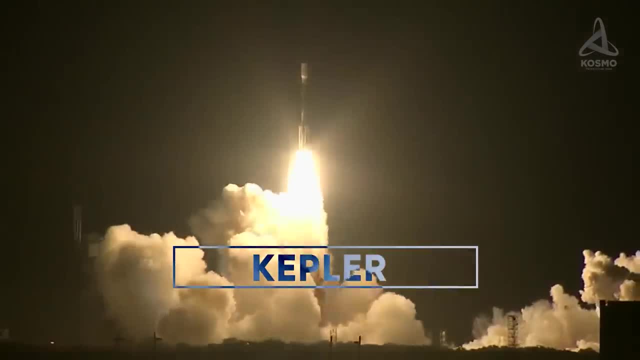 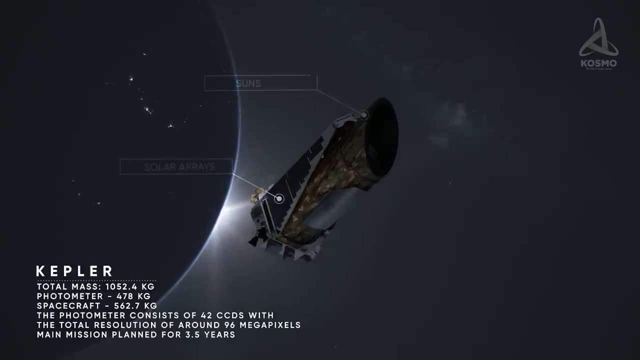 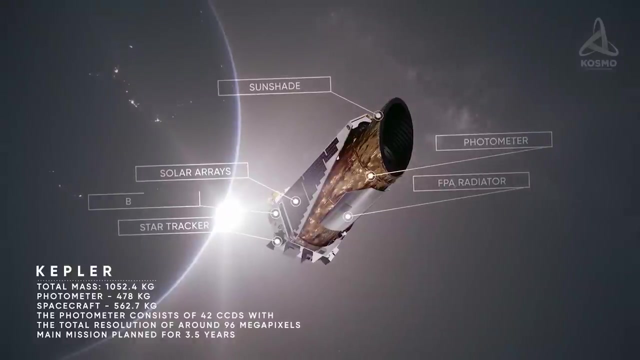 the first space telescope designed for searching for planets beyond the boundaries of the Solar system. The telescope's cameras had 42 Chart Cop assistants, or CCDs, with a total resolution of around 96 megapixels, with a field of view covering about 25% of the sky, and coupled 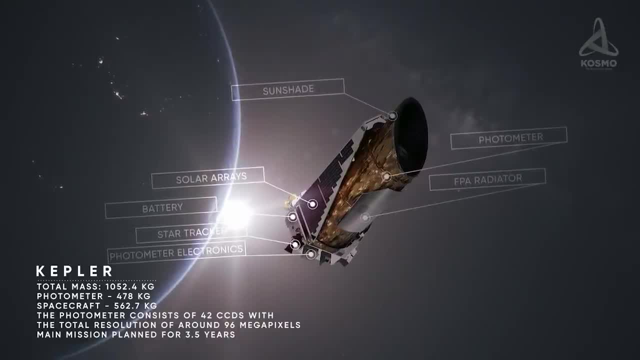 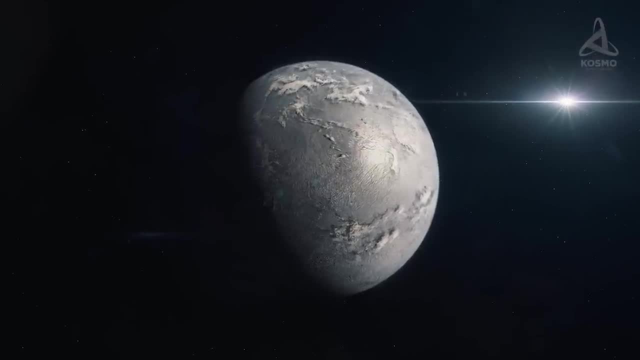 with a one-and-a-half-meter mirror of the telescope, it was able to detect astronomical bodies within 3,000 light years from the Earth. своим옷 believe. After three and a half years of productive operations, Kepler managed to spot over three. 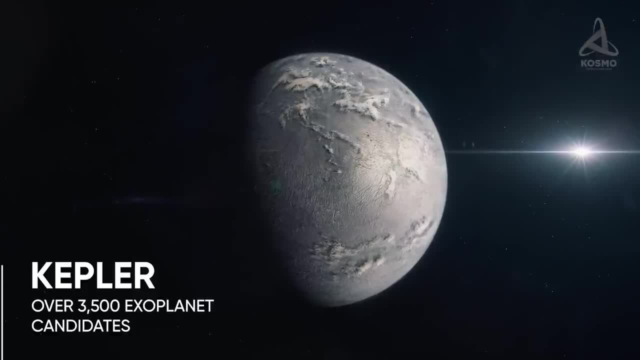 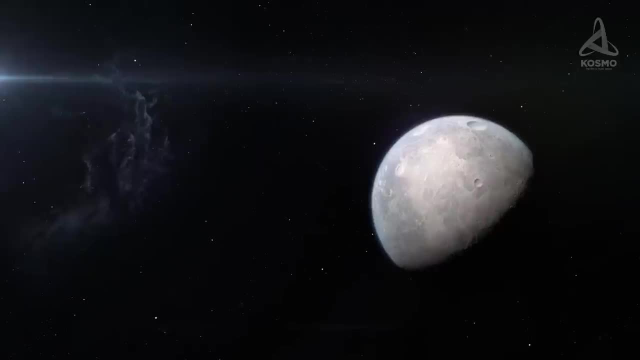 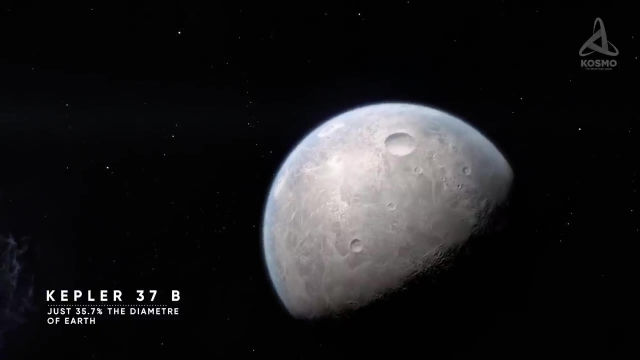 and a half thousand exoplanet candidates. The status of over two thousand of these has already been confirmed by repeated observations. It was in this period that the smallest of known exoplanets today was detected. The diameter of Kepler-37b is just 35.7% that of the Earth. 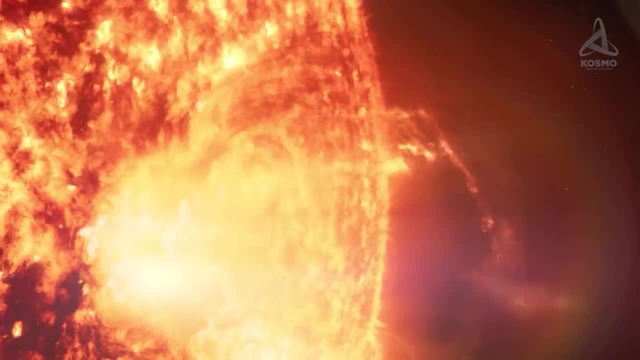 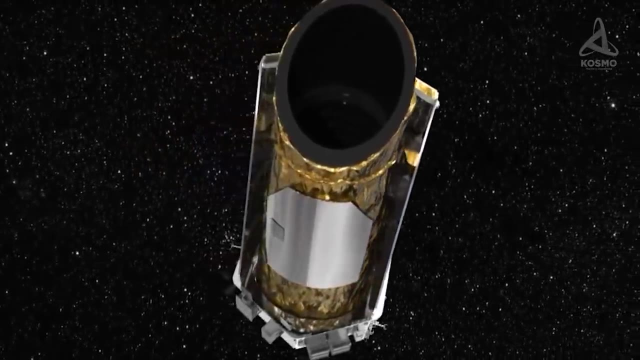 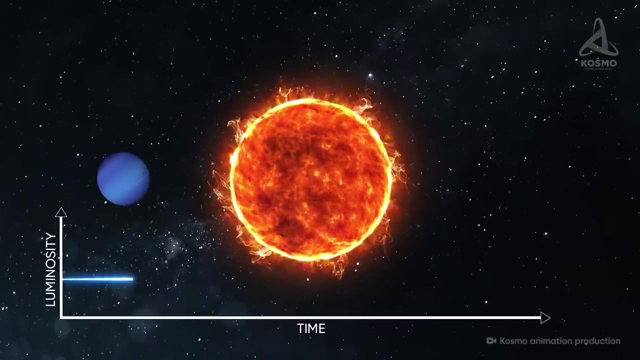 The telescope was also instrumental in registering several stars and brown dwarfs. The transit method was used by Kepler in the search for exoplanets. This method is based on observing the star's luminosity. If the supposed planet passes between the parent star and the observer, this will be. 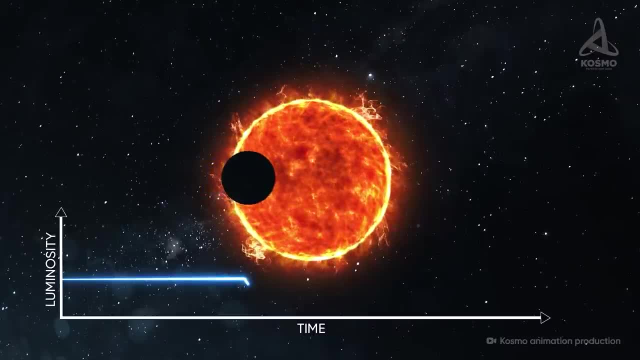 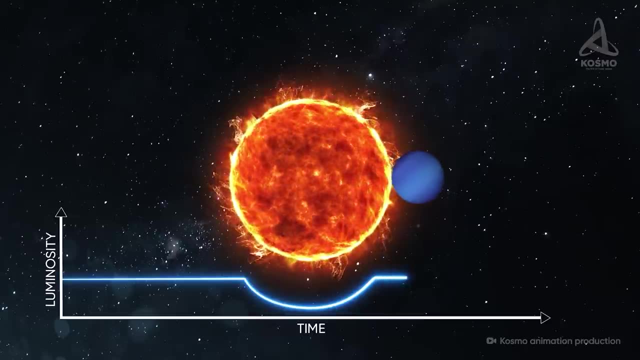 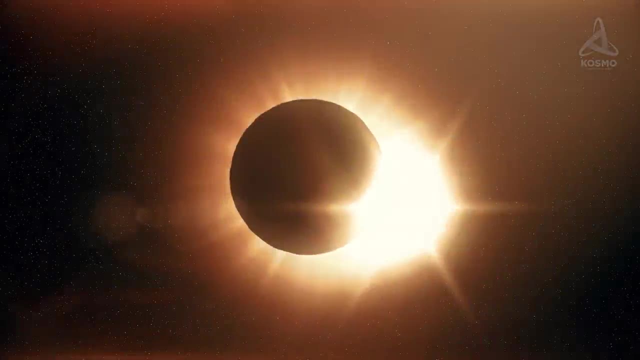 noticed in the telltale decrease in the star's luminosity. The extent of these fluctuations in luminosity directly depends on the ratio of the star's and planet's dimensions. While their regularity allows one to estimate the object's orbital period, The transit method requires accuracy in measurements. 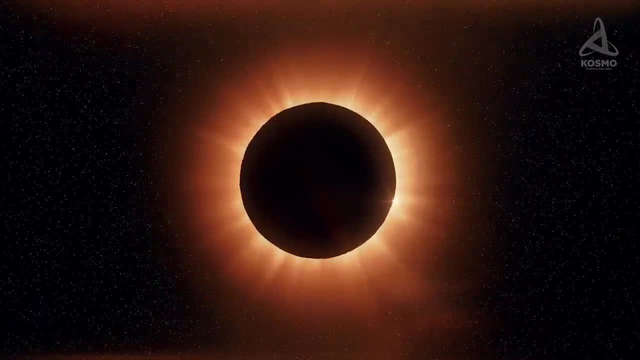 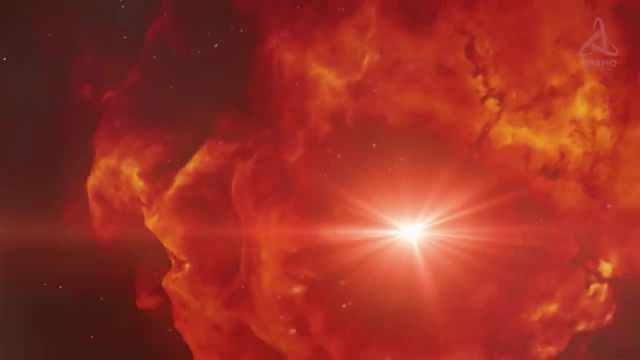 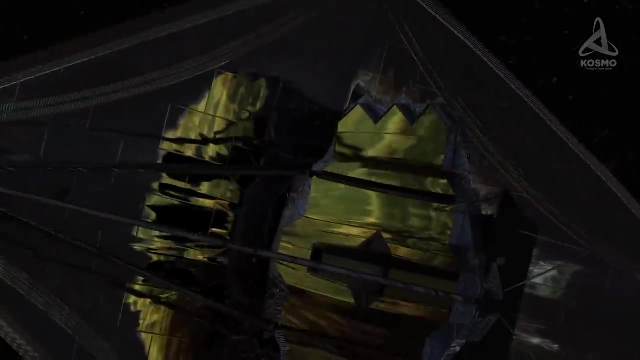 Changes in a star's spectrum account for less than two percent and are usually tenths or even hundredths of one percent. Ripples in the atmosphere, dust and precipitations negatively affect results produced by Earth-based telescopes. That is the reason why telescopes based on automatic space stations are used for searching. 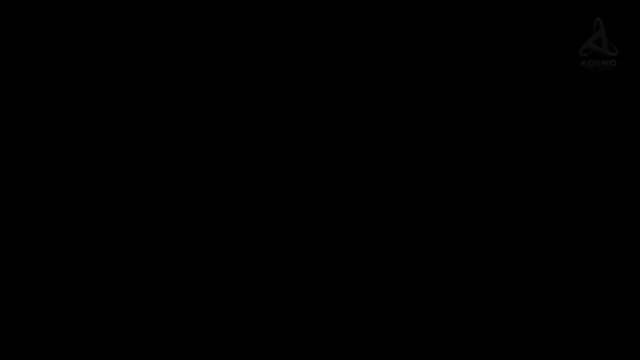 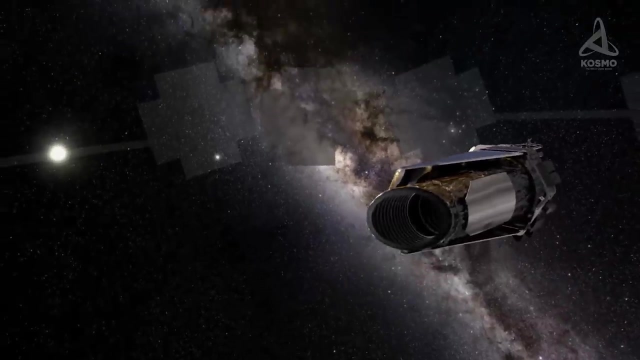 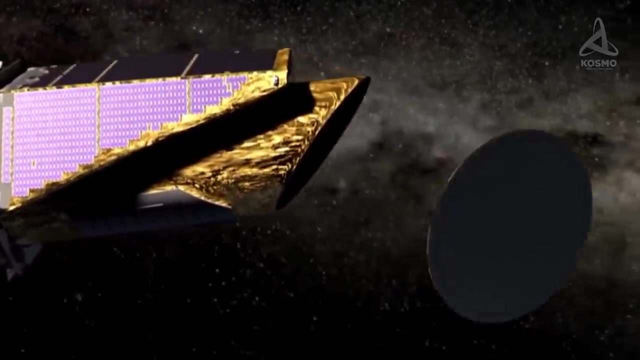 for objects. It's beyond the boundaries of the solar system. Unfortunately, in 2013,, three and a half years into the mission, the Kepler Space Telescope had several major equipment failures. In 2018, the spacecraft ended science operations completely. 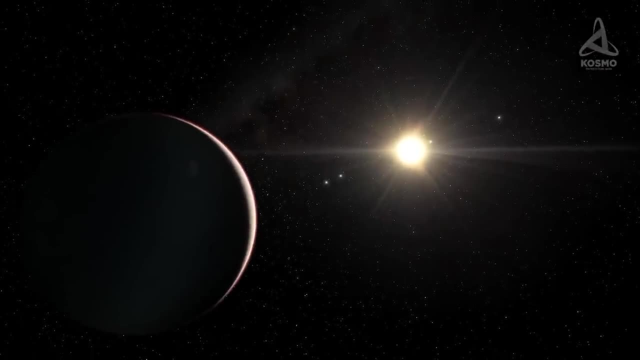 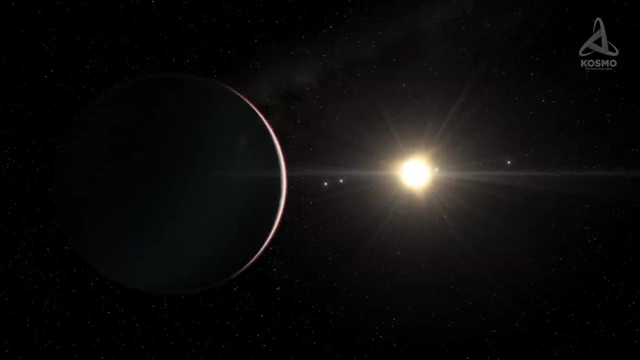 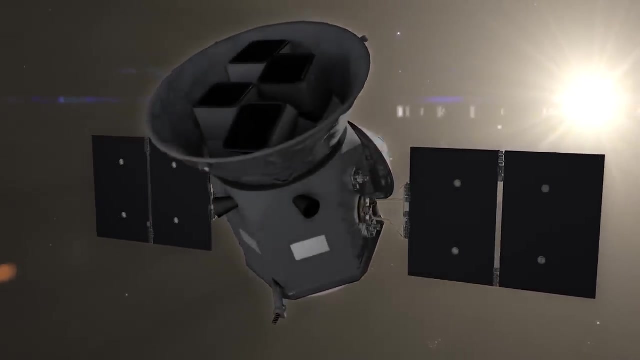 Kepler was the first spacecraft to be created specifically for looking for exoplanets. However, most of the objects it managed to spot happened to be too remote and dim to study them in any satisfying detail. That is why the next space research complex had slightly different parameters. 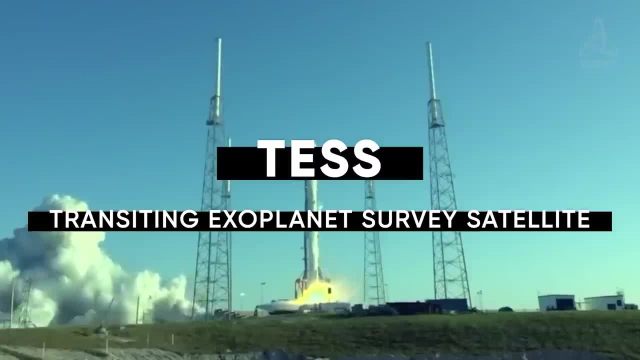 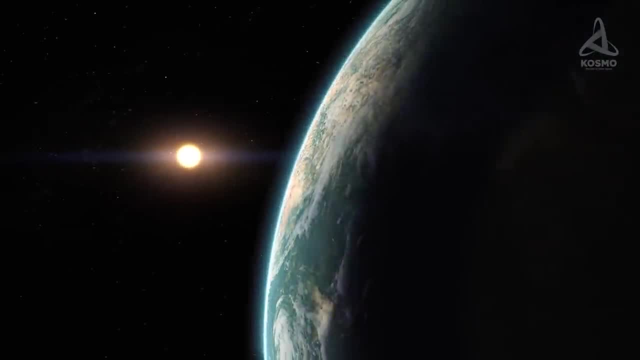 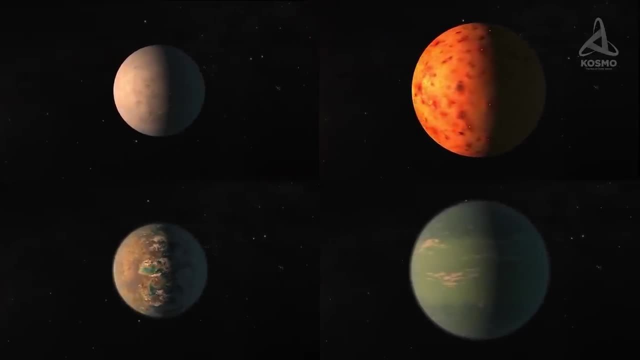 Kepler was succeeded by the TESS telescope, launched by NASA on the 18th of April 2018.. Its main object was searching for rocky exoplanets orbiting the brightest stars within 200 light-years from the Sun. This telescope also used the transit method. 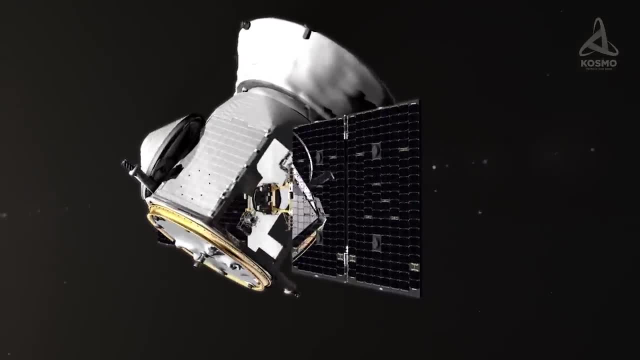 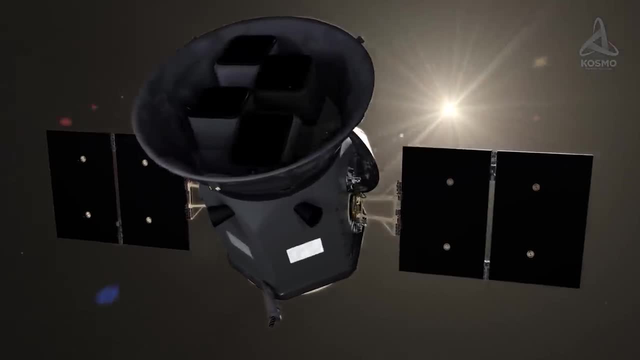 And here is the spacecraft's brief profile. TESS is the first spacecraft to use the transit method. TESS is equipped with four refractors with a 24 by 24-degree field of view and a 10-centimeter aperture. The spacecraft's peculiar orbit allows it to cover both the northern and the southern. 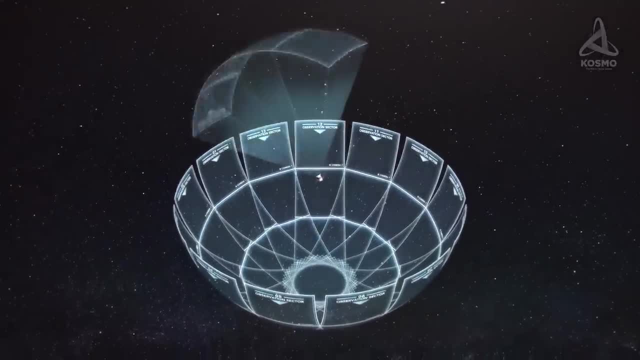 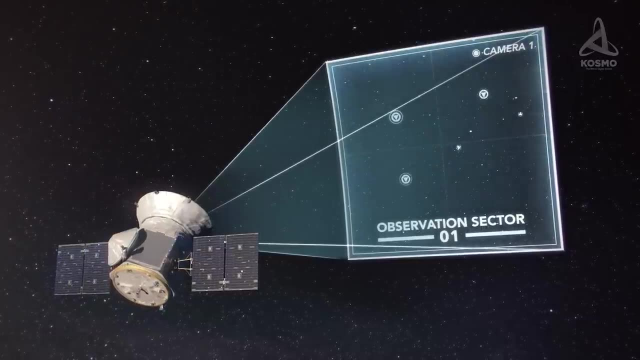 parts of the sky, which is approximately 85% of the entire sky. Photos are taken by four cameras, and the resolution of each camera's CCD is 16.8 megapixels. TOI-700D is one of the most known cameras in the world. 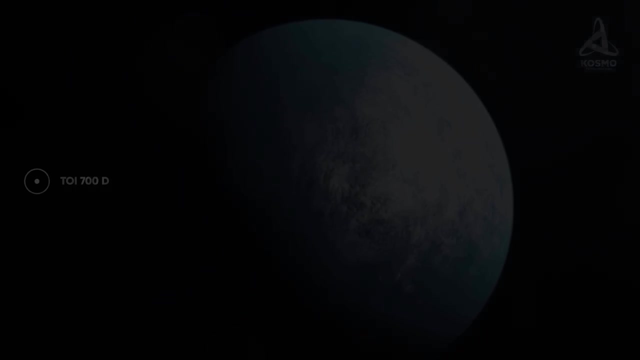 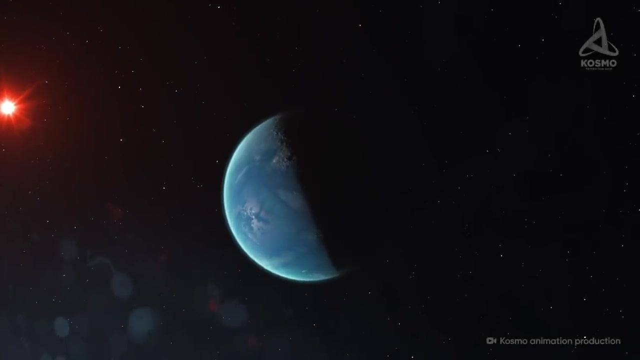 TESS is one of the most known cameras in the world. TESS is one of the most known cameras in the world. TESS is one of the most known cameras in the world. This exoplanet became the first object of the kind comparable to the Earth in size and 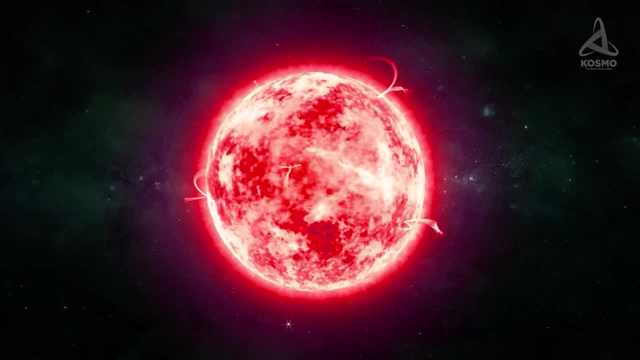 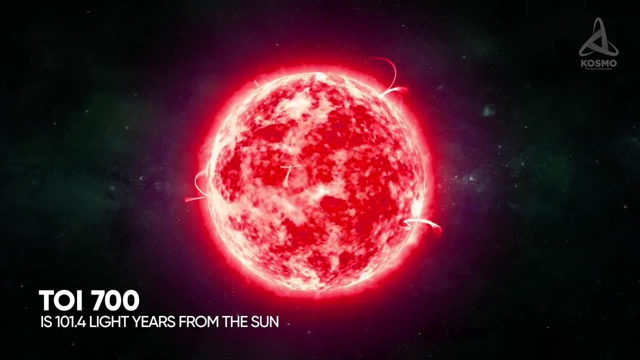 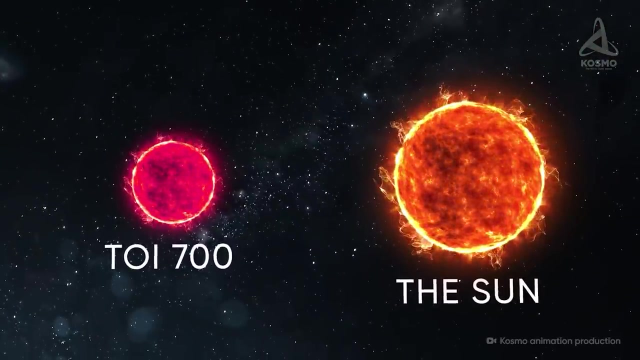 which found itself in the habitable zone of its star. It orbits TOI-700,, a red dwarf lying slightly over a hundred light-years away from the Sun. It is a small and rather cold star. Its temperature is half that of the Sun and its mass and radius are just 40% those of 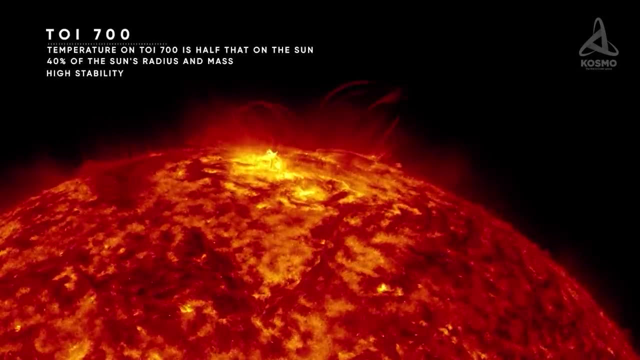 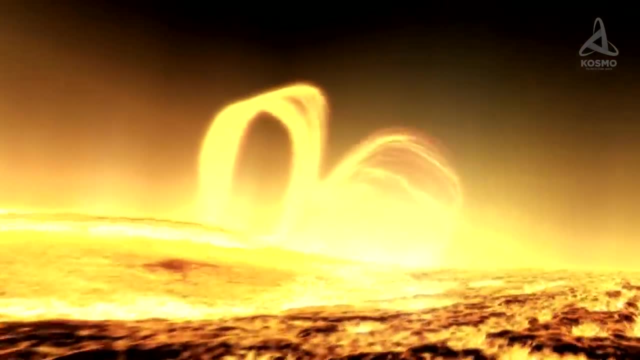 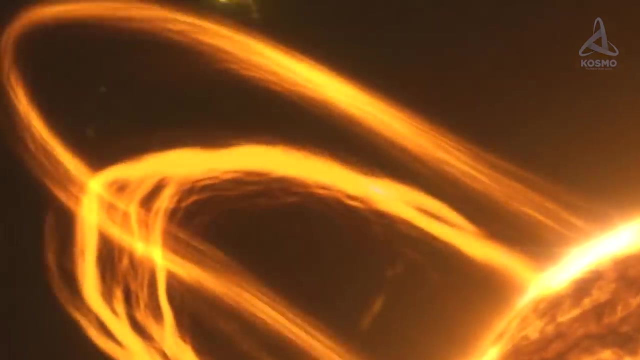 the Sun. TOI 700 is peculiar for its high stability. Not a single flare has been registered on it since the beginning of observations. A star's stability is a positive feature because bursts of activity are able to divest its planets of their atmospheres and be generally. 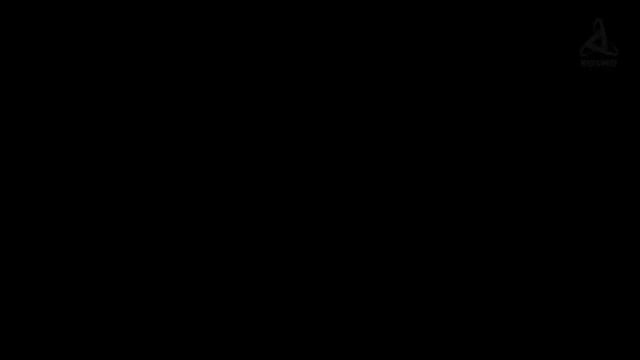 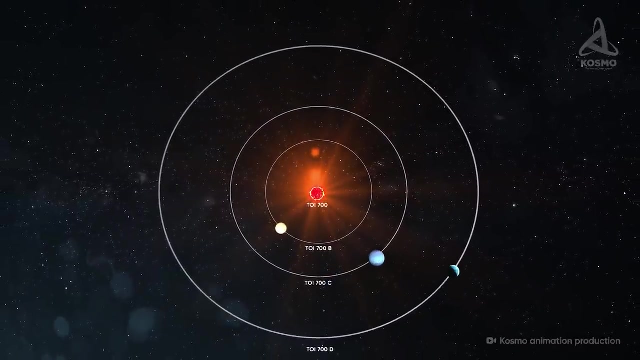 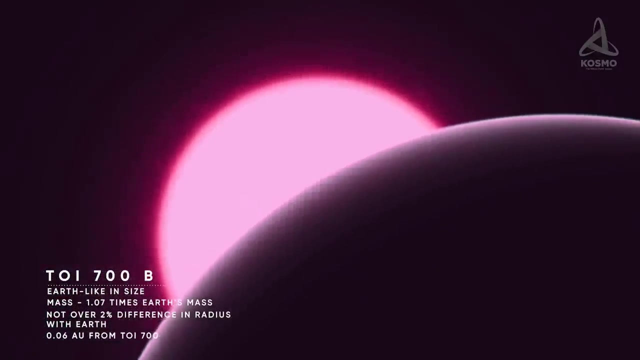 pernicious for potential life on planet's surfaces. There are at least three planets orbiting TOI 700.. The one closest to it, TOI 700 b, is comparable to the Earth in size. Its mass is approximately 1.07 times that of our planet, and its radius differs from. 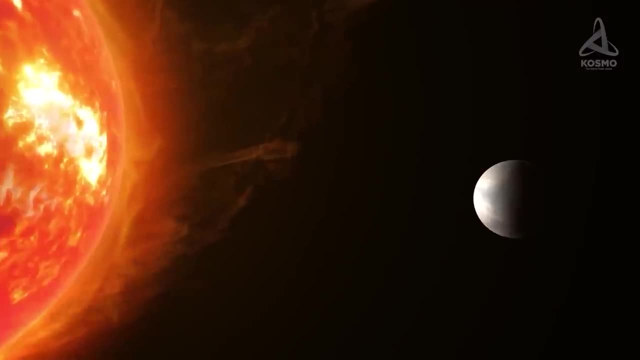 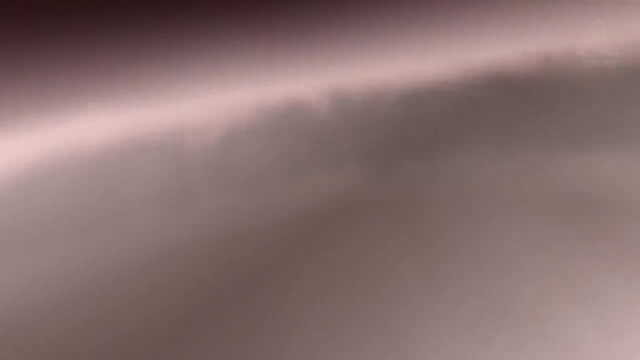 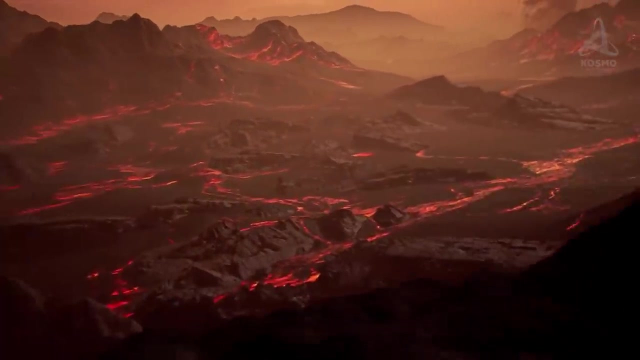 that of the Earth by not more than 2%. Unfortunately, TOI 700 b is too close to its host star. It is within about 0.06 astronomical units, and a year on the planet lasts just 10 days. In addition to that, chances are it is tidally locked, that is, it faces the star with one. 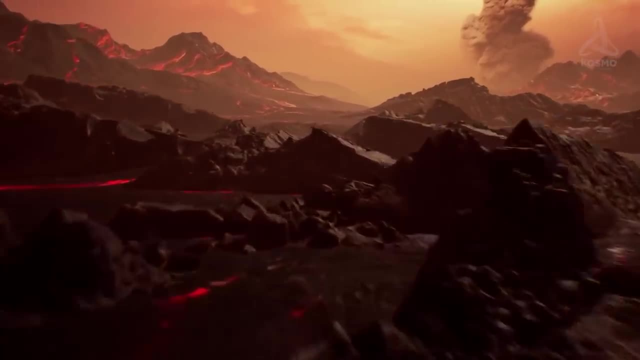 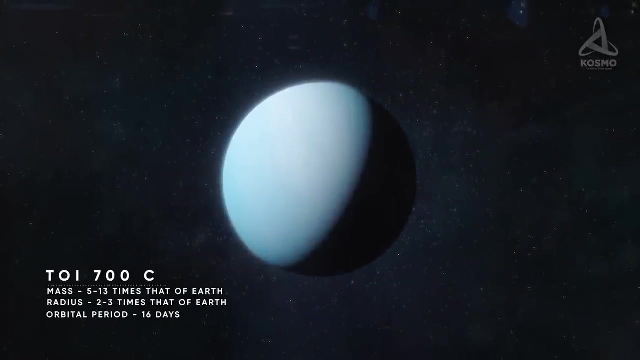 in the same side. This means that the planet is likely to be scorching hot. The planet lying further from its star, TOI 700 c, is thought to be a mini-Neptune. Its mass may be from 5 to 13 times that of our Earth, and its radius is 2 or 3 times that of the Earth. It takes TOI 700 c 16.7 times that of the Earth. This means that the planet is likely to be scorching hot As far as the planet lies. TOI 700 c is thought to be a mini-Neptune. Its mass may be from: 3 to 12 times that of our Earth, and its radius is 2 or 3 times that of our Earth. As far as the planet lies, TOI 700 d is thought to be a mini-Neptune. Its mass may be from: 5 to 14 times that of our Earth, and its radius is 2 or 3 times that of the Earth. Its mass may be from 5 to 15 times that of our Earth, and its radius is 2 or 3 times. 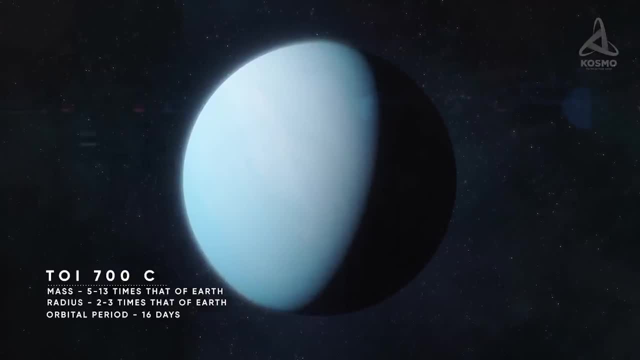 that of our Earth. Is Bohr ever found? The observatory will surely record traces of the muitoях Ito Lunar Scroll ´ horizon down above and cerc愛 around its host star, Located closer to the star than the inner border of the habitable. 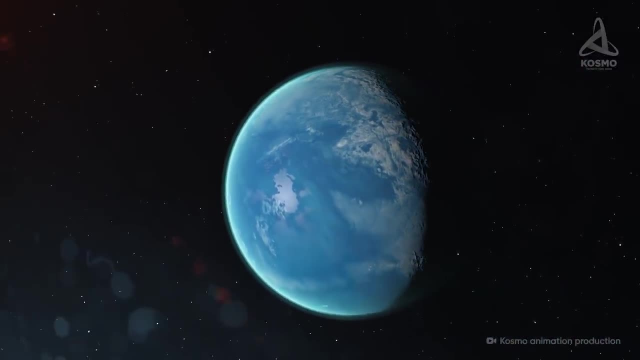 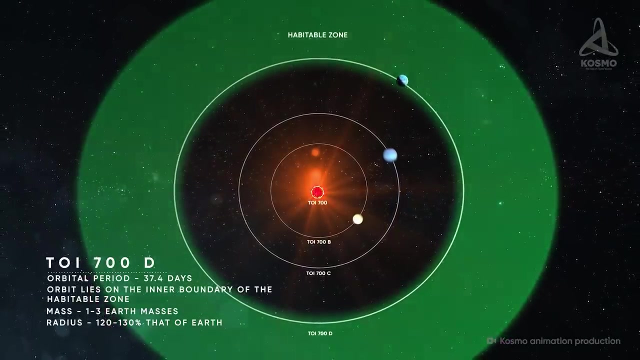 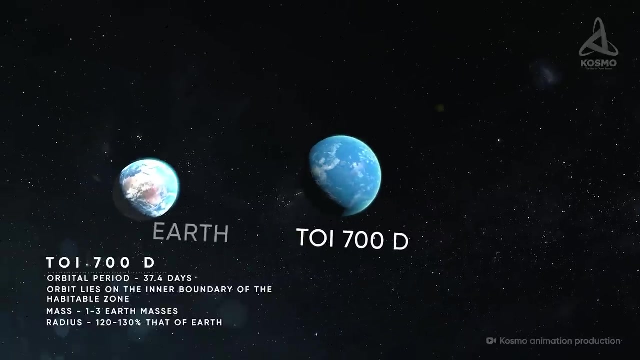 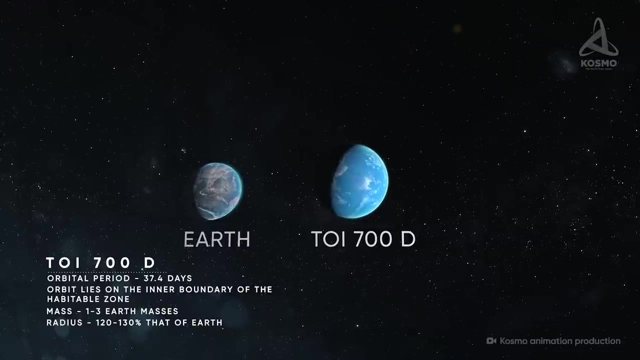 zone. it must be too hot for life to originate and evolve there. ート cilantro, transport, County, County expo Air Washington State 15, Think been gauged precisely and may be anything from 1 to 3 times that of the Earth. At the same time, the planet's radius is just 20 to 30% bigger than that of the Earth. 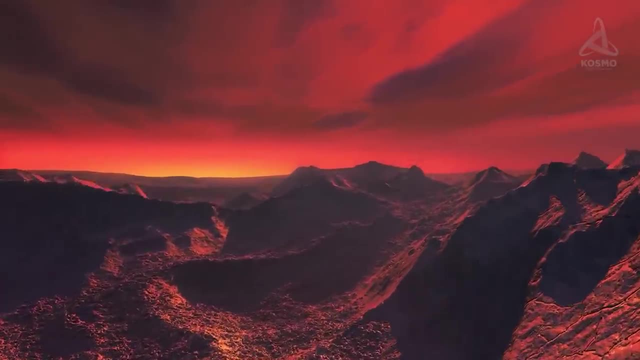 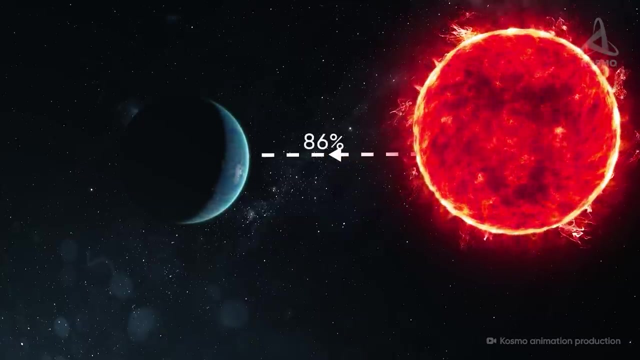 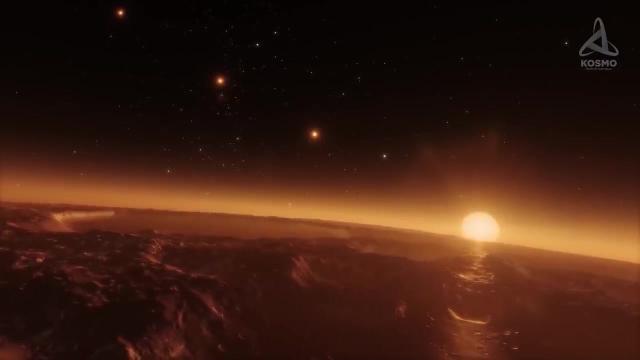 TOI 700 d is thought to be a rocky world, but its exact composition is not yet known. The amount of energy received by the planet from its star is 86% that of the amount we receive from the Sun. Assuming the planet's atmosphere is similar to ours, the steady-state temperature on the 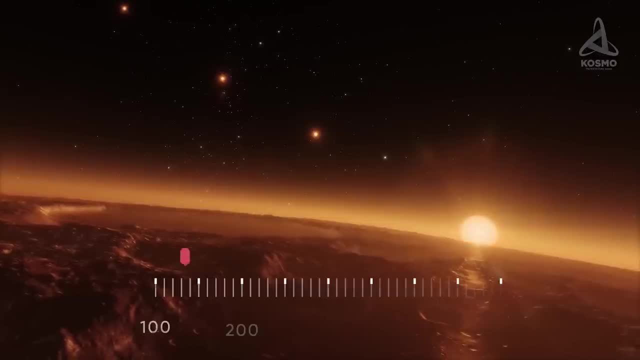 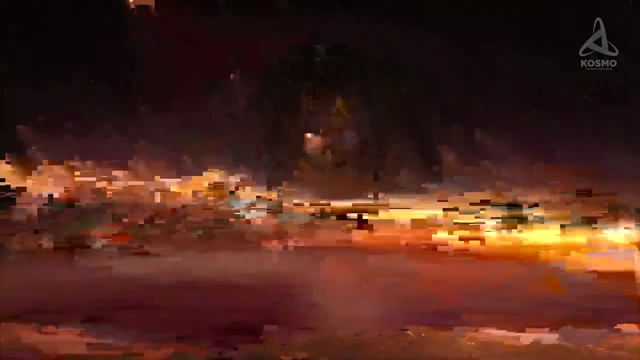 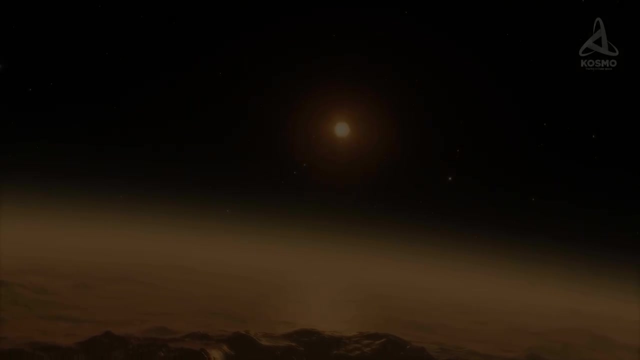 surface of TOI 700 d is estimated at 268.8 Kelvin, or 4.3 degrees Celsius below zero. However, due to the greenhouse effect or other features of the atmosphere, we may not know yet- this figure may shift either up or down. 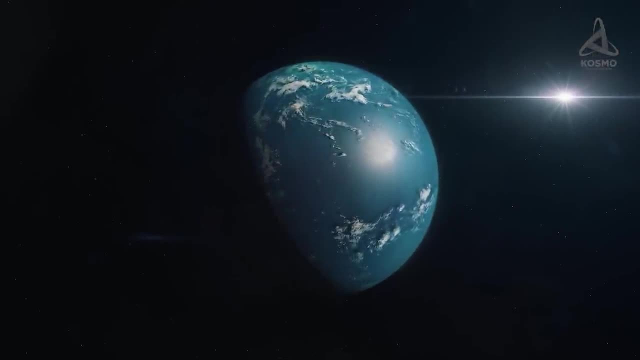 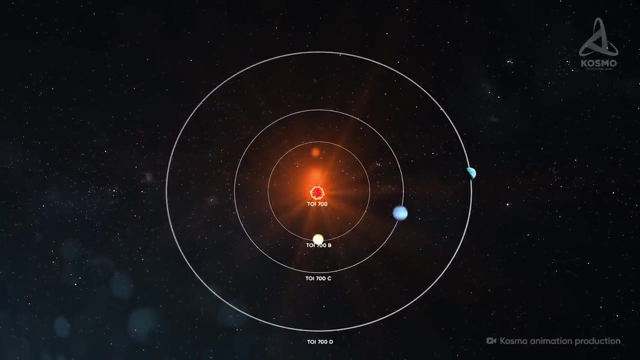 There is no precise data on the eccentricity of TOI 700 d, but it is thought to be small, at around 1.5 times the current, As the planet's orbit finds itself at the inner edge of the Godelok zone, the planet's 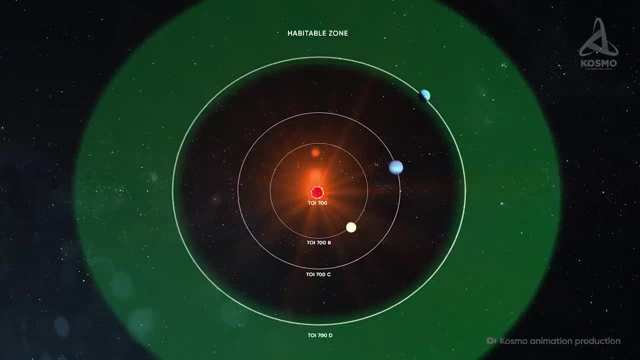 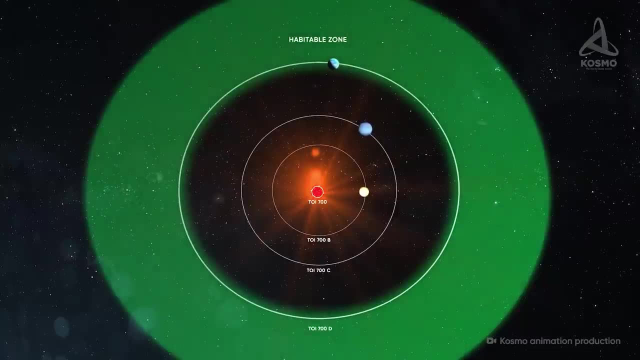 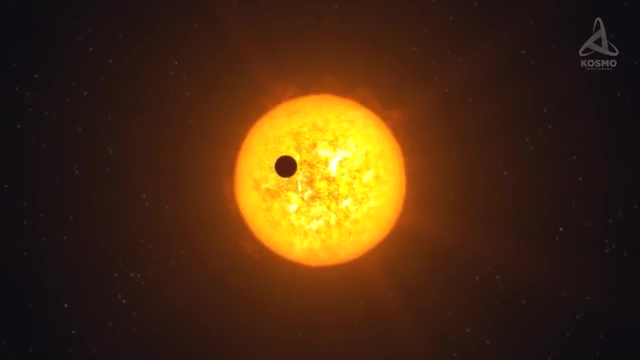 eccentricity, however small, may, incidentally, turn out to be perceptible when the planet comes too close to its star from time to time, thus actually leaving the habitable zone Still. with a year on the planet lasting slightly over one Earth month, such unfavourable periods. 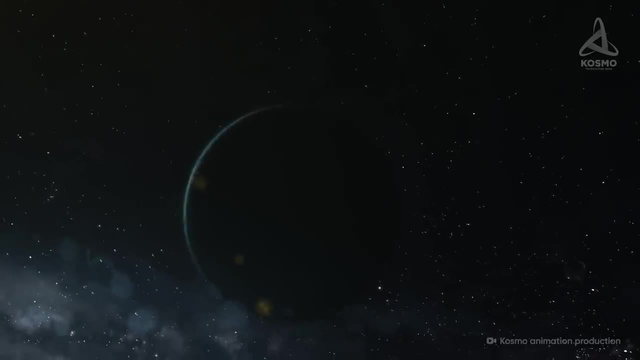 are expected to be rather short. If there are living creatures on TOI 700 d, the planet will have a short life span. If the planet is not in deep water, they will not be able to survive the harsh spells, and in the presence of a weak host of animals it is likely to become more dangerous. 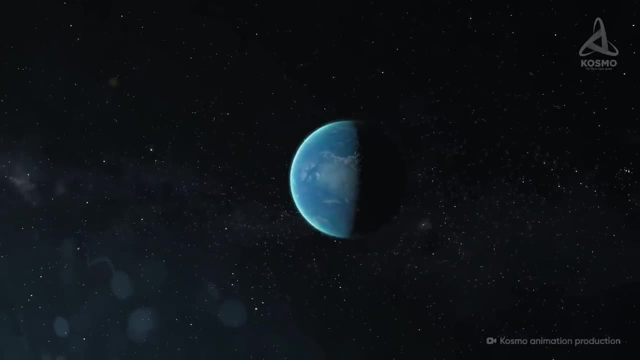 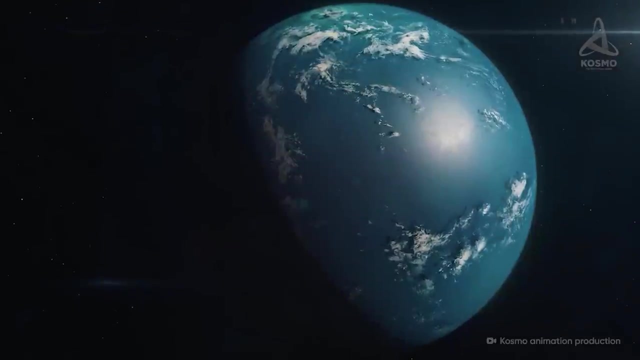 Then they might be able to weather the harsh spells in a state of anabiosis. Alternatively, they could adapt or migrate to less inclement areas, Even though the data acquired by spectral analysis of TOI 700 d can't be enough for. making conclusions. there is a chance that there is liquid water on the planet's surface. Then there is bound to be the greenhouse effect too, which will help the surface temperature to reach favourable values. As I've already mentioned, TOI-700D, along with the other known planets in the system. 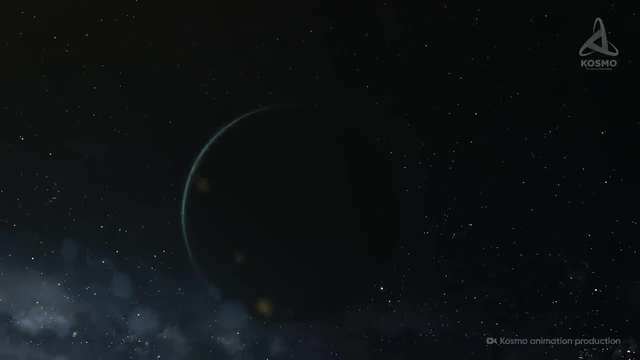 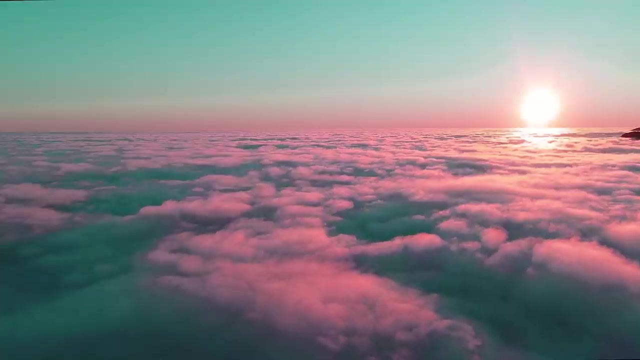 is highly likely to be tidally locked to its star. If this is the case, there should be a stark difference in temperatures between the sunny side and the shadow side. This contrast could be leveled off by a dense atmosphere, but that would cause powerful 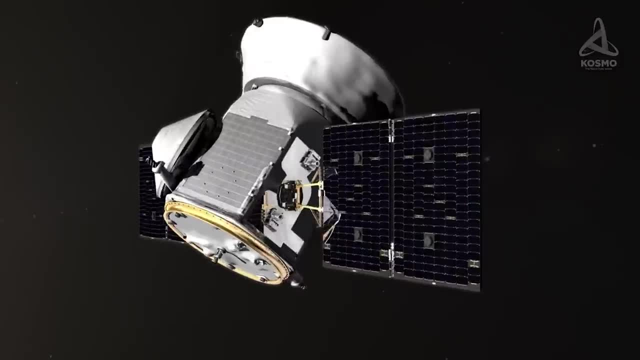 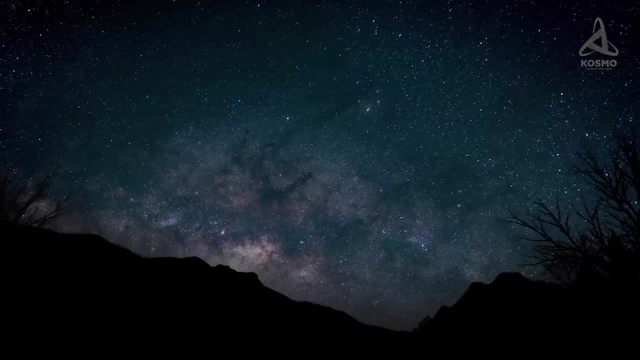 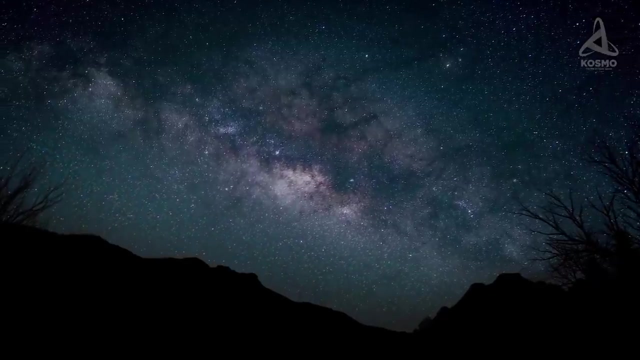 hurricane winds. Although the main mission of TESS has been accomplished by now, it still has enough resources to carry on operations. The telescope will continue taking snapshots of the sky, including the Milky Way plane, which is the most challenging direction for observation. 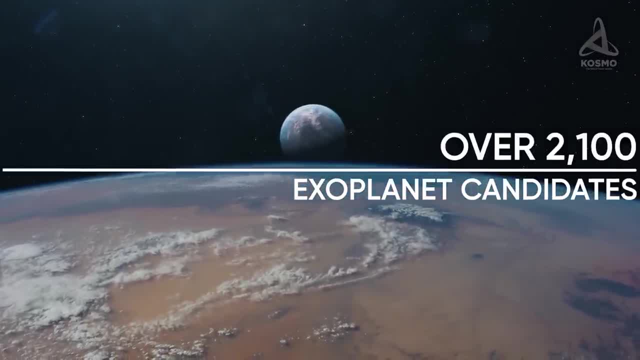 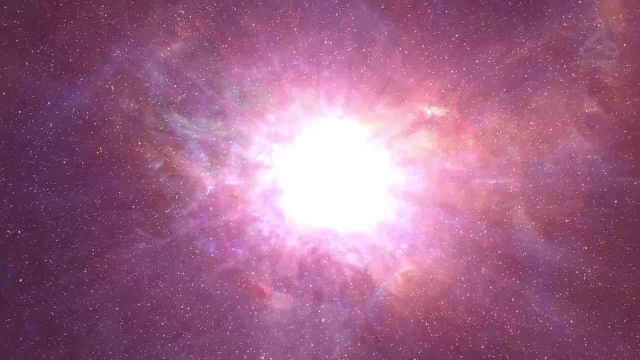 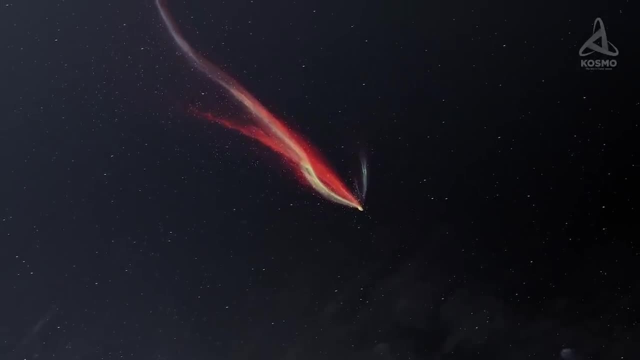 Over 2,100 exoplanet candidates have been discovered by TESS in the course of the main mission. Not less than 66 of them have already been confirmed. Apart from that, six supernovae flares have been registered. three exo-comets identified. 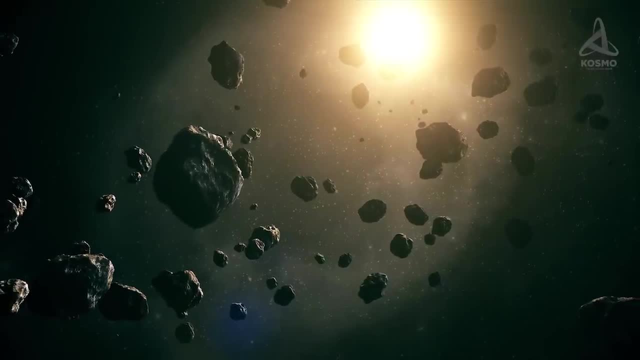 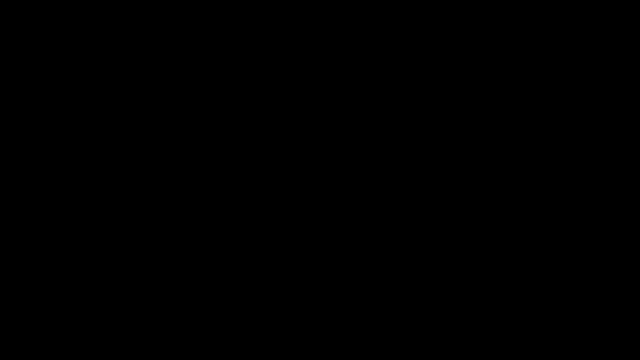 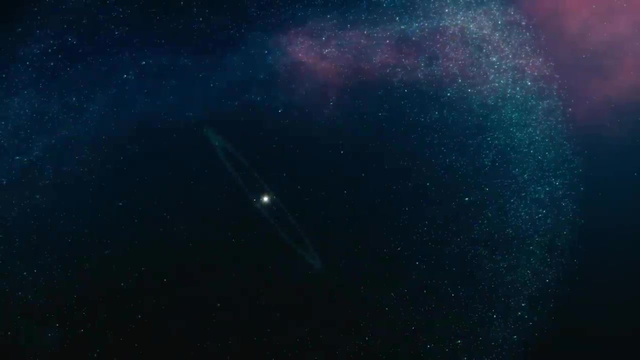 and a great number of exoplanets have been discovered. There were a great number of photos taken of small bodies in the Solar System. The latters were not objects of the main mission but are, of course, of scientific interest. Before we set out on a space journey beyond the boundaries of our system, we have to decide. 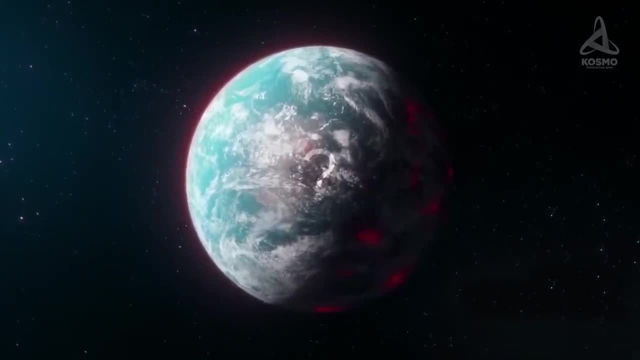 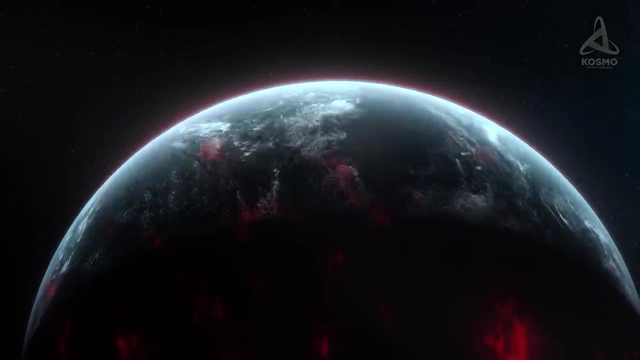 on the manner of selecting a planet that resembles the Earth most from thousands of candidates. What should be the parameters of this fascinating work, What would be the parameters of the space journey beyond the boundaries of our system world, and what should be taken into consideration first? 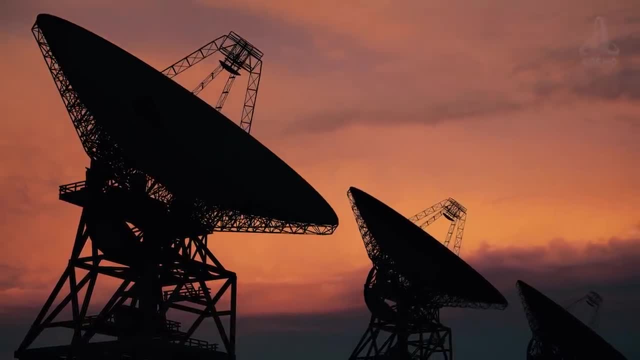 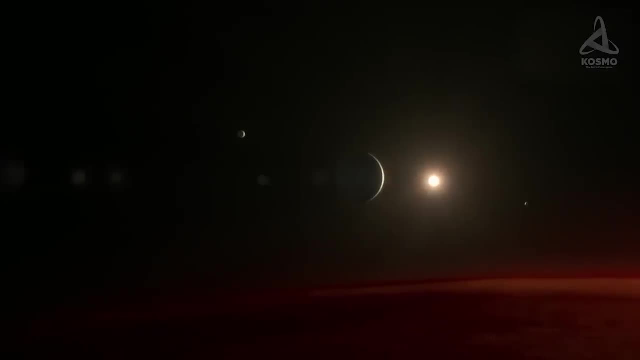 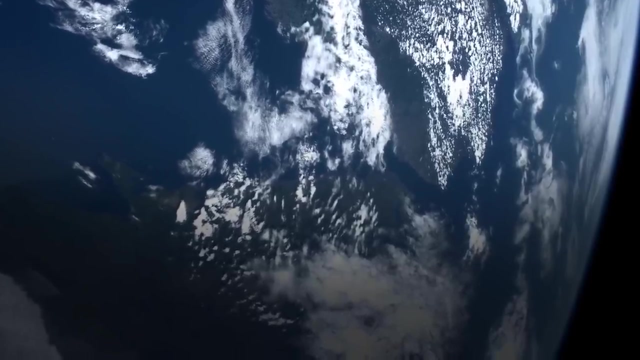 It goes without saying that planets favourable for the genesis and sustenance of life have always posed considerable interest to scientists. However, it is no easy matter to single out suitable celestial bodies among a great number of those discovered by now. To have clear-cut selection criteria, scientists worked out the so-called Earth Similarity. 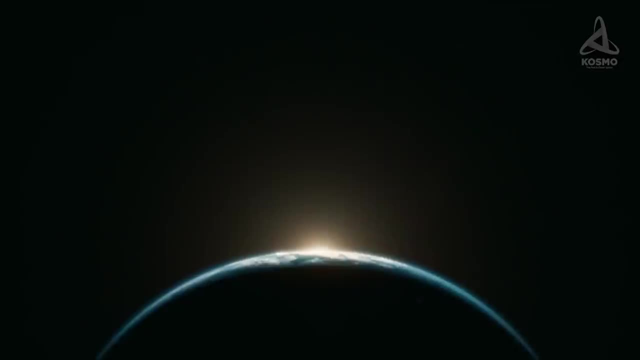 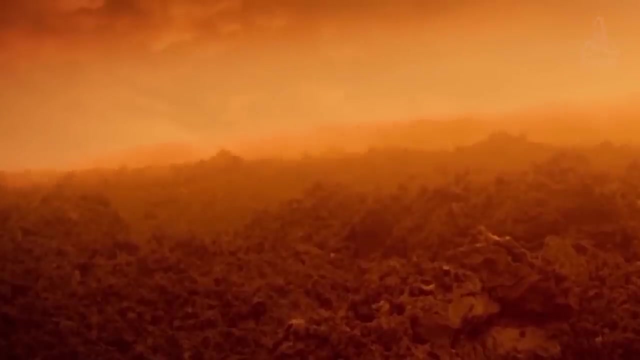 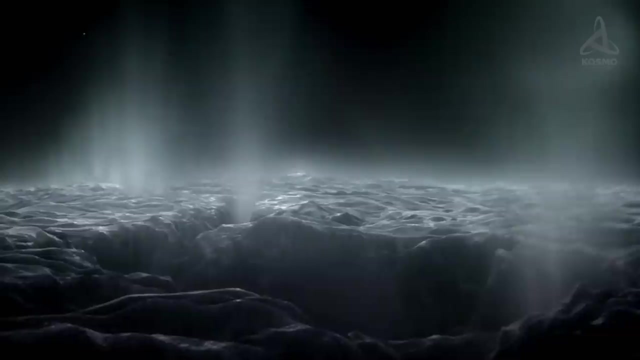 Index, or ESI for short. It is based on several principal parameters – a planet's radius, density and average surface temperature. This combination makes it possible to calculate the object's mass approximately, estimate its chemical composition, gravitational level, whether or not there is an atmosphere and 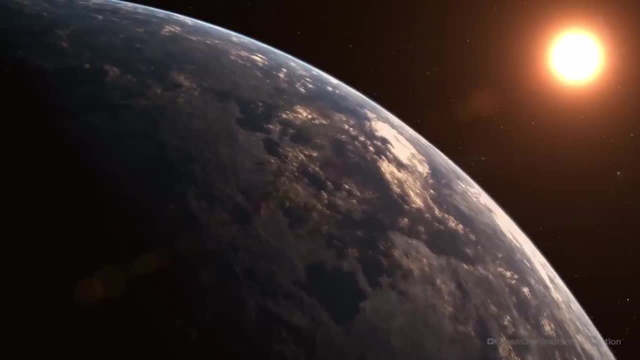 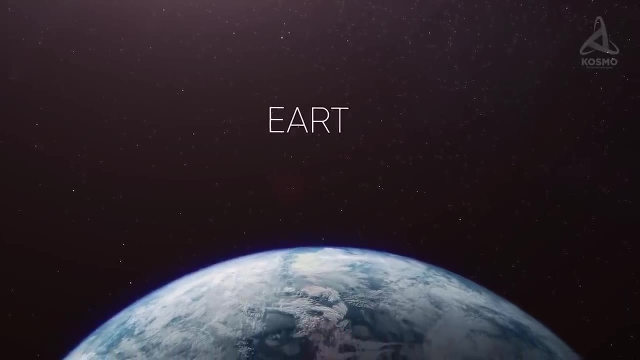 if there is, analyse some of its characteristics. It also helps establish if there is liquid water on the planet's surface and other information. The standard of this index is the Earth, with its parameters assumed as ideal and its ESI equaling 1.. 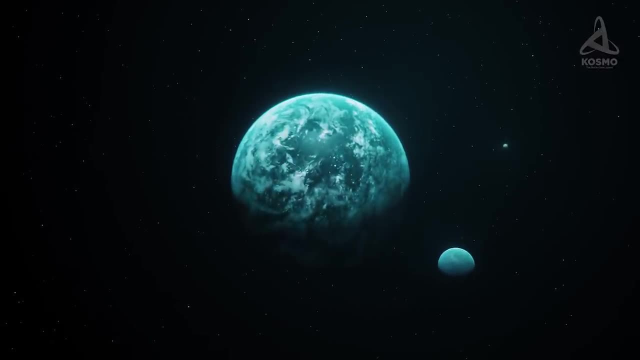 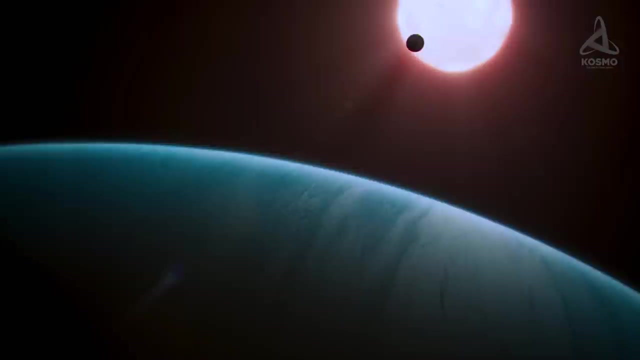 Based on the Earth Similarity Index, all the objects known to us conventionally fall into three categories. The first one is objects whose ESI is under 0.5. These are, for the most part, gas and dice giants, as well as extremely hot or, on the contrary. 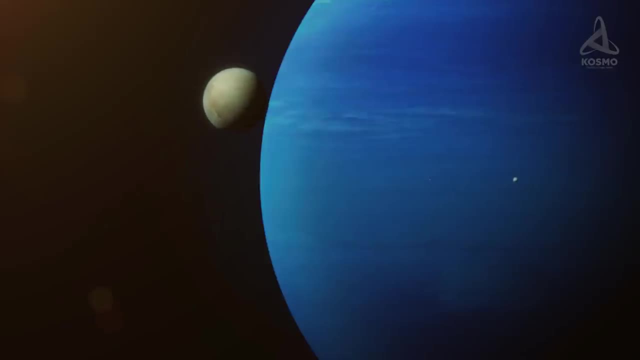 cold objects. This is the category most of the solar system planets and satellites fall into. It takes just one characteristic to greatly exceed the maximum. This is the category most of the solar system planets and satellites fall into. It takes just one characteristic to greatly exceed the maximum. 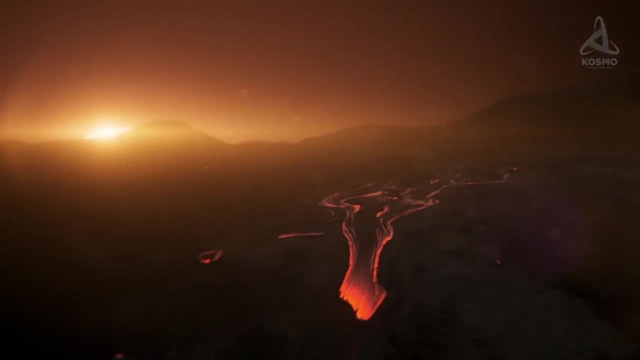 This is the category most of the solar system planets and satellites fall into, And it's for real that this is very withdrawal. It is to much for a celestial object to be unfavorable for the genesis and sustenance of life. Let's take Venus, for instance. 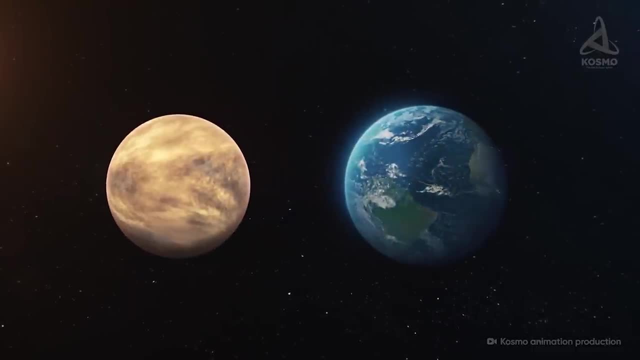 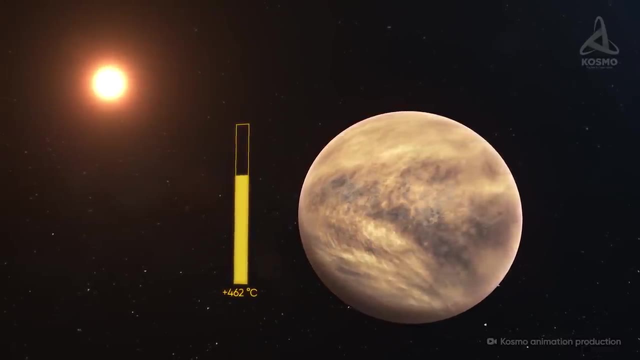 The radius and mass of this celestial body are very close to those of the Earth. However, due to its close proximity to the Sun and a dense atmosphere, its surface temperature is extremely high. That is why, in spite of a close similarity to Earth on the face of it, Venus's ESI is 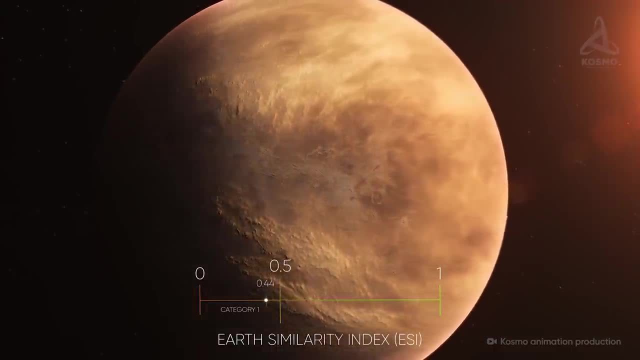 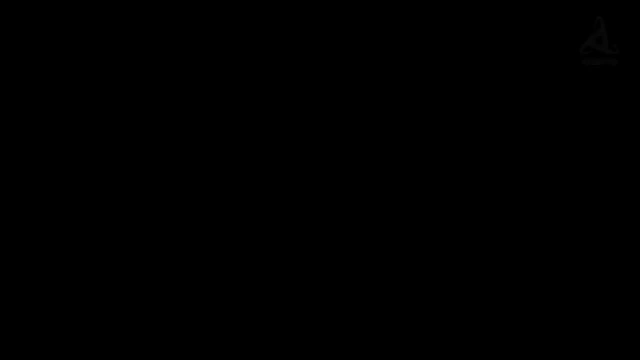 not high at just 0.44.. That is why, in spite of a close similarity to Earth on the face of it, Venus's ESI is not high at just 0.44.. We again complement $не". Of course. there being any life on its surface is totally out of the question. 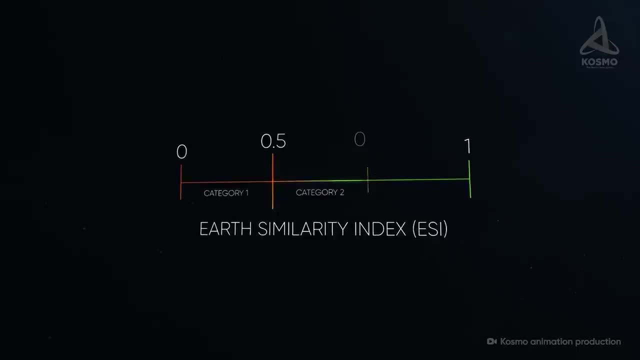 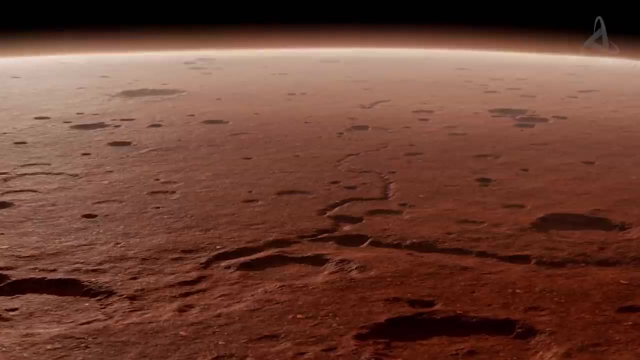 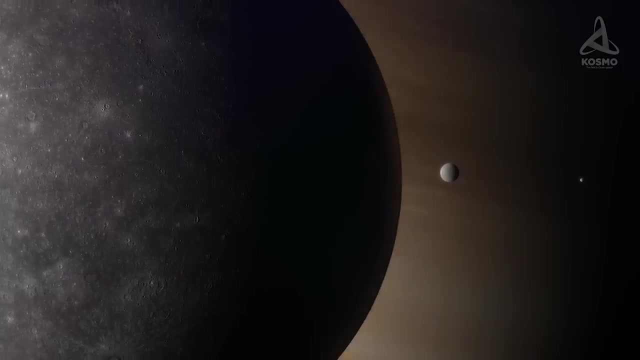 Celestial objects whose ESI is within 0.5 to 0.7 fall into the second category. These objects resemble our home planet noticeably more. They're mostly rocky worlds with relatively moderate temperatures, but it can also be ocean planets and even some large satellites. 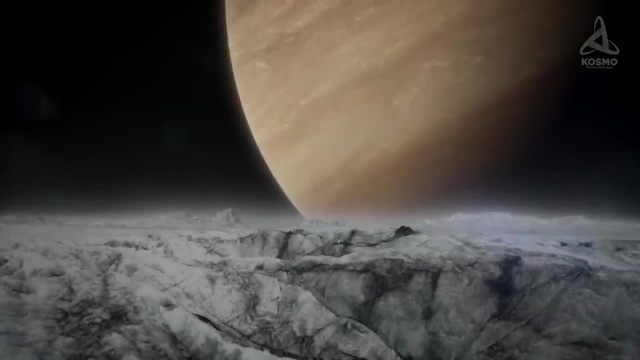 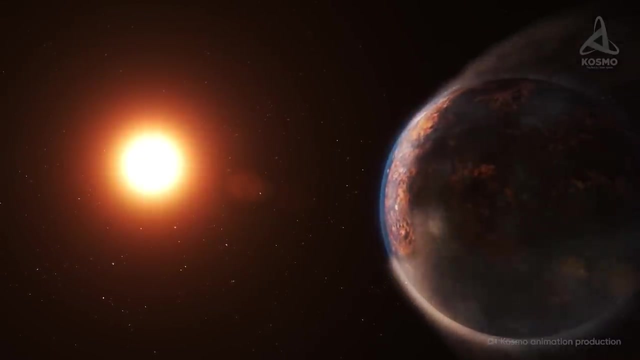 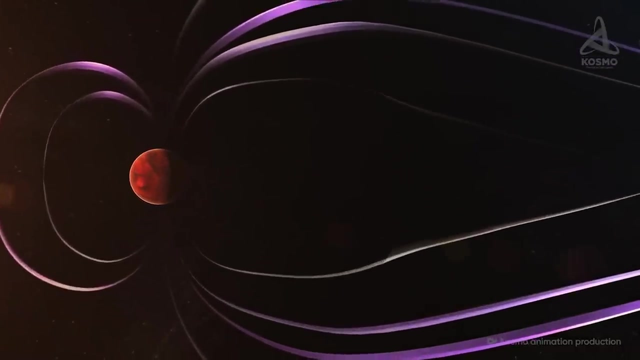 Incidentally, a high Earth similarity index per se does not warrant favourable conditions for life. For example, quite often low-mass planets are incapable of retaining a dense enough atmosphere, while their magnetic field is too weak to protect the surface from lethally dangerous radiation. 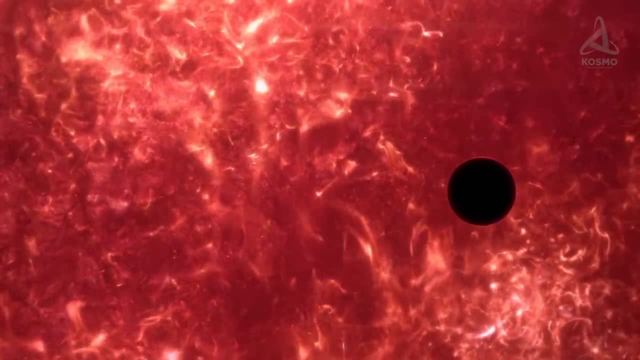 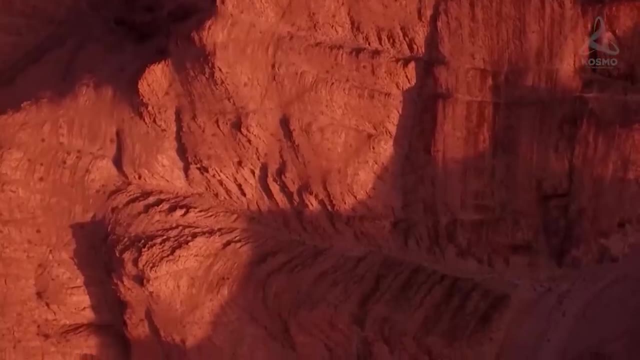 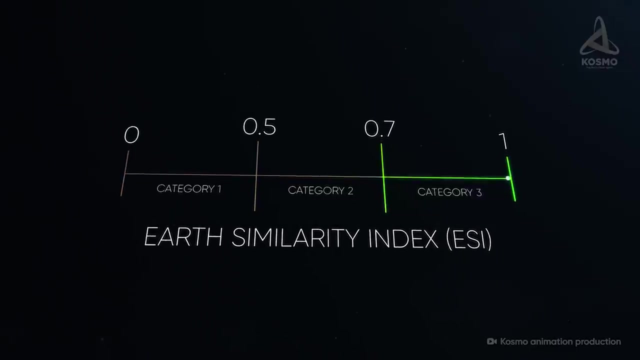 Other celestial bodies yet may happen to be located too close to their parent star and so get tidally locked. Of course, all these factors greatly reduce the chances of life's change. As for the third category, it contains celestial bodies with a high ESI that is over 0.7.. 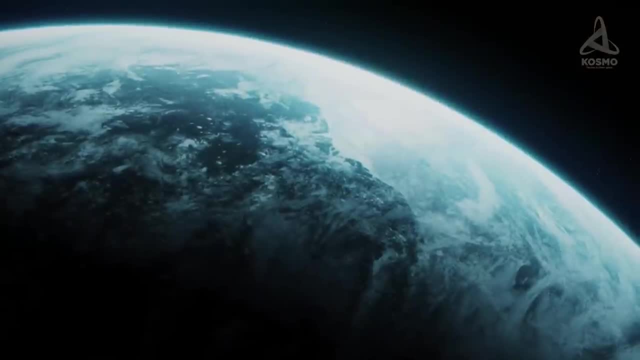 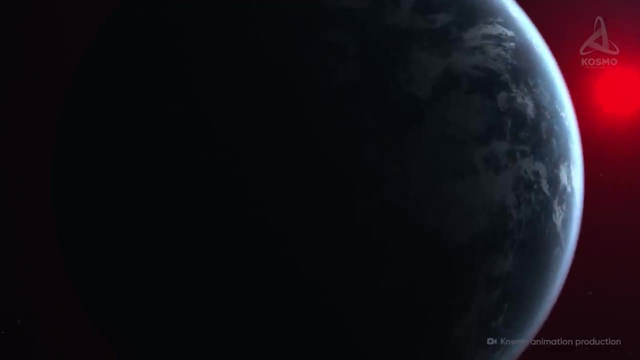 All of these planets are beyond the Solar System. According to estimates, the size of these worlds and the conditions on their surfaces are potentially close to those of the Earth. Among these planets, there is one which resembles ours most, and it lies just 12.5 light-years. 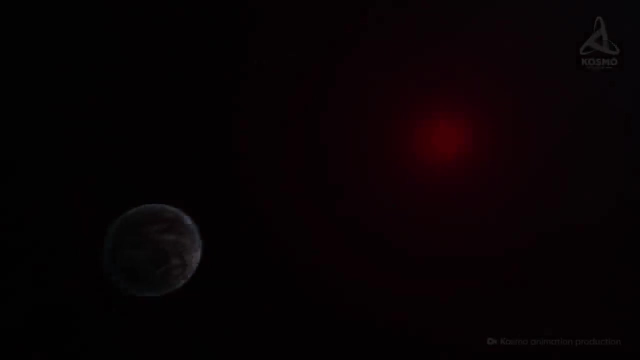 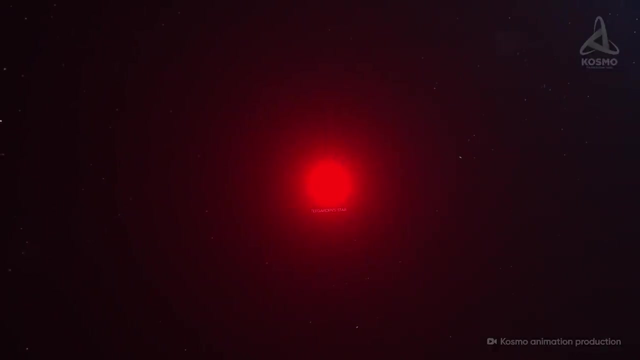 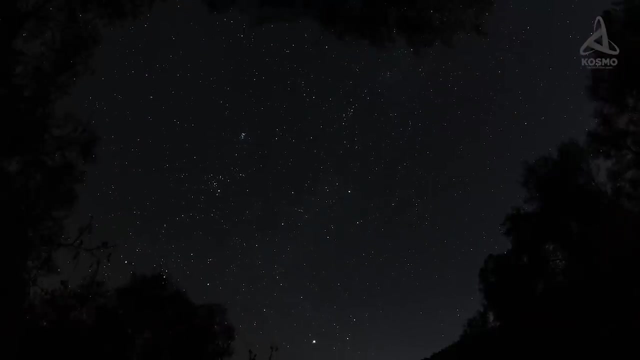 away from the Earth. This amazing world orbits Teegarden's star, a small red dwarf discovered in 2003.. This star is 1,370 times dimmer than the Sun. This means that it cannot be observed with the naked eye, even though it lies quite close. 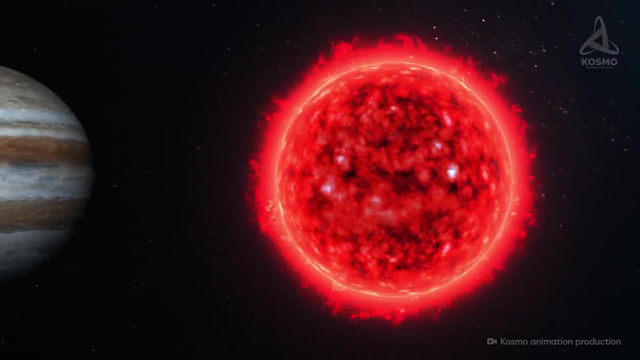 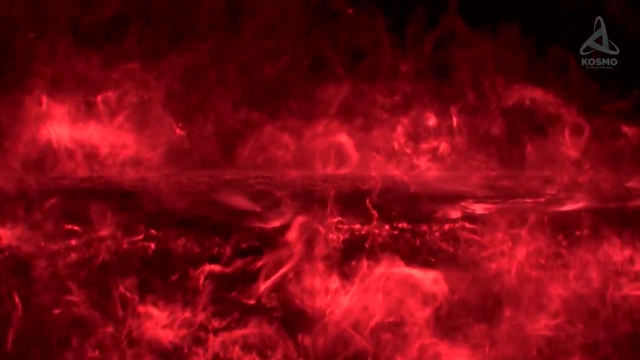 to the Earth. The mass of this tiny star is roughly 9% that of the Sun, and its radius is about 5% bigger than that of Jupiter. Gravitational forces are barely strong enough to maintain the thermo-mechanism. However, it is possible to observe it with the naked eye, even though it lies quite close. 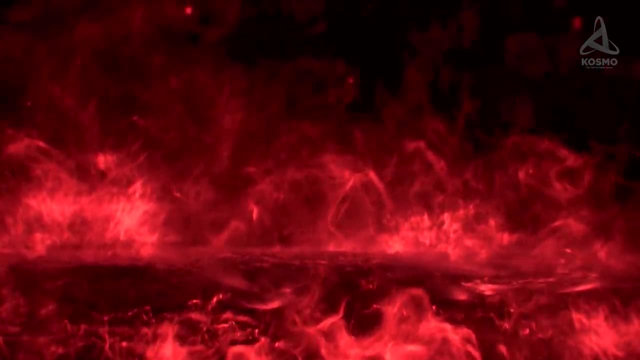 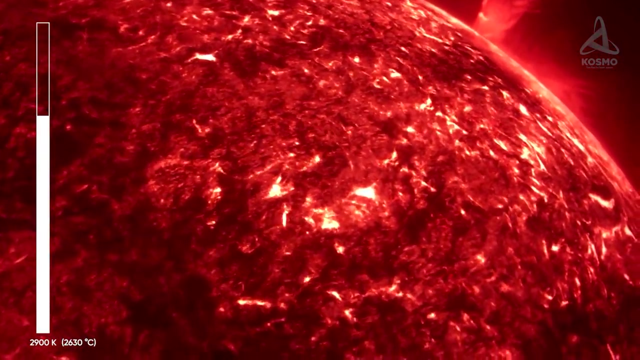 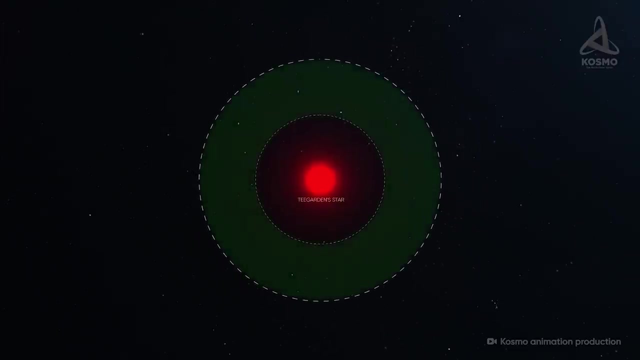 to the Earth. The red dwarf has a very strong nuclear reaction in the star's interior. That is why the surface temperature is just 2,900 Kelvin, or roughly 2,630 degrees Celsius. As is the case for all red dwarfs, Teegarden's star's habitable zone is comparatively narrow. 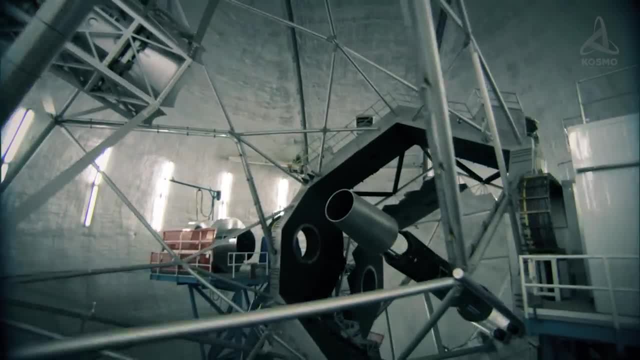 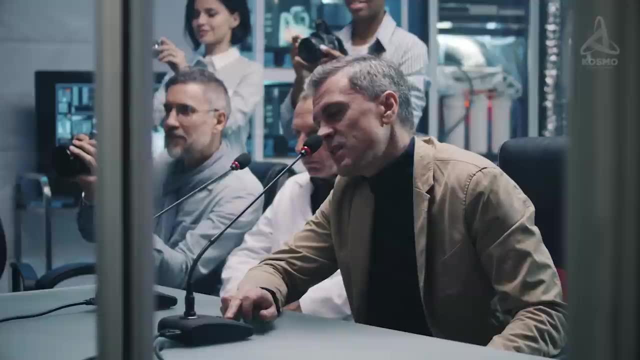 and located very close to it. Back in 2019, two exoplanets were detected in its system after continuous observations of the star's proper motion. Interestingly, one of them was called Teegarden's star. The other one was called Teegarden's star. 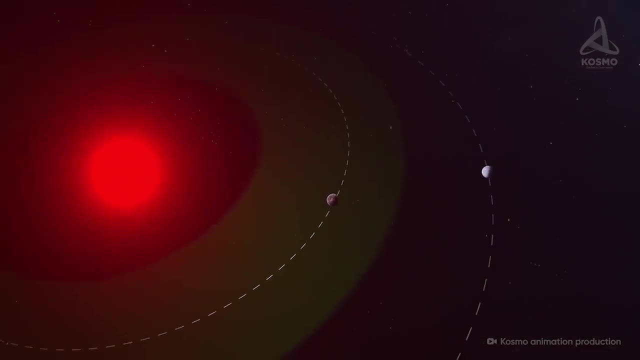 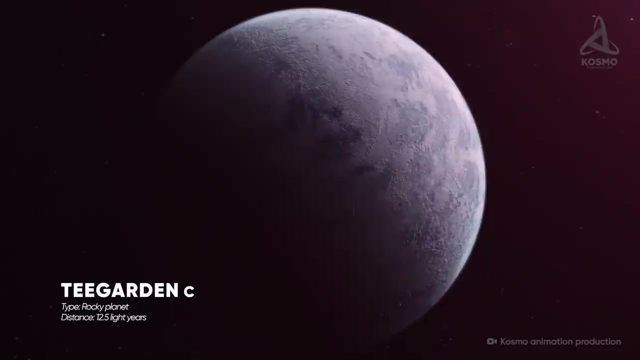 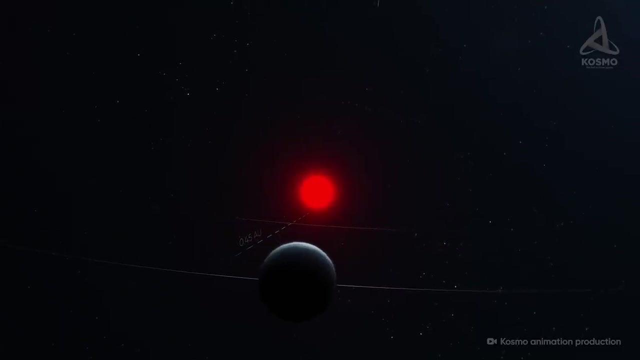 Interestingly, one of them lies beyond the star's habitable zone and the other within The outer planet. dubbed Teegarden C follows an almost ideal circular orbit around the system's centre. With the orbit's radius 0.045 AU, it is completed every 11.5 days. 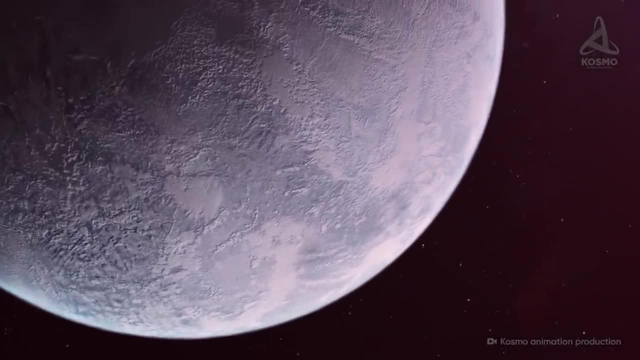 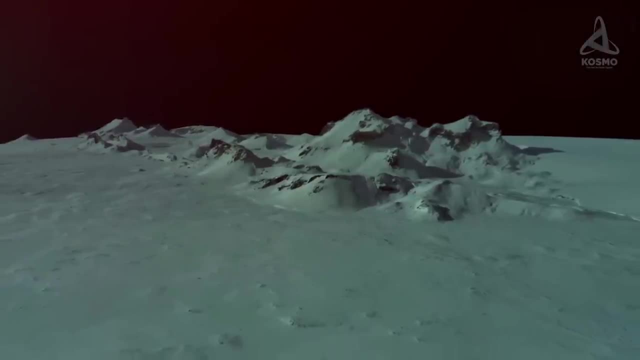 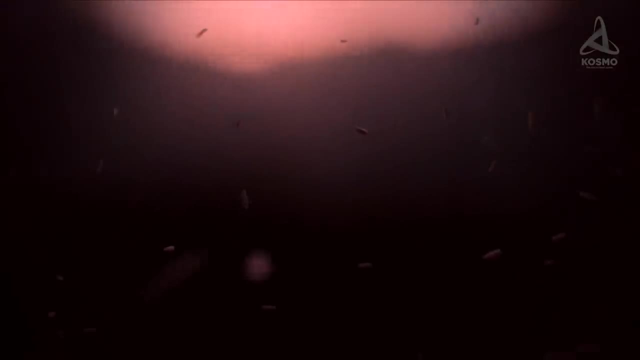 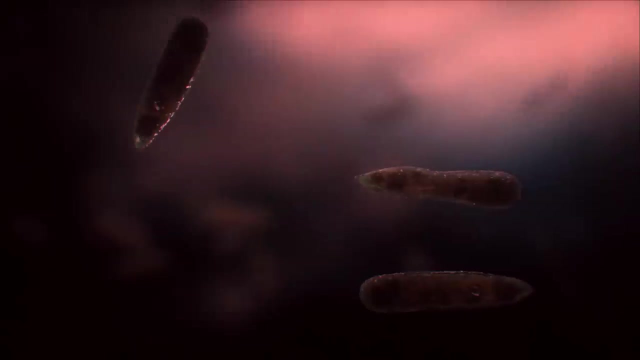 Due to the low luminosity of its parent star, the object enjoys 63% less energy than what the Earth receives from the Sun. As time goes by, primitive organisms might evolve in the warm depths saturated with energy and microelements. Just a tiny chance is sometimes enough for life to develop into something bigger. 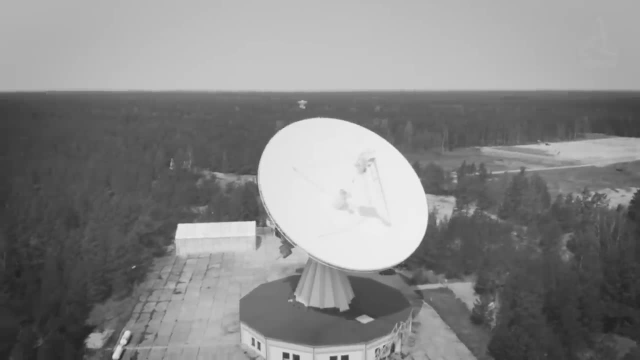 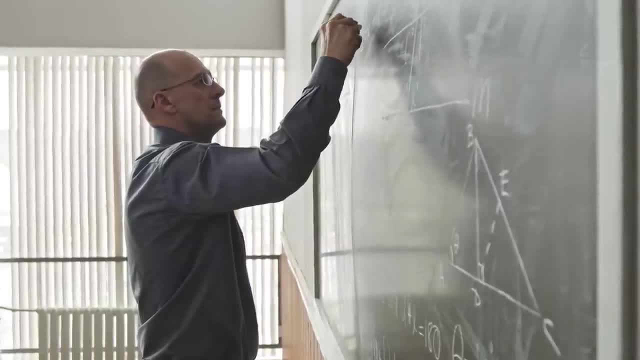 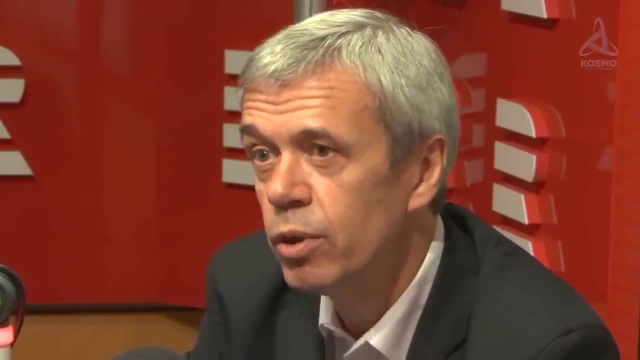 That is, planets fully covered in water, were made back in the 1970s. The theoretical calculations of these planets' formation and evolution processes were carried out in 2004 by French astrophysicists headed by Christophe Sartin. 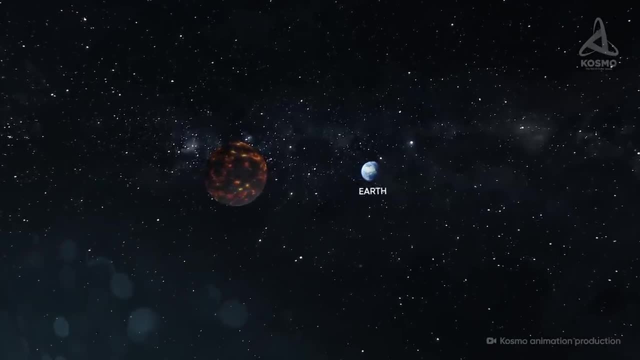 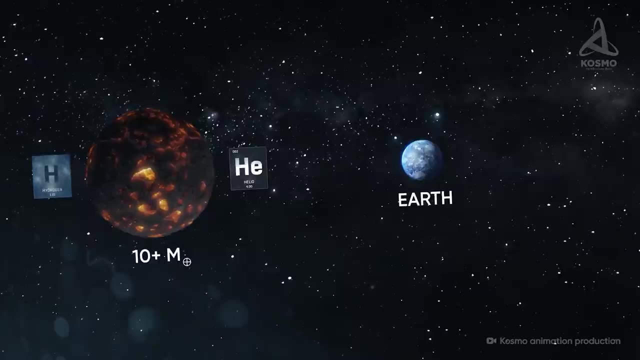 According to this theory, if the mass of a forming planet is more than 10 times that of the Earth, this starts to actively attract hydrogen and helium from the gas and dust cloud around it. In this manner, with time, it grows into a gas giant. 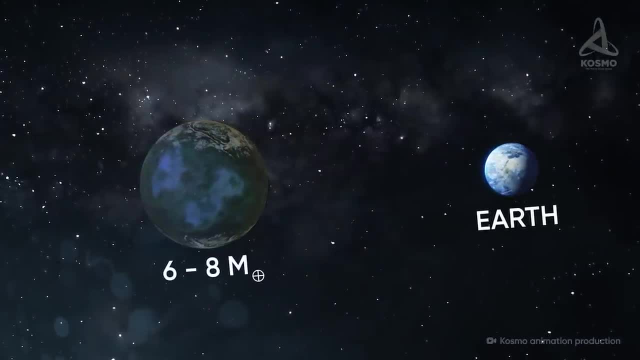 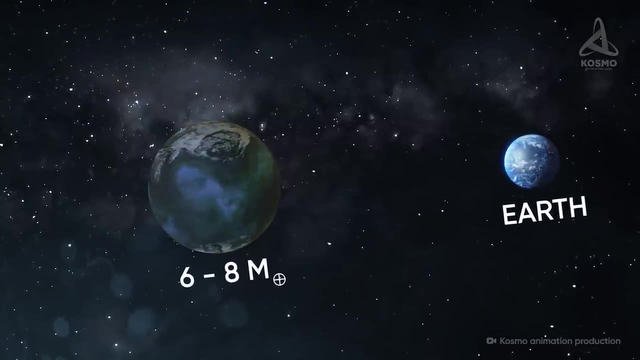 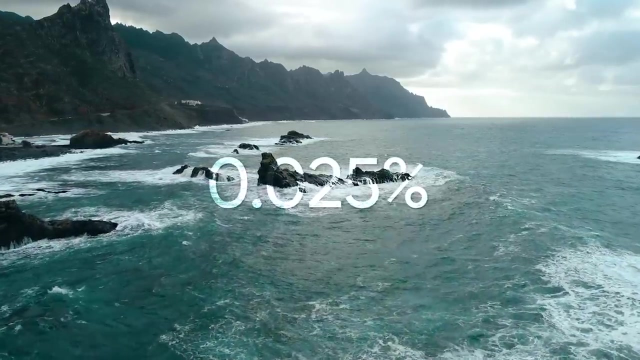 By contrast, if this planet's mass is just 6 to 8,, the new planet is going to be comprised of ice and rocks roughly in equal measure. Just to compare, the mass total of all water in the global ocean on our Earth accounts for just 0.025% of the Earth's total mass. 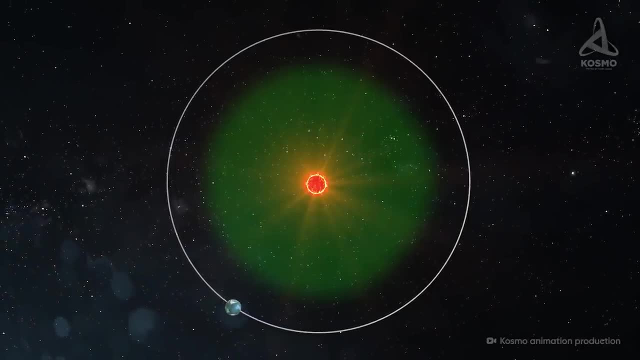 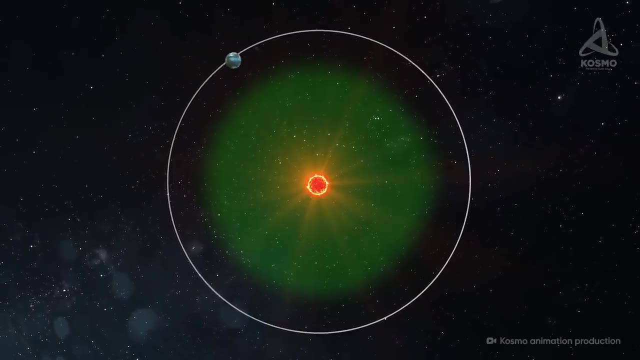 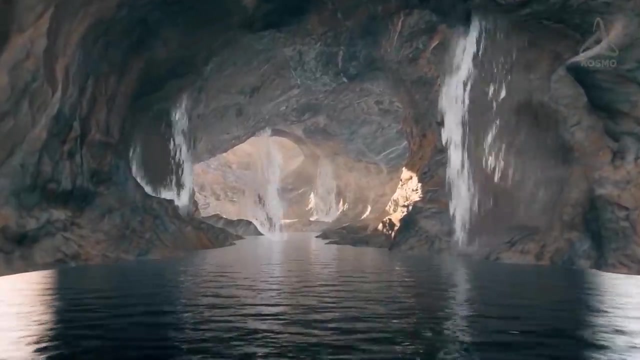 In this case, provided a space object's orbit lies far from the host star, this object is going to be either an ice giant or a cold super-Earth, radioactive decay taking place instantly. The ice inside the core will help melt some portion of the ice. 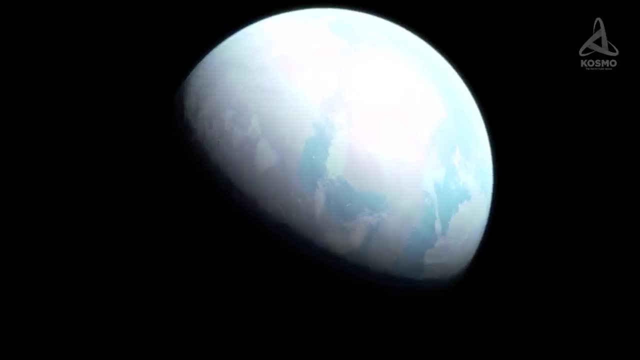 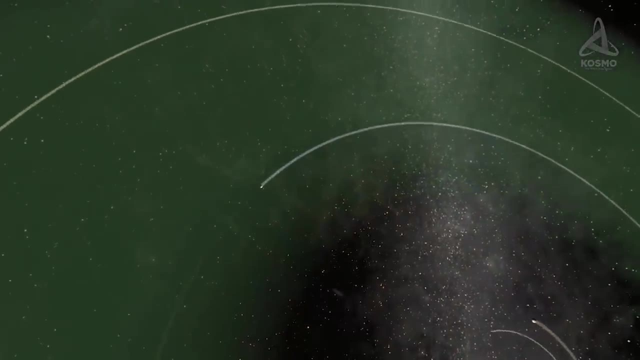 which in its turn will help form a subsurface ocean, but the planet's outer layers will still remain frozen. If the planet happens to find itself in its star's habitable zone, its outer layers will melt and spill all over the surface in a boundless ocean. Theoretical calculations show that a planet with a mass 6 to 8 times that of the Earth may have a layer of water over 100 kilometers thick. The temperature exerted by this amount of water may reach 20,000 atmospheres, depending on temperature, impurities and other parameters. 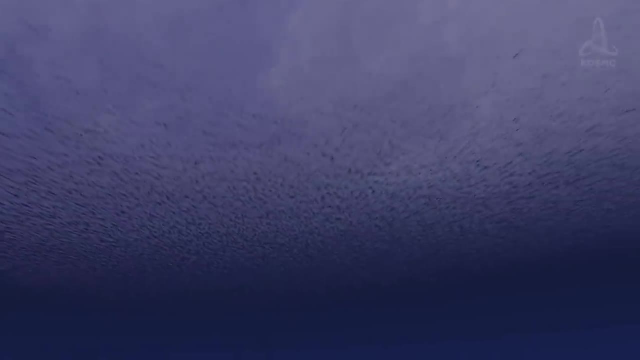 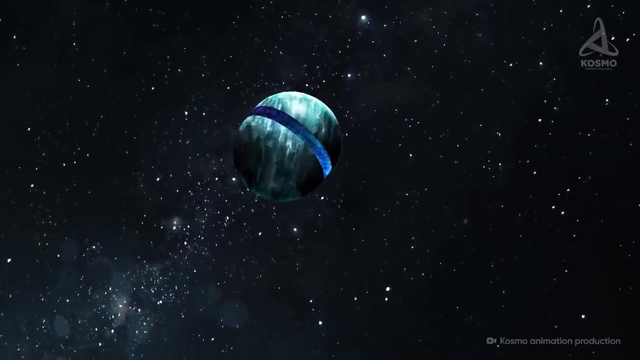 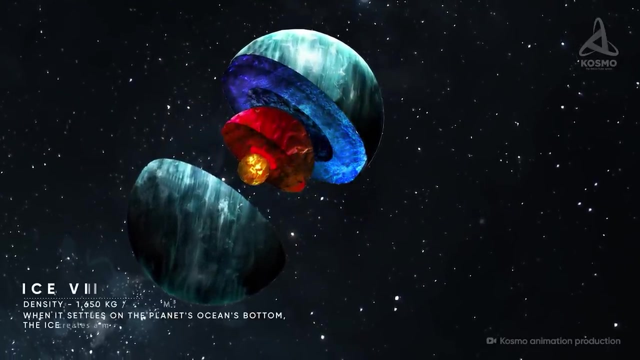 This is enough for some special exotic varieties of ice to form, like ones remaining solid even at high temperatures. In addition, unlike the familiar water ice, these modifications would be heavier than liquid water. For example, the density of ice 7,, which is likely to form in these conditions. 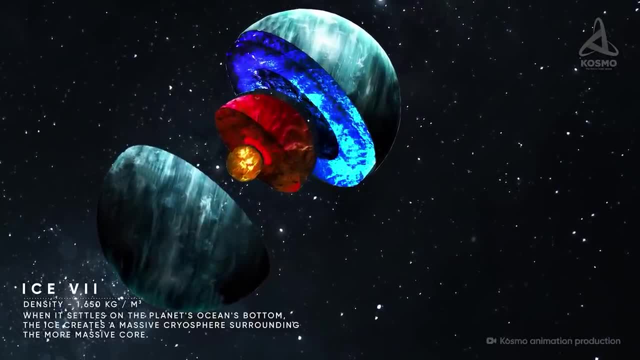 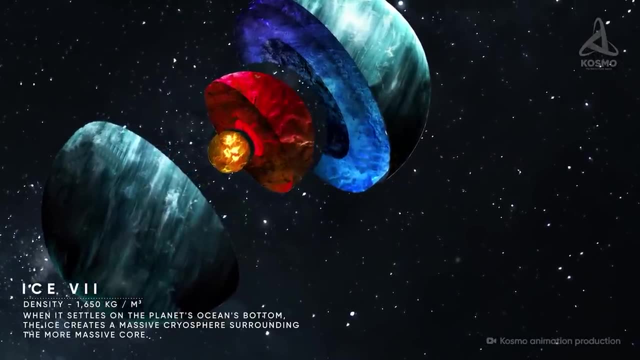 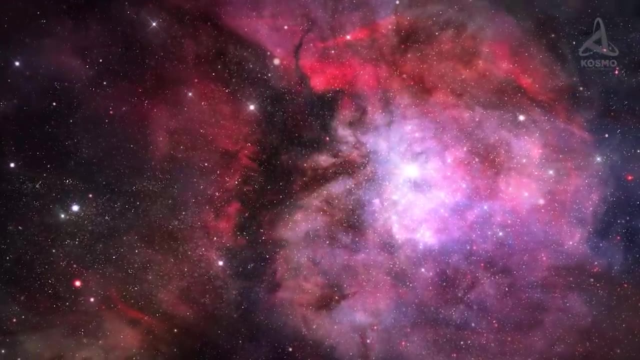 should be around 1,650 kilos per cubic meter. This ice settles on the planet's ocean's bottom and forms a massive cryosphere that envelops the more massive core. The opportunity to put these theoretical assumptions to test arose when a tiny and dim star was spotted 42 light-years away from the Earth. It was dubbed Gliese 1214.. The diameter of this red dwarf turned out to be five times smaller than that of the Sun, with its mass just 15.7% that of the Sun. At the same time, Gliese 1214 is 300 times dimmer than our parent star. 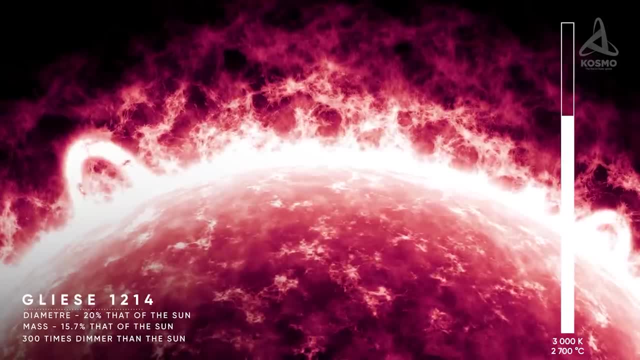 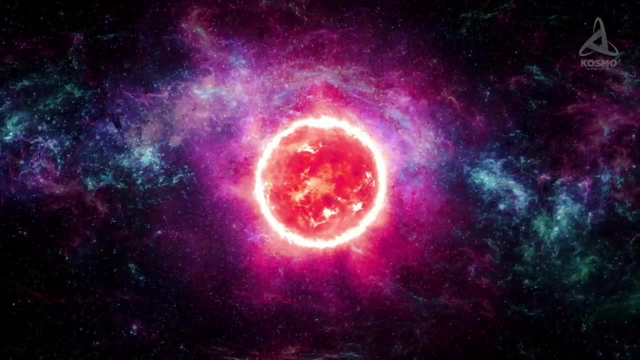 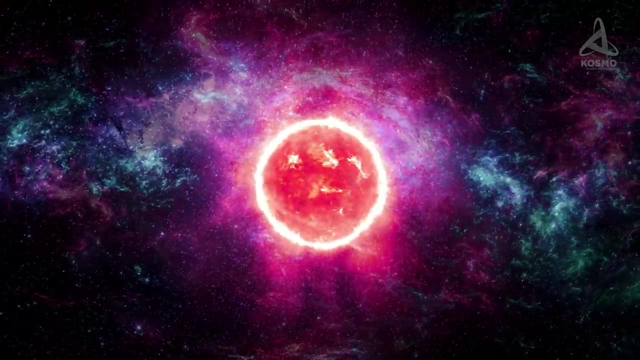 while its surface temperature is only 3,000 Kelvin or 2,700 degrees Celsius. There is nothing particularly remarkable about the star itself. To be blunt, it is just another nondescript red dwarf that looks like any of the billions of other stars in our galaxy. 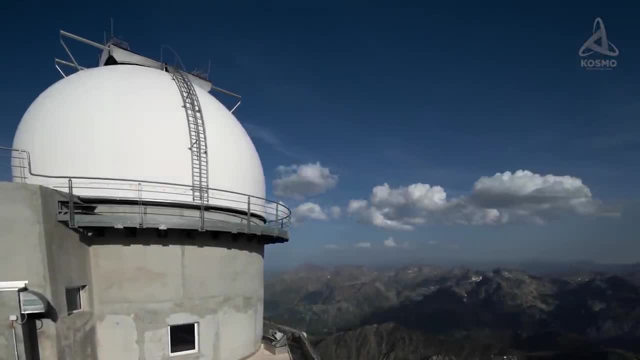 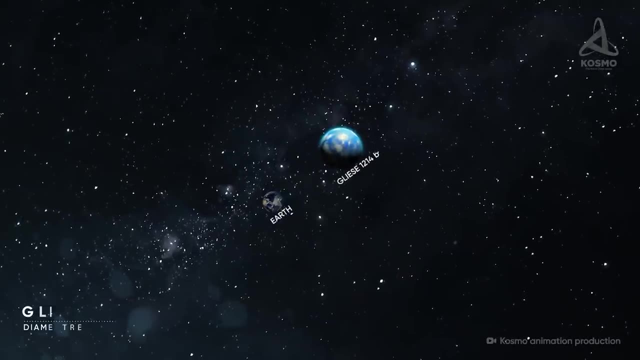 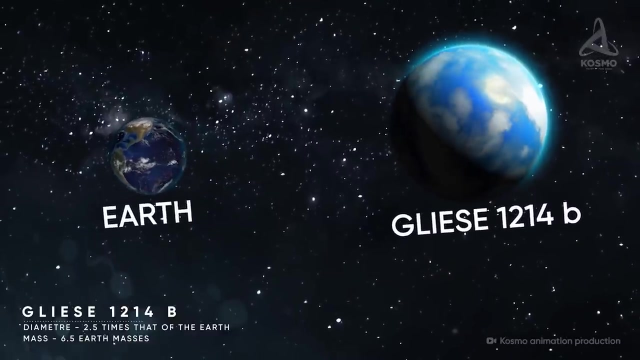 However, in 2009,, a solitary planet was detected in its environs, which was dubbed Gliese 1214 b. With its diameter measuring 2.5 times that of the Earth. this exoplanet is just 6.5 times heavier than our home planet. 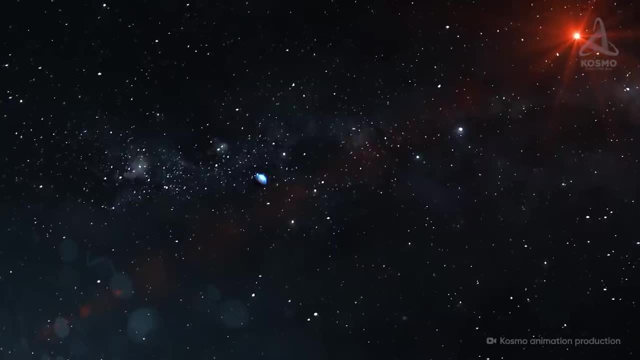 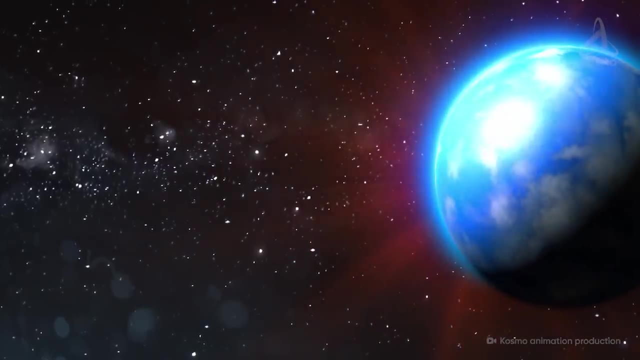 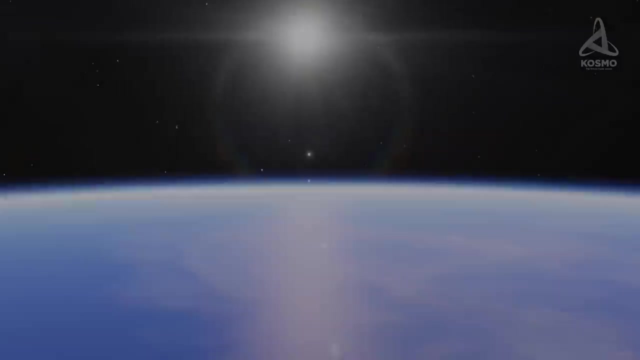 Straightforward calculations show the freefall acceleration on the exoplanet's surface to be just 91% that of the Earth. The average density of Gliese 1214 b is approximately 1,870 kilos per cubic meter. Judging by this comparatively small value, 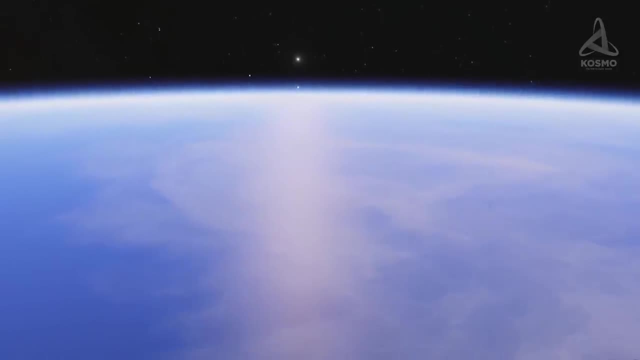 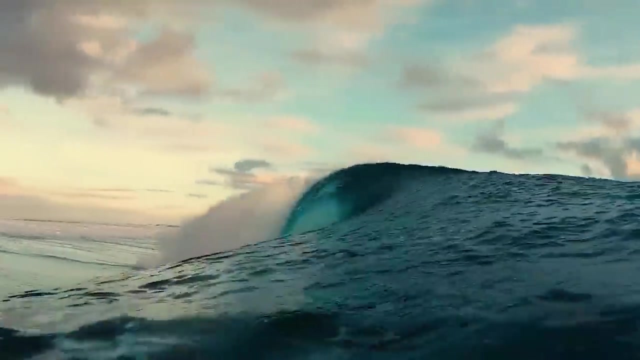 the exoplanet cannot realistically be made up of mostly metals and rocks, as is the case with our Earth, for example, But incidentally, this average density value seems to confirm the assumption that the astronomical body is 75% water or water-rice. 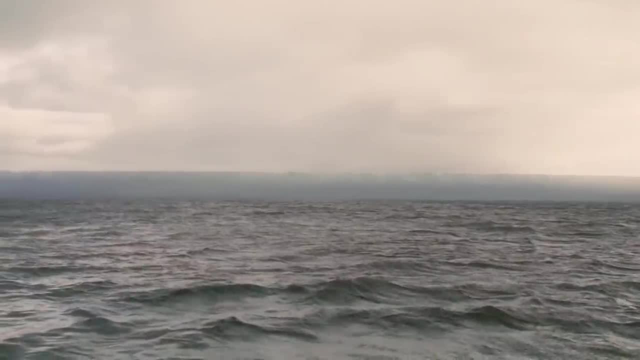 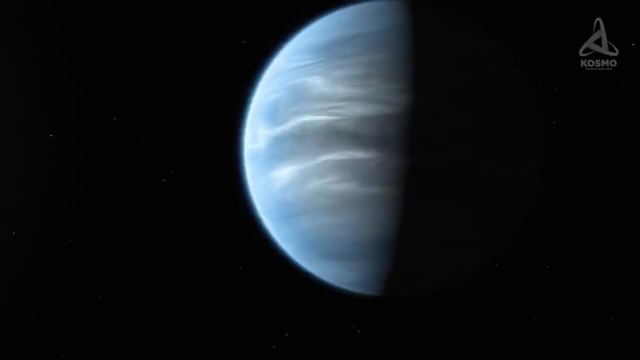 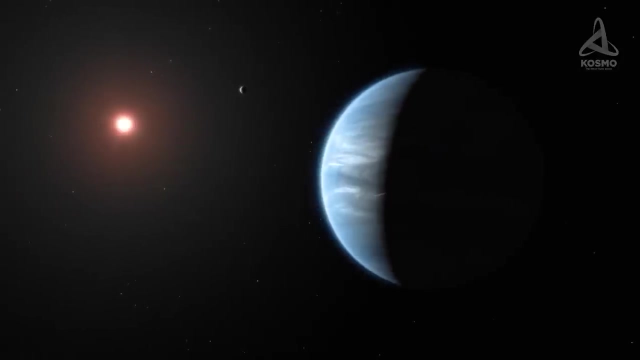 and just 25% water. Thus, it appears safe to suggest that this exoplanet is an ocean planet. The object lies very close to its host star. The average distance between them measures just around 2 million kilometers, or 0.014 astronomical units. 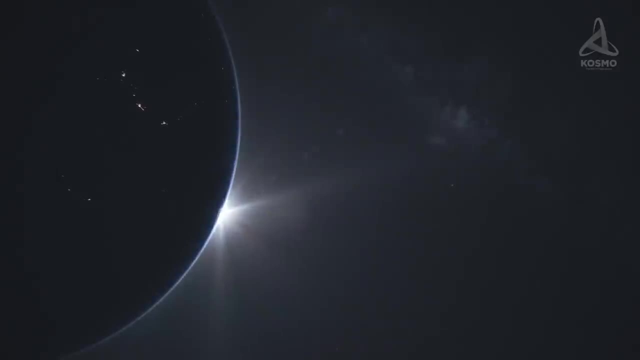 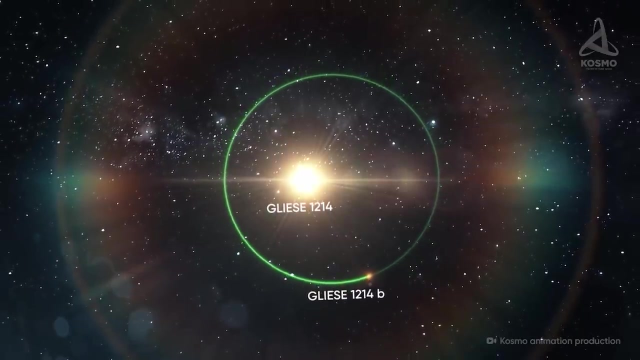 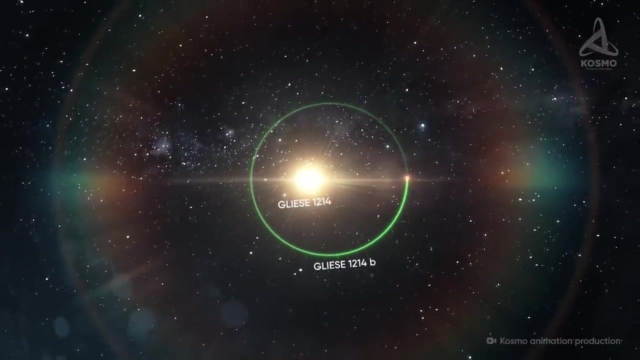 which is 75 times smaller than that between the Earth and the Sun. Also, the orbit eccentricity is rather high, at 0.27, slightly more than that of Pluto. This means that in its perihelion, Gliese 1214 b is approximately twice as close to its star. than when in its aphelion. As for its orbital period, it takes the planet about 36 hours to complete it. The red dwarf Gliese 1214 may be 300 times dimmer than the Sun, but this incredible proximity to the star makes the climate on Gliese 1214 b scorching hot. 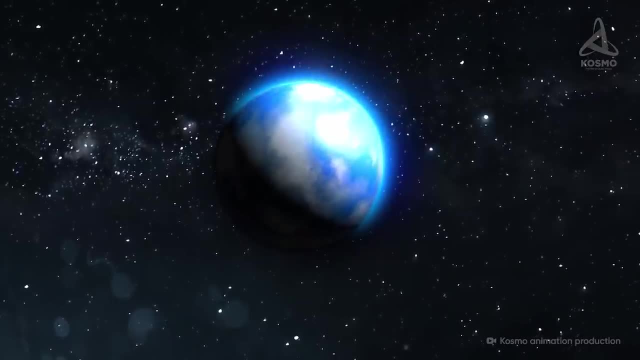 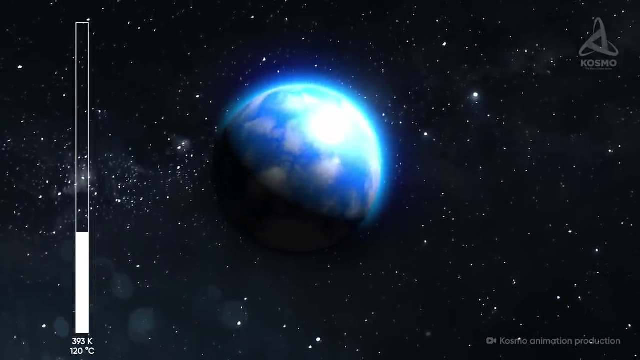 Supposing the reflection coefficient of the surface of Gliese 1214 b is the same as that of Venus, the planet's surface temperature is supposed to be around 393 Kelvin or 120 degrees Celsius. If, on the other hand, the surface is darker, 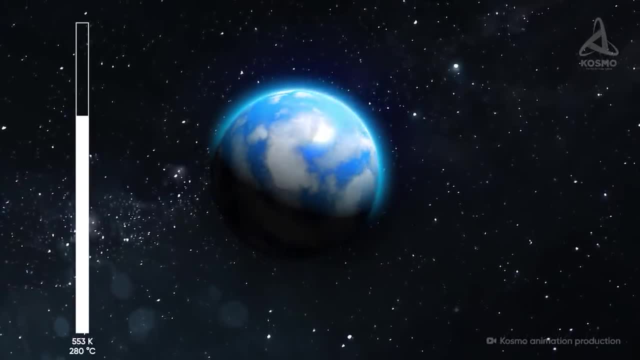 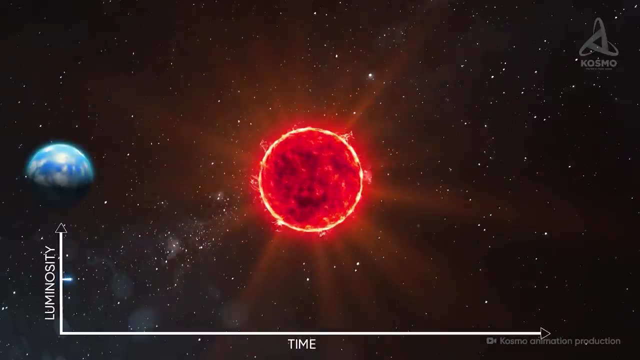 the temperature may reach as much as 553 Kelvin or 280 degrees Celsius. Due to the fact that the orbit of Gliese 1214 b crosses the star's disk, scientists are able to carry out spectroscopic investigations of its atmosphere. Still, the results are rather ambiguous. 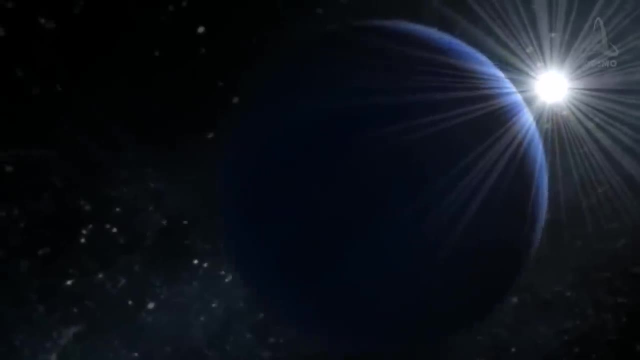 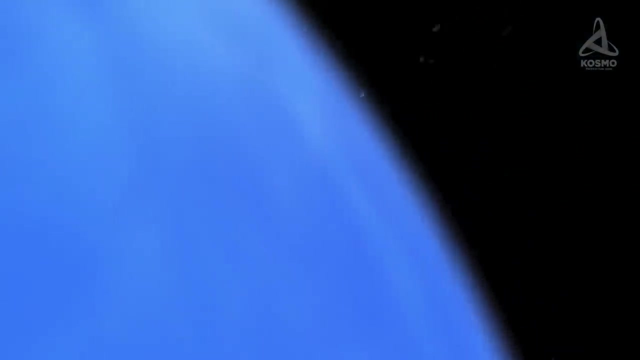 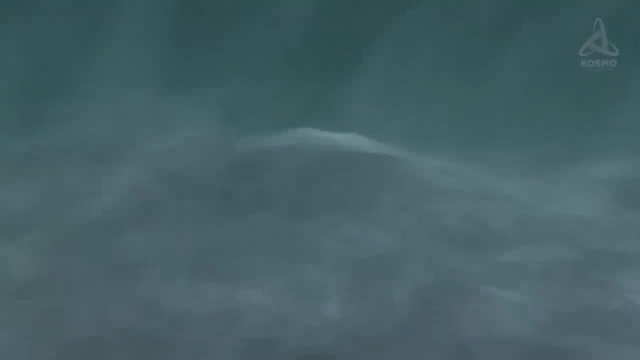 If this space object really is an ocean planet, its atmosphere is supposed to predominantly consist of water vapor with some accompanying gases. Interestingly, no lines of hydrogen, helium or complex substances like water, CO2, and ammonia have so far been detected in the planet's spectrum. 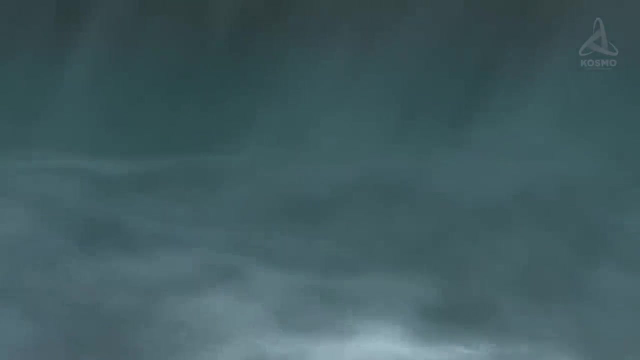 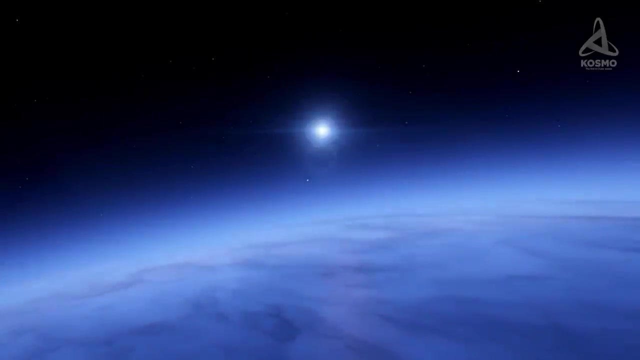 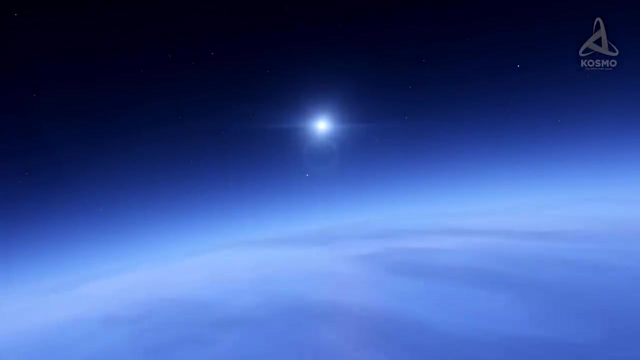 It is thought that the outer layer of the dense atmosphere conceals its true content from the observer. The conditions on the surface of Gliese 1214 b remind one of what it is like inside a giant steam boiler. Interestingly, the atmospheric pressure in its lower strata should be at least 15 times as high as that of the Earth. 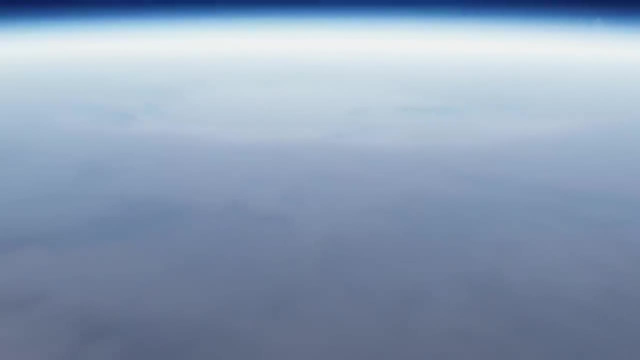 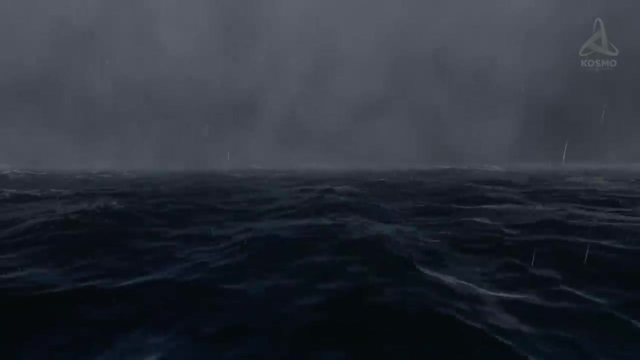 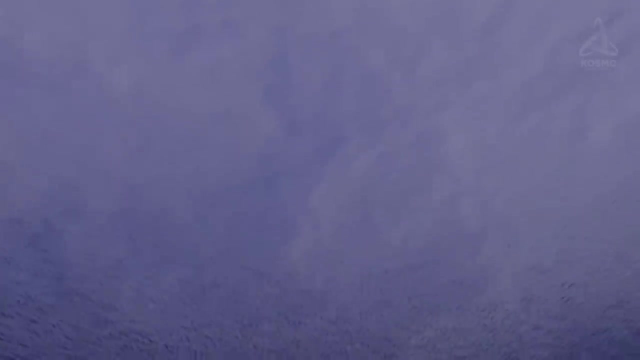 As the ocean and the atmosphere are in a state of thermodynamic equilibrium, the border between them is rather blurred. No wonder, as the density of water vapor just above the ocean's surface is practically equal to that of constantly boiling water As we look deeper at the lower strata of the ocean. 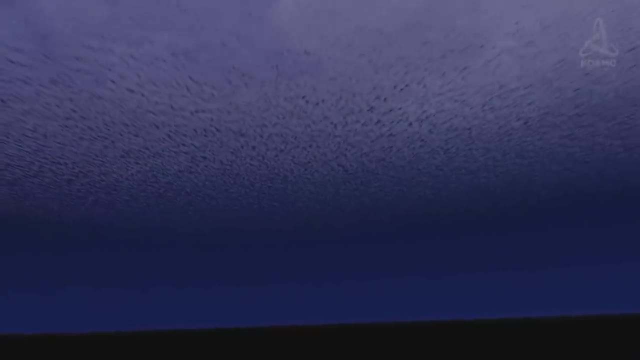 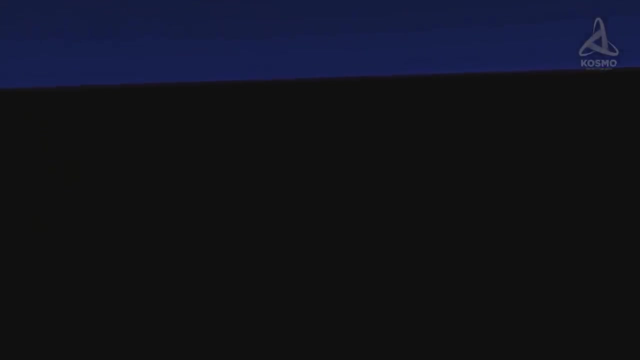 the pressure will continue to increase until we reach the depth of 100 kilometers. With a pressure value at this depth, water will be unable to remain in its liquid state even at temperatures this high, and so we will see the bottom made up of dense and heavy ice. 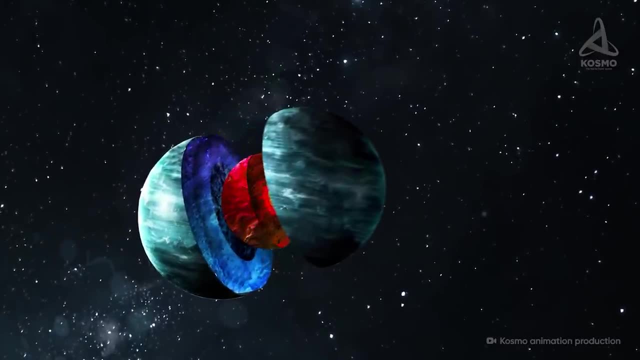 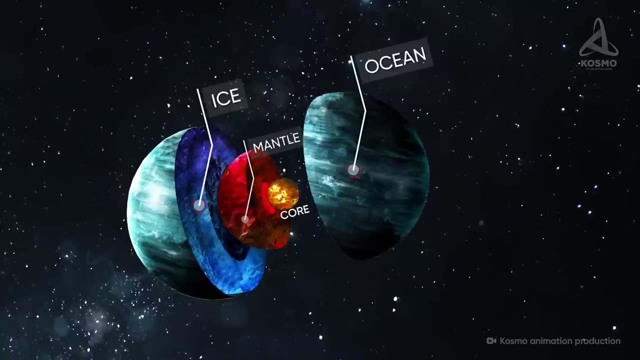 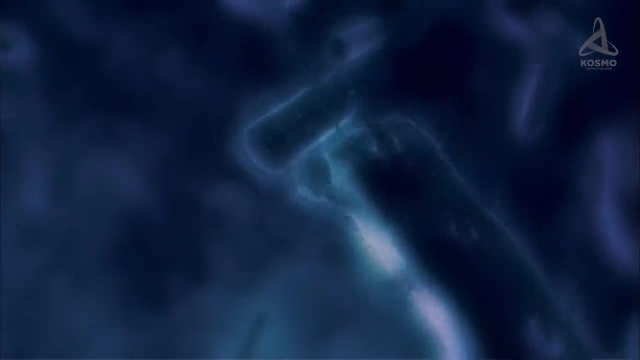 whose thickness is estimated to be upwards of 5,000 kilometers. Thus, most water on the planet is concentrated here. Below the cryosphere, there should be the core, made up of rocks and metals. Unfortunately, chances of life evolving on any ocean planet are rather thin. 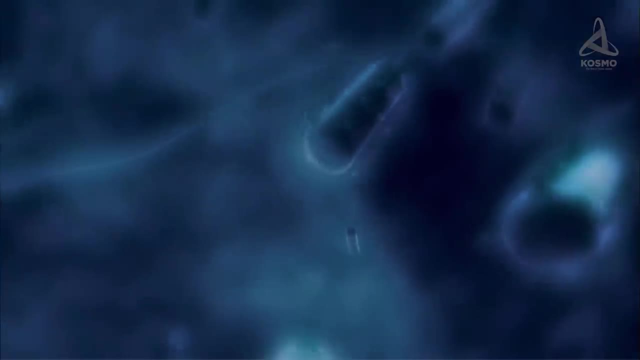 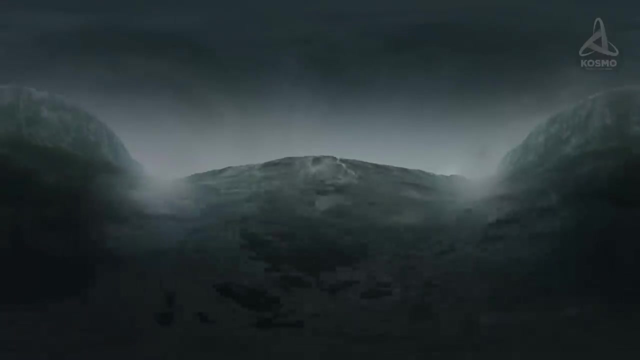 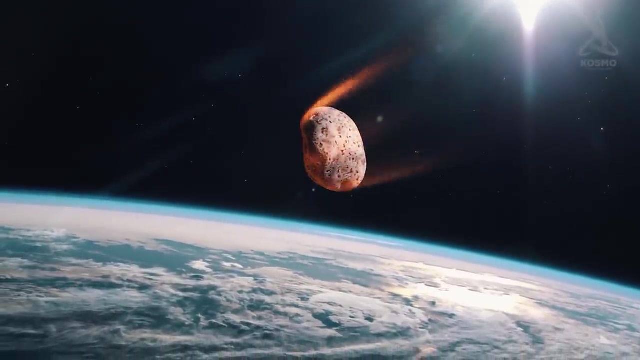 even if the surface temperature happens to be more favorable than on this one. This is so due to the fact that oceans on planets like that are too poor in terms of microelements that are vital for living creatures, Even taking into account meteorites that occasionally bombard the surfaces of these celestial bodies. 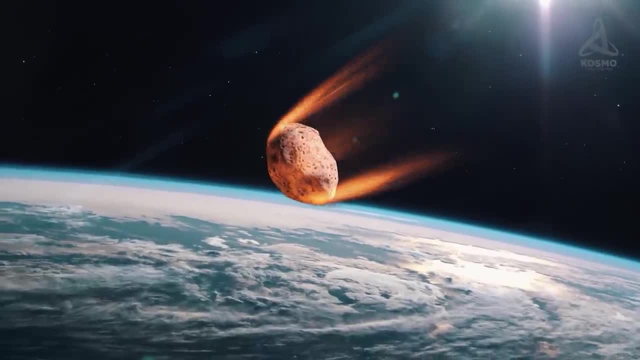 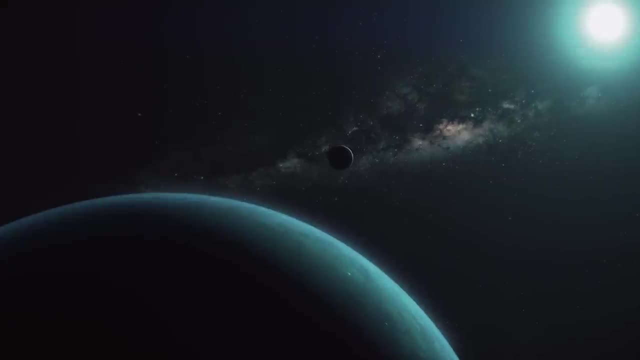 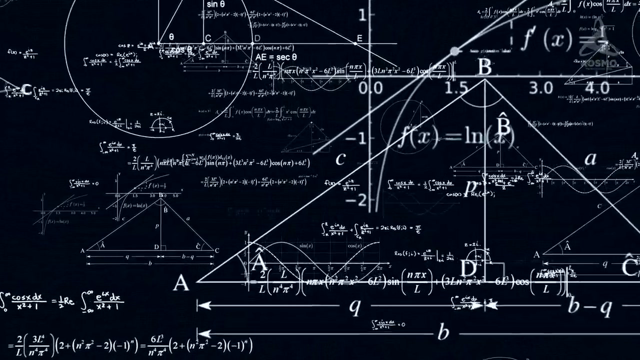 the chemical diversity is simply not good enough for life to originate here. Still, studying ocean planets poses a great scientific interest. According to NASA's mathematical modeling estimates published in 2020, there may be billions of planets of this type in our galaxy. 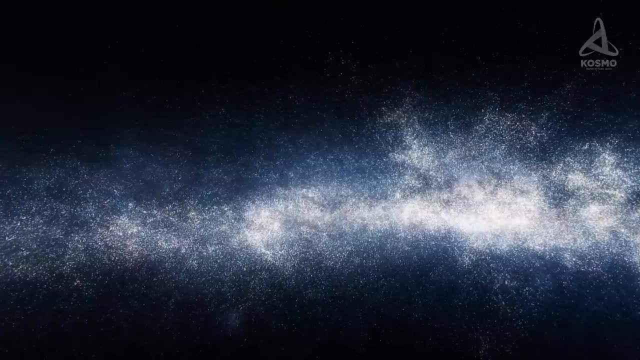 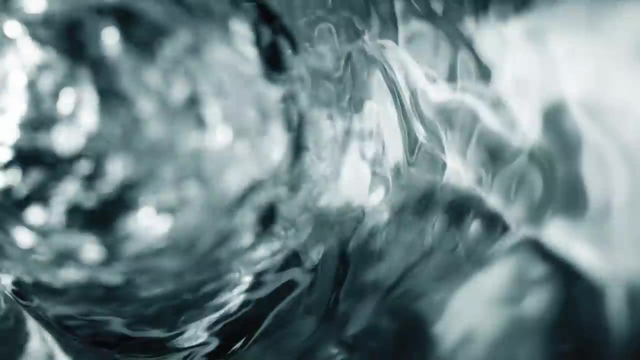 both cold, harboring an ocean under an ice shell, and warm, like Gliese 1214 b. Water is one of the most widespread complex chemical compounds in the Universe, and this means that the chances of discovering new ocean planets are quite optimistic. 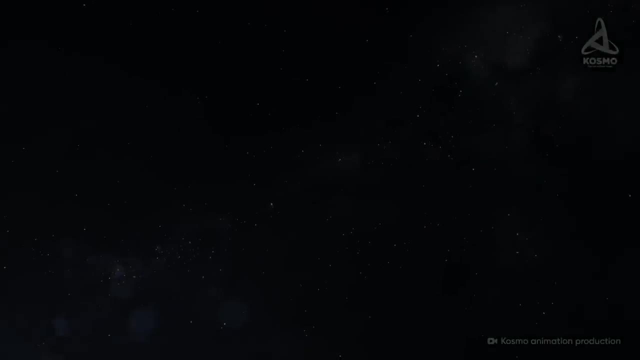 What is the existence of space objects the size of a planet? Assumptions about the existence of space objects the size of a planet which are independent from any star have been around for a long time, Such celestial objects freely drifting around interstellar space. 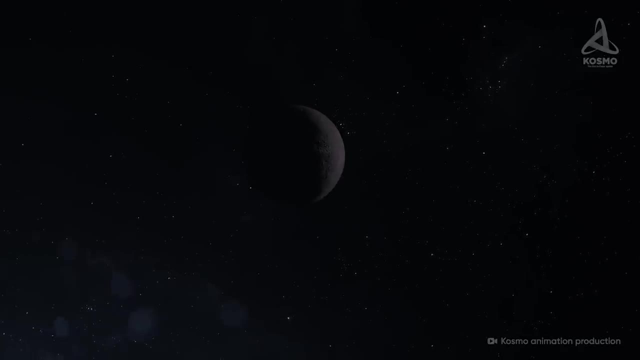 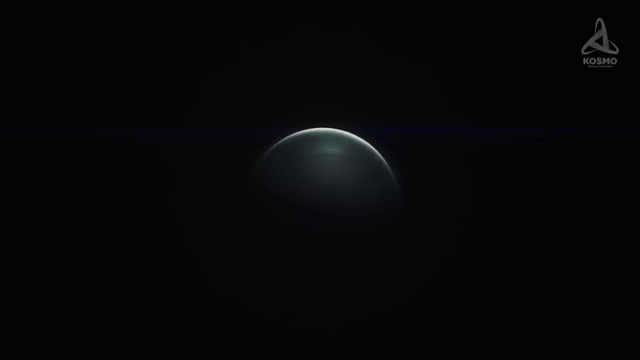 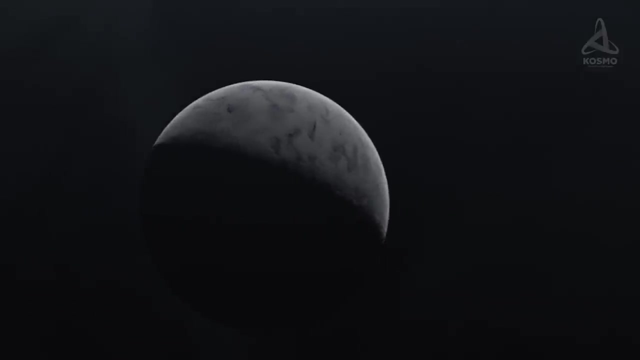 are referred to as orphan, free-floating or rogue planets. Astronomical bodies of this kind emit very little thermal and light energy into space around them. It is suggested that there are no bodies in their close proximity they could clearly interact with or be bound to. 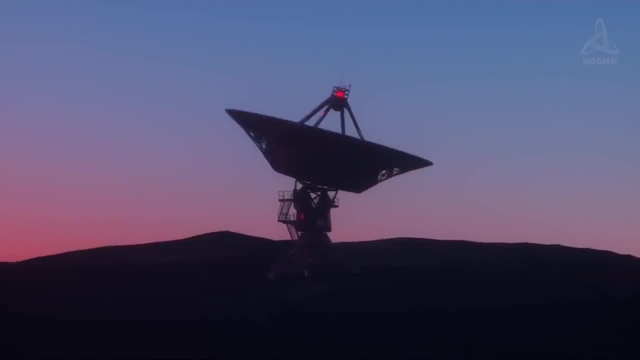 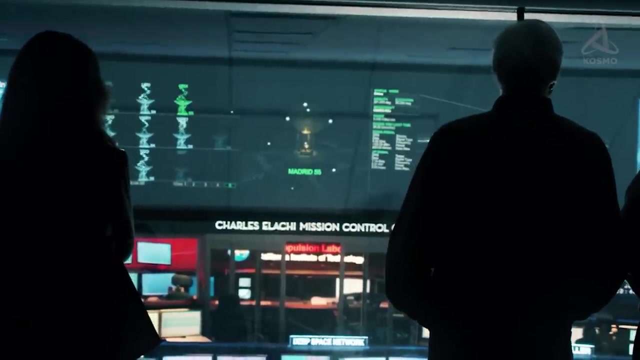 That is why it is hardly surprising that these objects are so difficult to detect. The first potential representatives of this class of planets were spotted as recently as in the early 21st century. The warmest rogue planets can be detected with infrared telescopes. 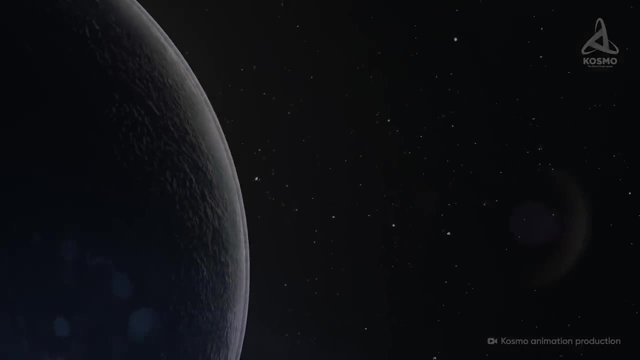 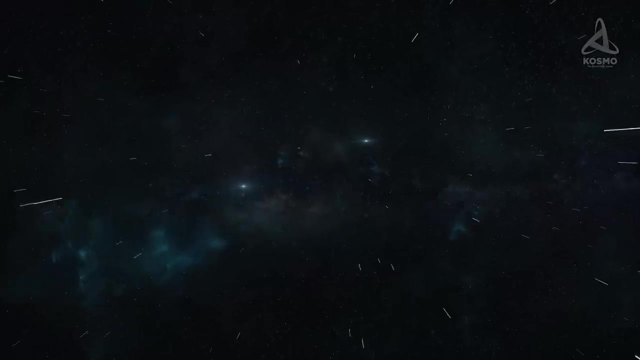 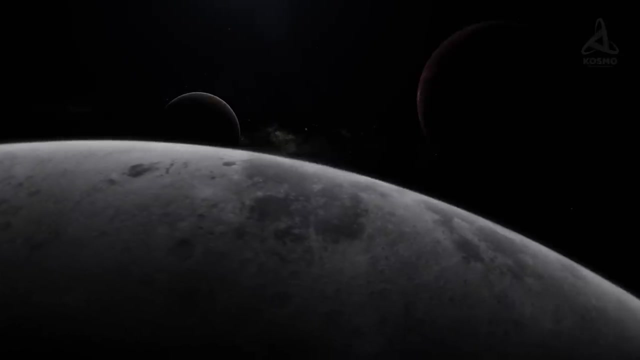 and others, thanks to something called the gravitational microlensing effect. As one would expect, this class of celestial objects is one of the most mysterious and understudied. Today, only three astronomical bodies can be classified as rogue planets with a sufficient degree of certainty. 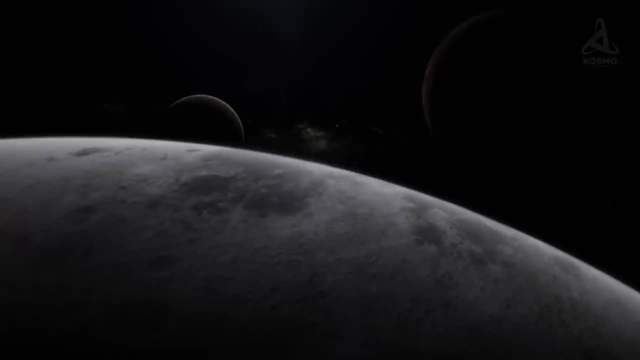 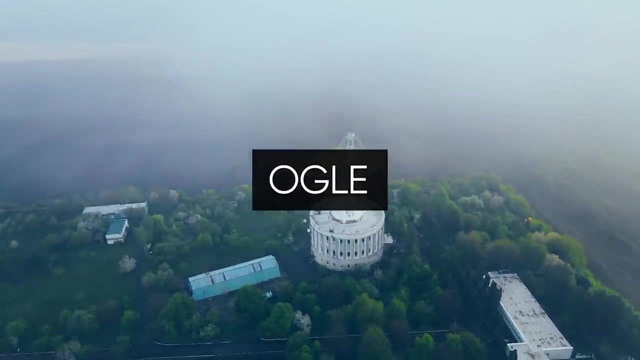 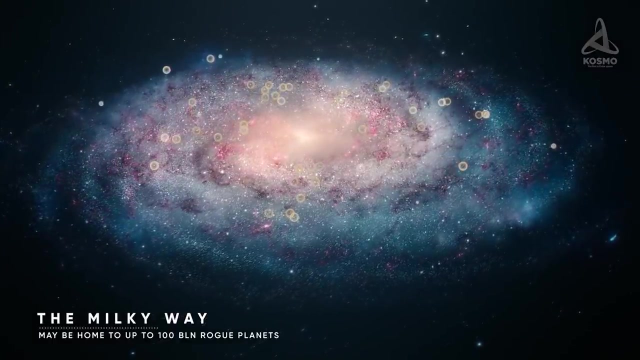 with the overall number of rogue planet candidates over two dozen. Incidentally, according to the analysis of data collected in the course of the OGLE project, the Milky Way may supposedly be home to up to a hundred billion objects of this class. This may only mean that right now, 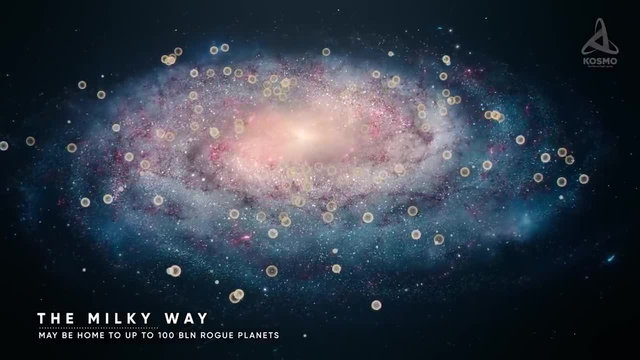 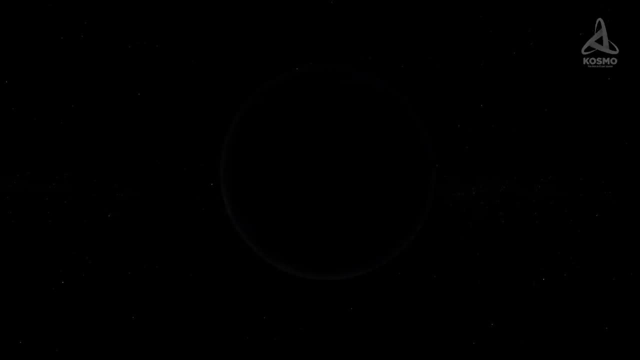 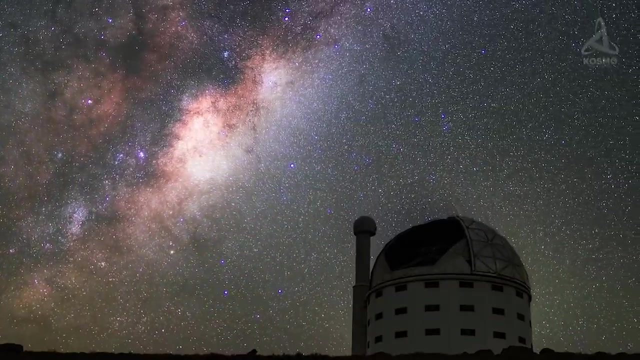 we are at the very beginning of an upcoming series of discoveries in this field. Our notions of what rogue planets are like have long been based purely on assumptions and hypotheses. With the technological advancement of highly sensitive observation equipment, there arose opportunities to put them to the test in practice. The rogue planet lying closest to the Earth among those already confirmed is known as WISE 0855-0714.. 7.27 light years away from the Sun, it was detected in 2014 with the WISE Orbital Infrared Telescope. 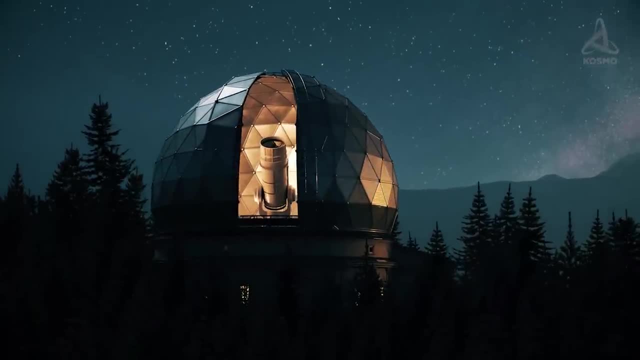 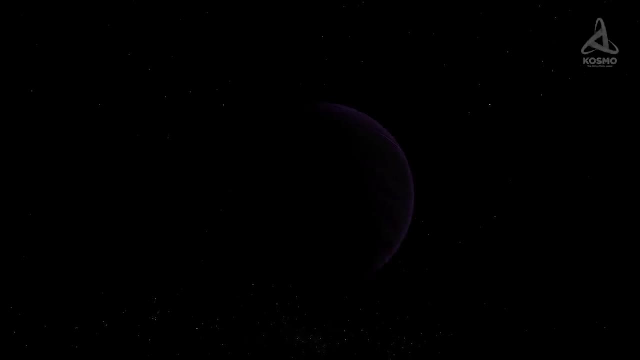 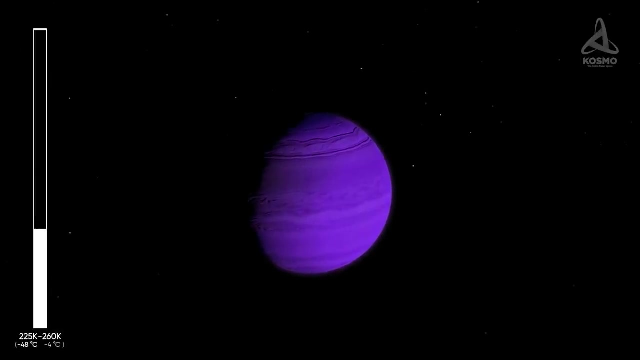 The astronomical body cannot be seen through optical telescopes as it emits no visible light to speak of. The reason for this is its extremely low temperature, From 225 to 260 Kelvin, or 48 to 13 degrees Celsius below zero In terms of its parameters. 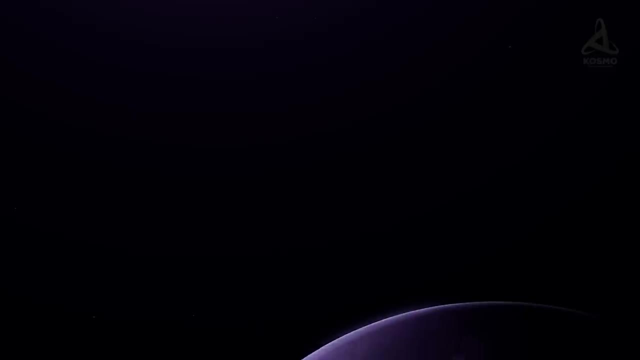 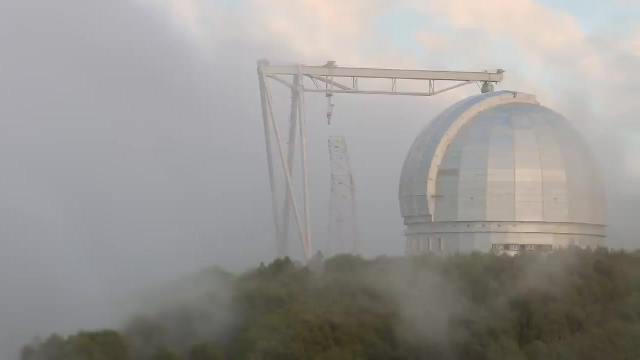 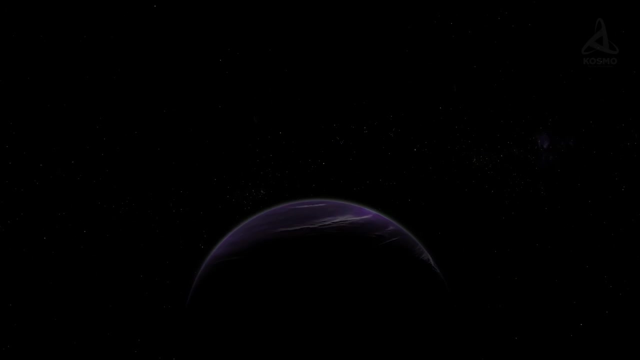 it resembles a cooled-off gas giant and its age cannot be under a billion years. The rogue planet is mostly made up of hydrogen, However. in 2016,, the Gemini Observatory produced evidence of the presence of large amounts of water in its atmosphere. 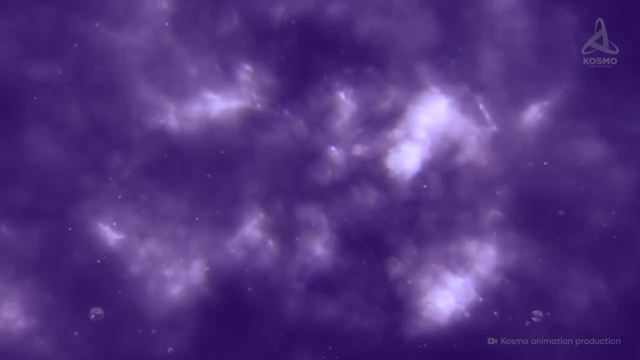 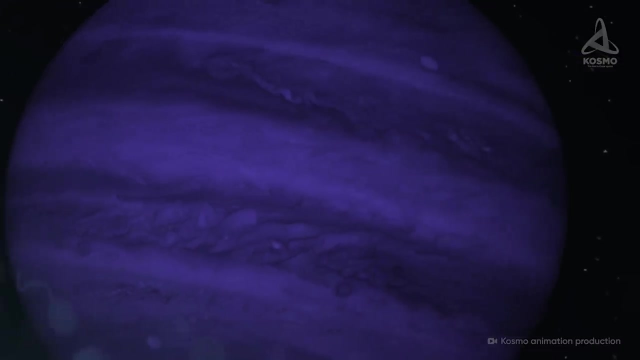 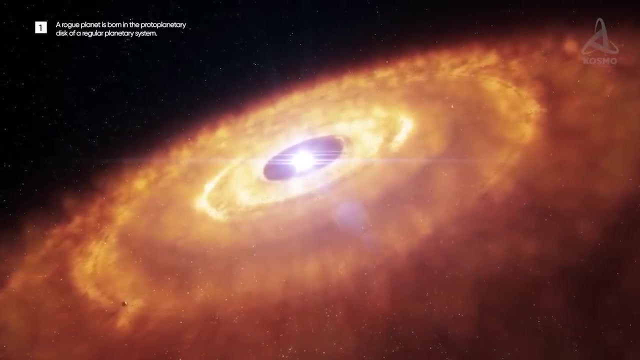 It is suggested that water is condensed into clouds made up of tiniest particles of ice. Today, it hasn't been established for certain how this object came to be. There are currently two versions suggested by researchers. According to the first one, a celestial object like that starts its life cycle. 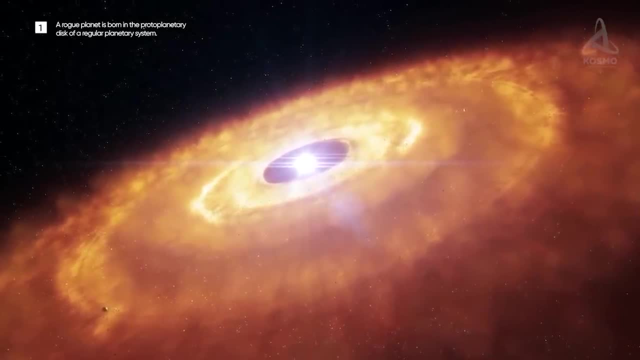 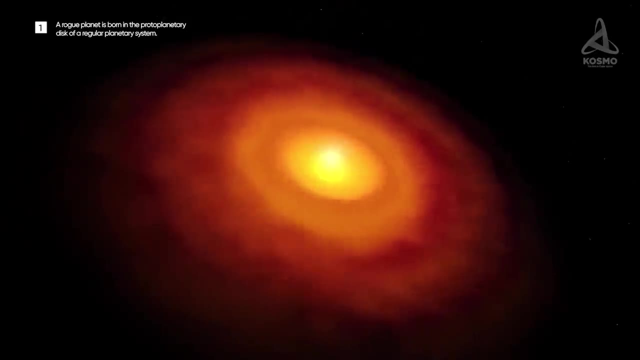 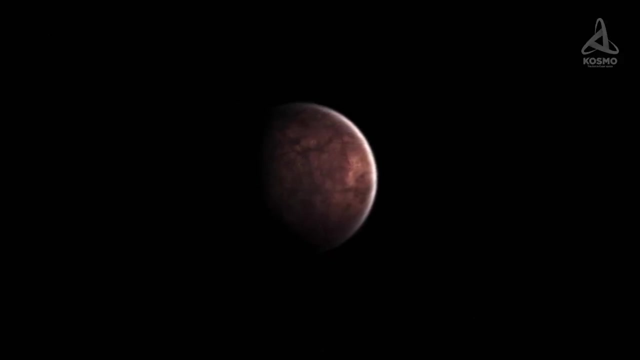 in the protoplanetary disk of a regular planetary system. Mathematical modeling of this process shows that if the original cloud of gas and dust is heavy enough, it is highly likely that at least one planet will be ejected beyond the system. The celestial object may also be forced out of its star's environs. 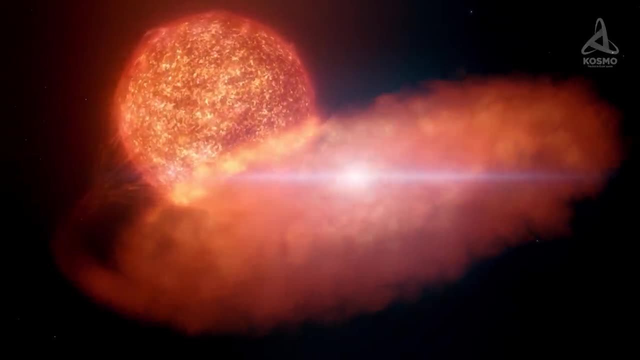 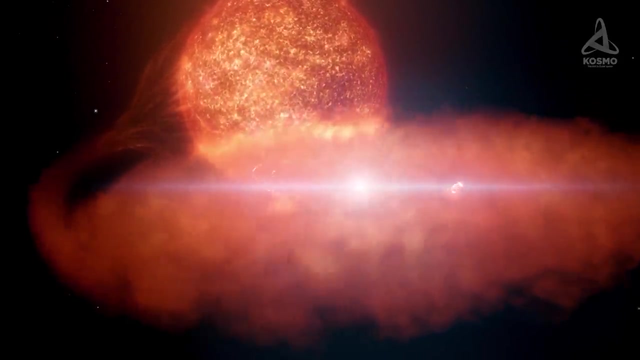 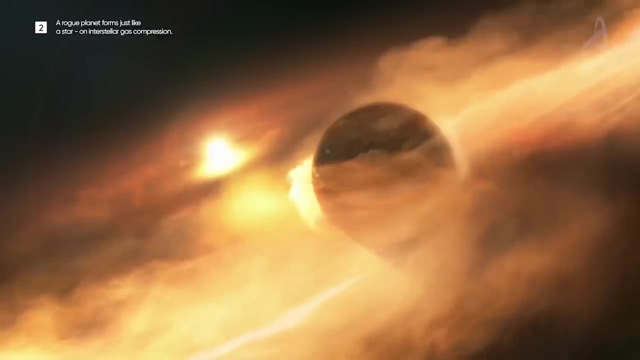 if another massive star passes it by, or else if its planetary system collides with another system. The chances of events like that are, admittedly, comparatively small. The other version has it that the space object was born just like any other star on compression of interstellar gas. 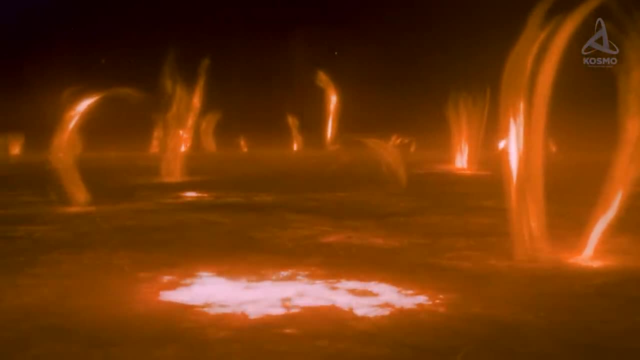 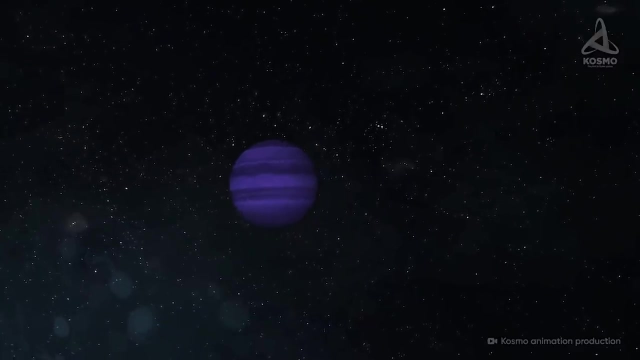 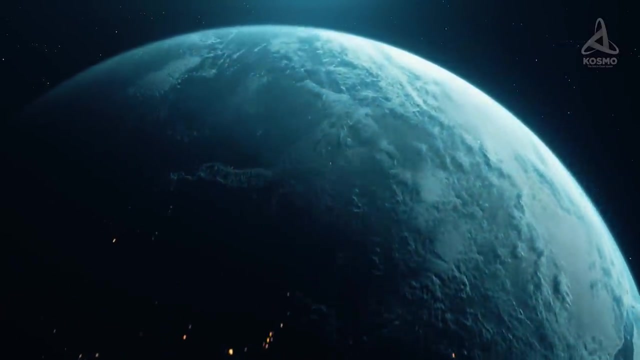 At the same time, the mass of the object proved to be too small to unleash any thermonuclear reactions in its interior. It goes without saying that in this manner, it may turn out only as a gas giant or a brown dwarf, but not a rocky planet similar to the Earth. 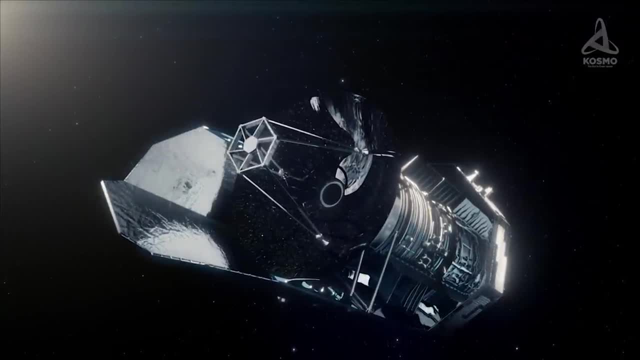 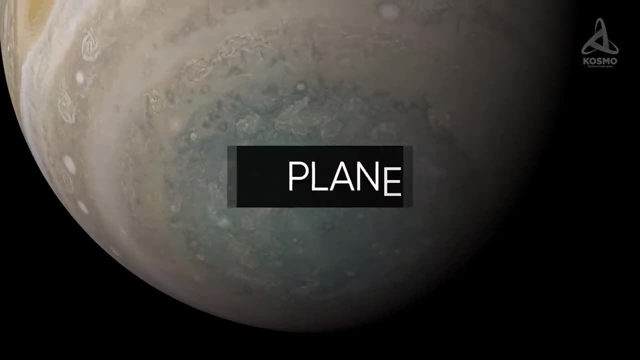 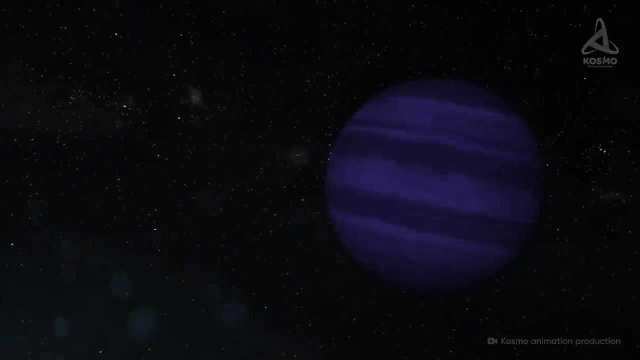 Some researchers don't agree that these objects should be seen as rogue planets and classify them as sub-brown dwarfs. instead, Others suggest using the term planemo for all interstellar wanderers that don't show any thermonuclear activity. Bearing in mind today's notions, 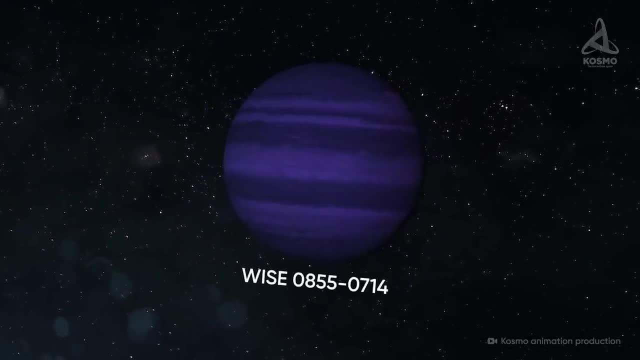 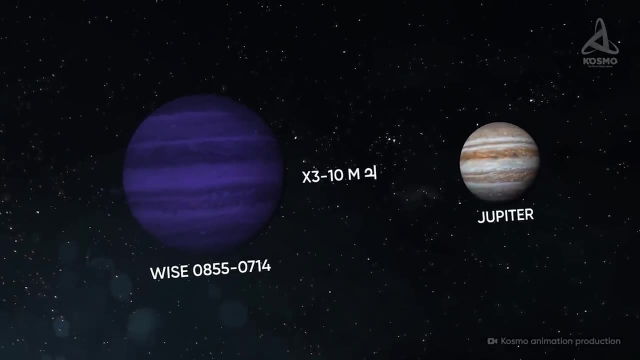 of the makeup of brown dwarfs and gas giants. we may estimate the mass of WISE 0855-0714 at anything from 3 to 10 Jupiter masses. This rather falls short of starting a thermonuclear reaction, but quite enough to keep the heat. 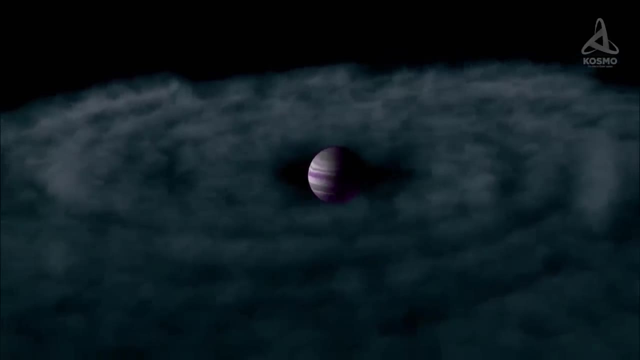 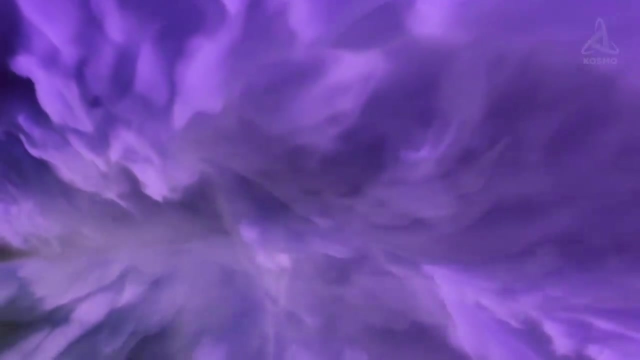 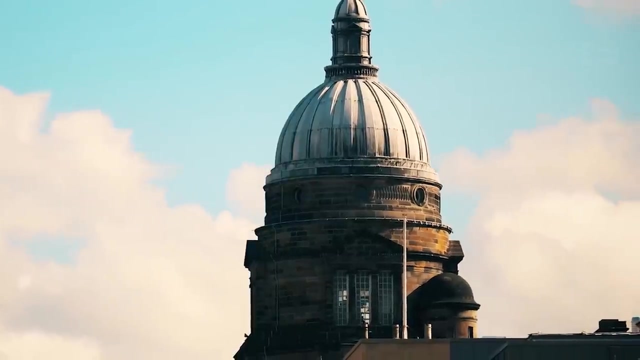 effectively trapped inside the planet. Taking into account our knowledge about natural laws, we can predict what the conditions on the astronomical bodies serve are like. For example, according to research by David John Stevenson from the University of California in the US, gas giants similar to Jupiter. 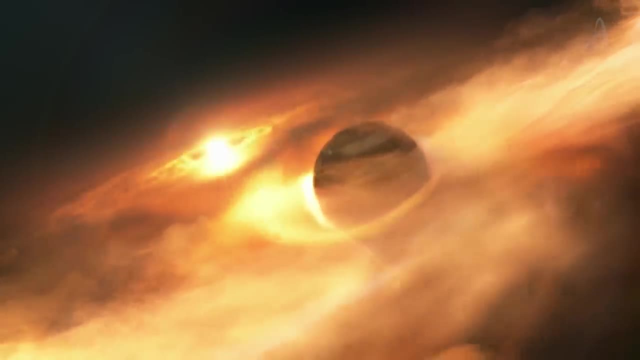 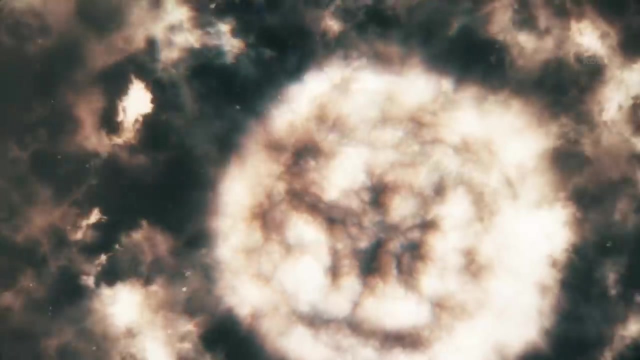 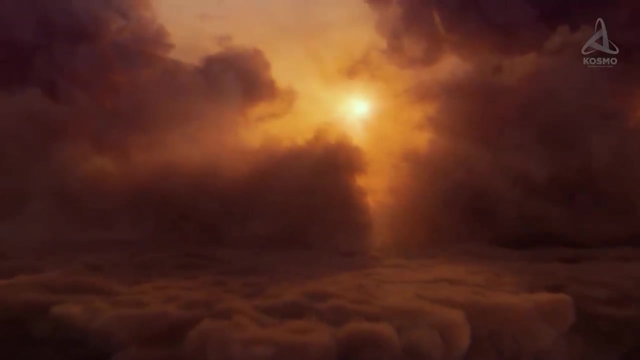 don't cool off instantly after receding from their star. Their thick hydrogen atmosphere is quite reliable thermal isolation, while the dense and hot nucleus made up of metallic hydrogen can keep the planet heated for a considerable time. Estimates show that the temperature of the lowest strata of a hypothetical celestial object 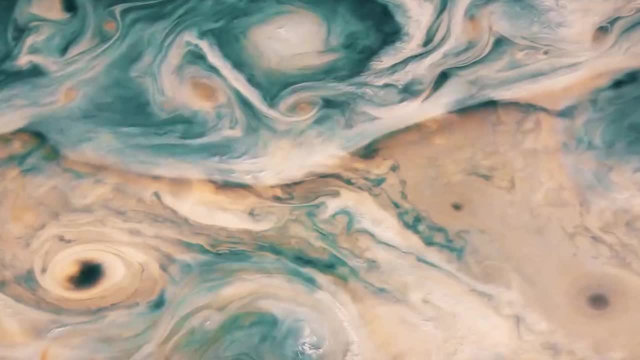 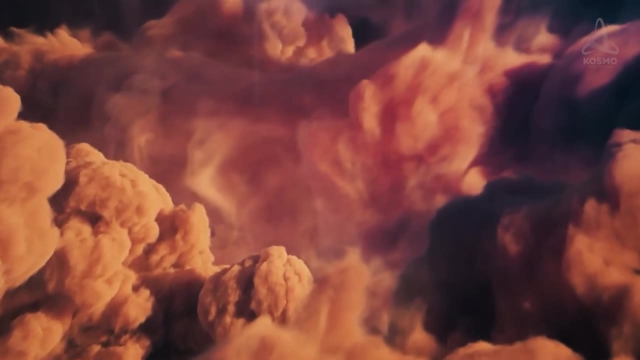 's atmosphere may be high enough for liquid water to be around, It is likely to be present in the atmosphere as giant clouds made up of tiniest droplets. These deductions agree with the results of mathematical modeling of WISE 0855-0714. 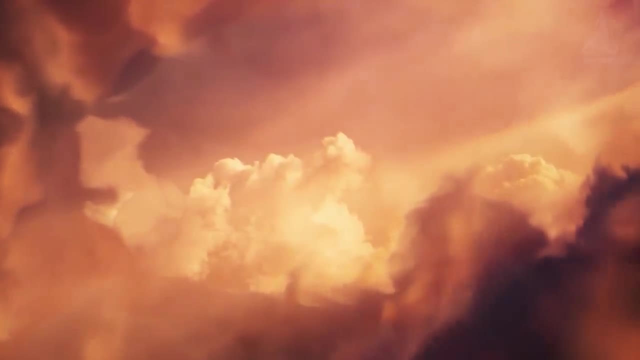 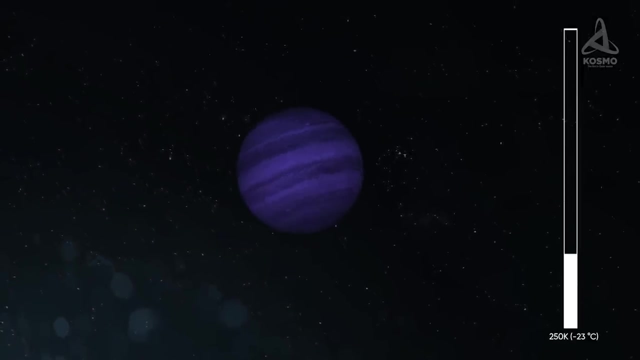 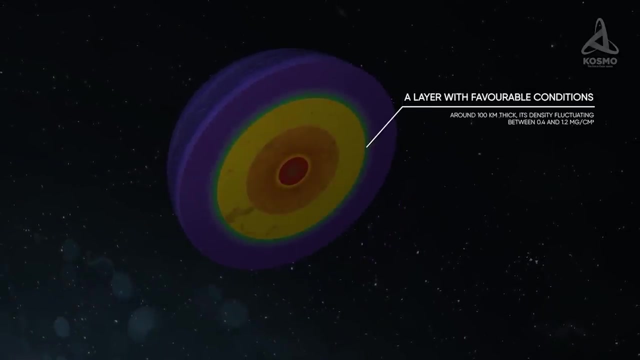 carried out by a team of scientists from the University of Edinburgh. It showed that the most likely temperature value of the planet's surface is 250 Kelvin, or 23 degrees Celsius below zero. The celestial body's atmosphere also has a comparatively warm layer around 100 kilometers thick. 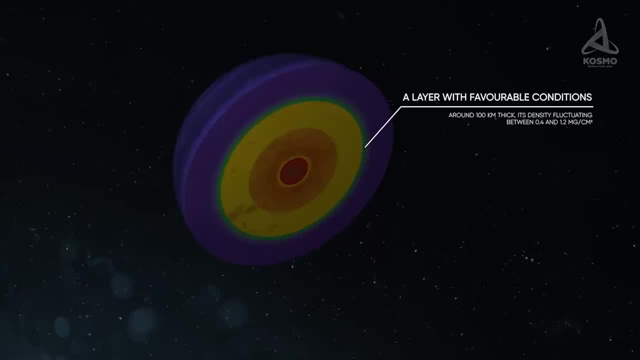 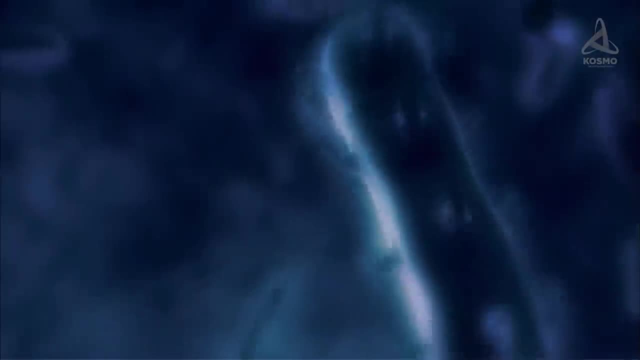 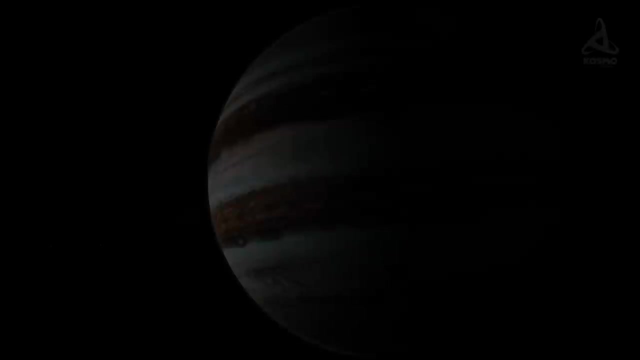 whose density fluctuates from 0.4 to 1.2 milligrams per cubic centimeter. It is comparable with the conditions on the Earth, and so it is thought that this environment should be favorable for potential organic life. Incidentally, a planet doesn't have to be. 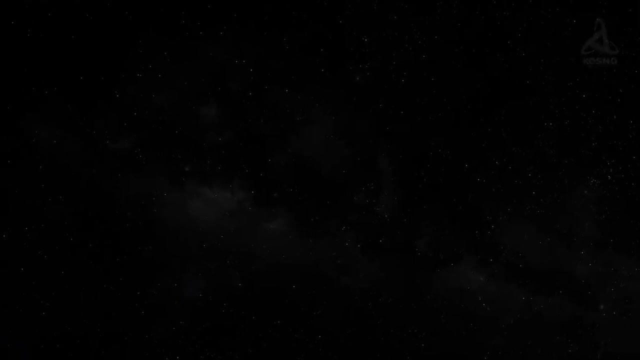 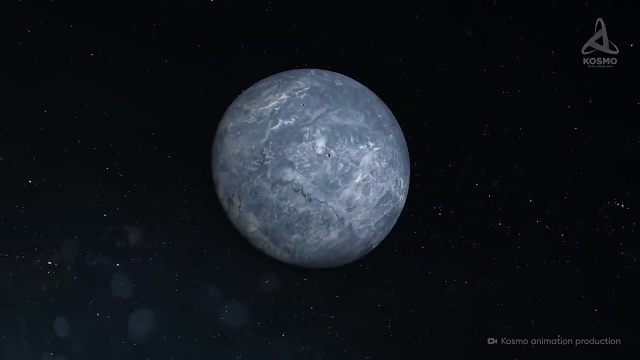 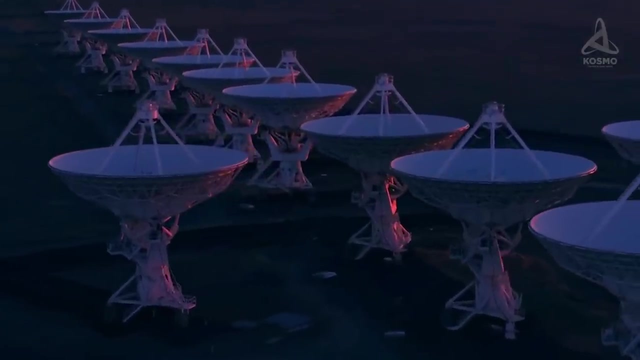 a massive gas giant to avoid freezing in the cosmos. In 2020,, a rogue planet candidate was detected using gravitational microlensing techniques, And here is the long designation it got. It is still awaiting confirmation of the rogue planet's status, and its parameters have been defined. 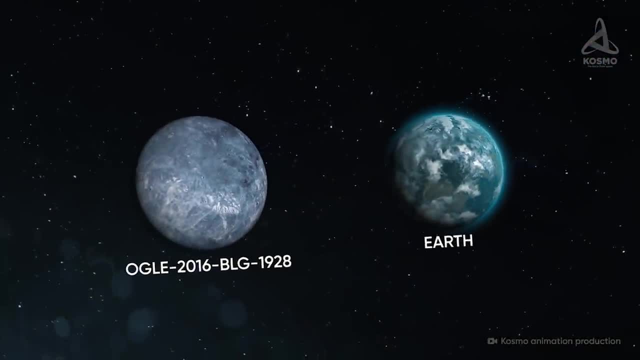 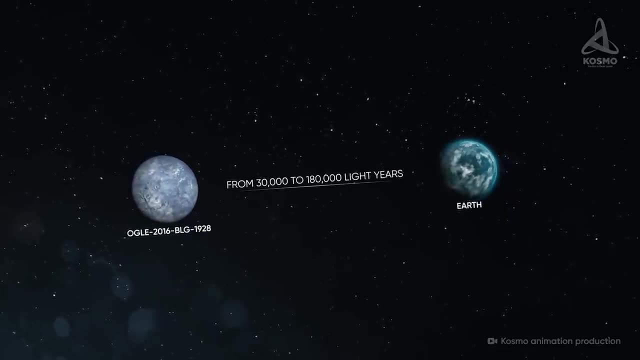 only generally so far. According to preliminary data, however, the object is comparable to the Earth in terms of its mass and is anything from 30 to 180 thousand light-years away According to our current scientific notions. an object with a mass like that- 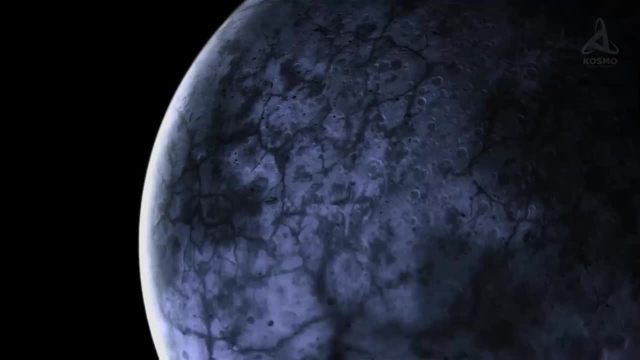 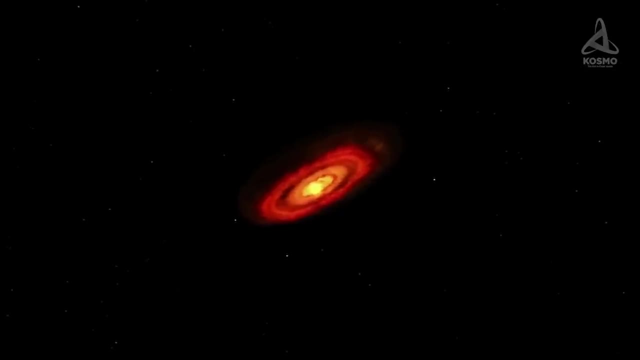 is not supposed to be a gas giant and is more likely to be a rocky planet. This, in its turn, offers good grounds to believe that the object formed in the protoplanetary disk of a planetary system as the latter was forming It, may have been ejected from the system. as a result of a cataclysm in space or, alternatively, under the influence of a larger neighbor. After that, it was left to its own devices, and so became a free-floating planet. What will happen to it next is predefined by a combination of several factors. 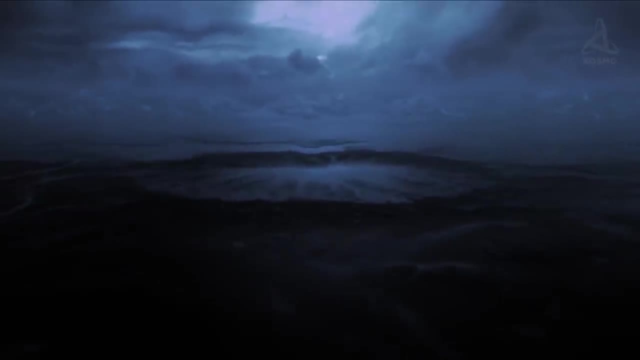 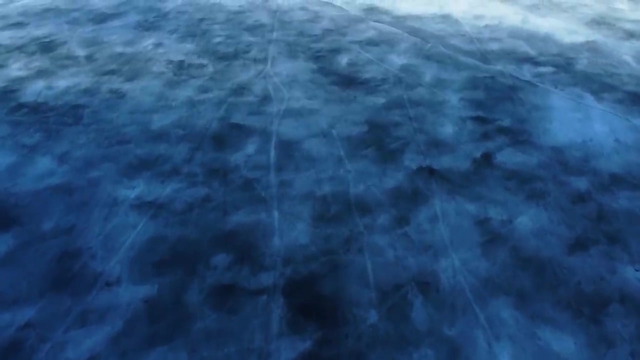 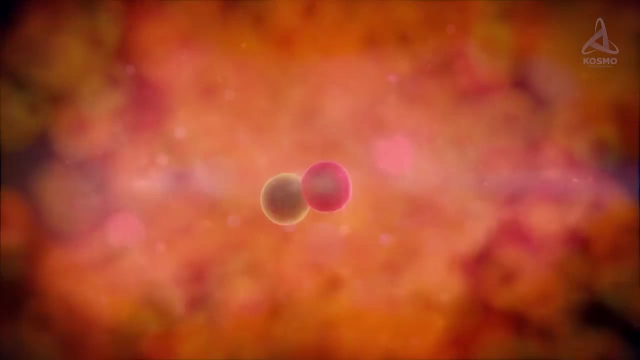 Provided the object's atmosphere is sufficiently dense, it will be reliably thermally isolated. Potentially, a layer of ice on its surface could produce the same isolating effect. In addition, with the object's interior scorching hot and with radioactive elements, 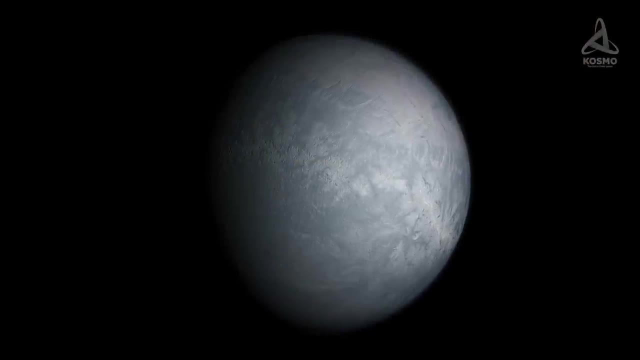 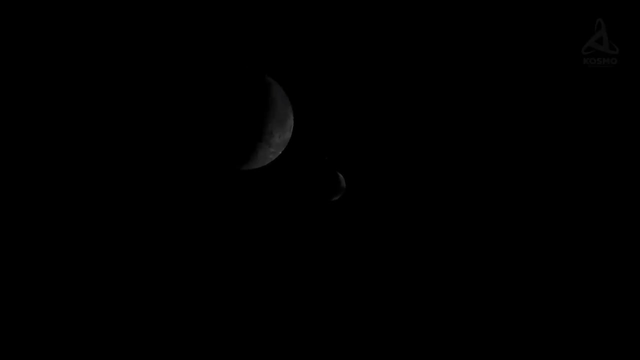 undergoing decay, most of the hypothetical ocean will remain in a liquid state. If the planet happened to have a moon, it may have retained it on ejection. If this is the case, tidal forces are likely to continue to deform and warm up the lithosphere. 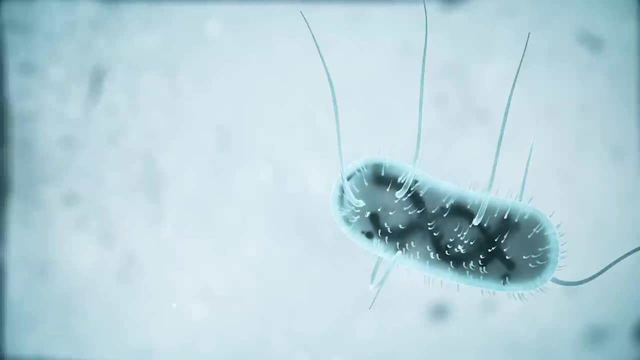 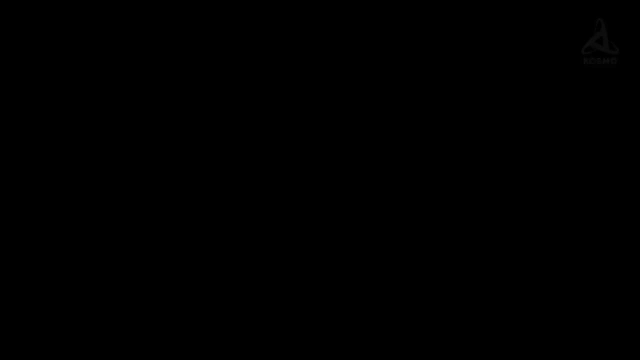 Theoretically, with any luck, primitive anaerobic life forms may have stayed around, although, of course, it would be next to impossible to discover their traces now. Most of the data about the rogue planets we know today were arrived at following mathematical models. 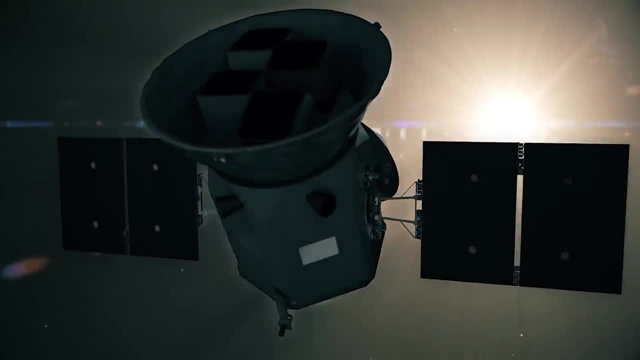 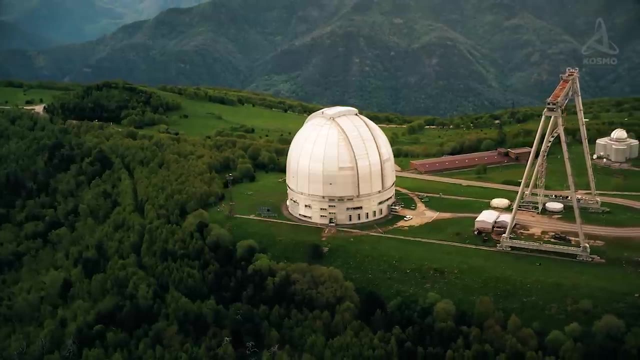 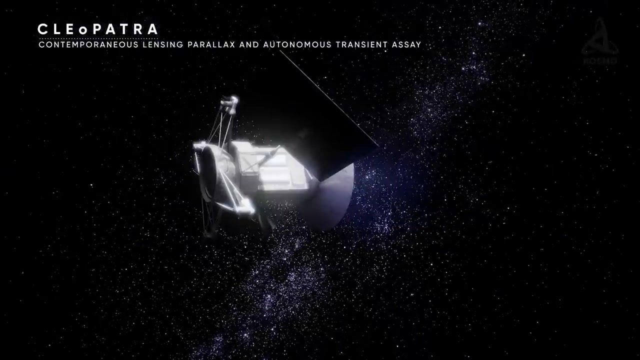 and complex calculations. It was possible to do these calculations thanks to the tiniest bits of information gleaned with the help of orbital and Earth-based telescopes. Even as I speak, a project is being worked on known as Cleopatra. Its main objective will be to search for free-floating planets. 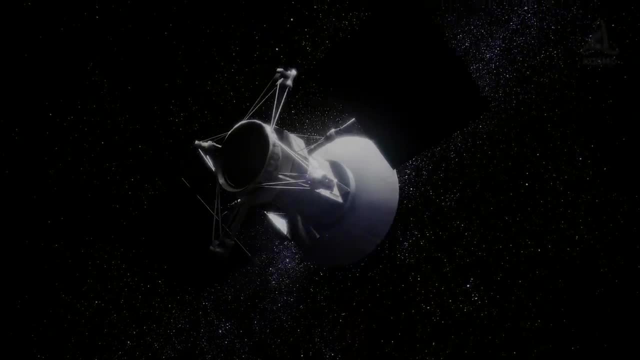 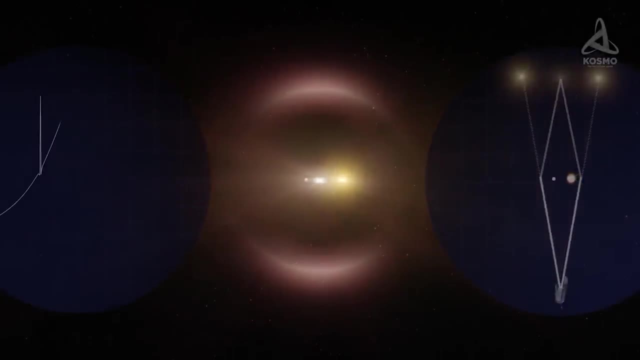 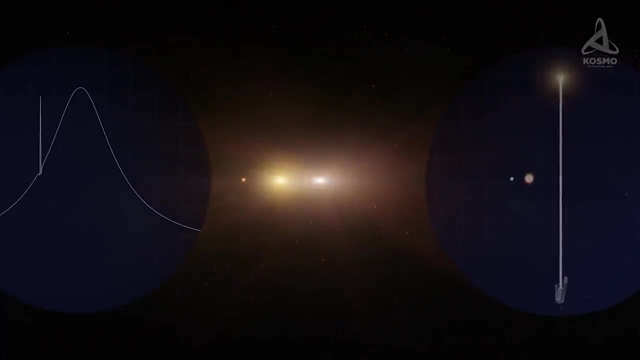 and other objects in space, with subsequent definition of their parameters. The project relies on something called microlensing. It is a phenomenon when a celestial body passes between a remote star and the observer on the Earth and briefly interferes with the light emitted by the remote star in the background. 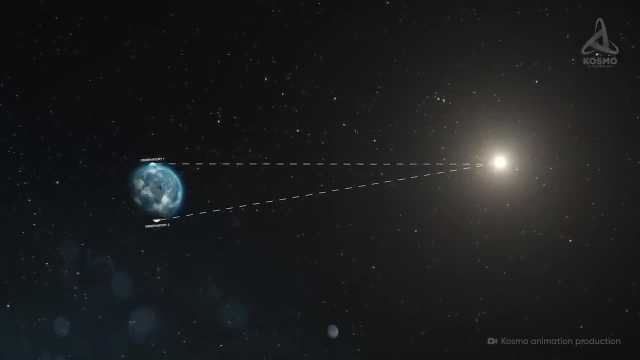 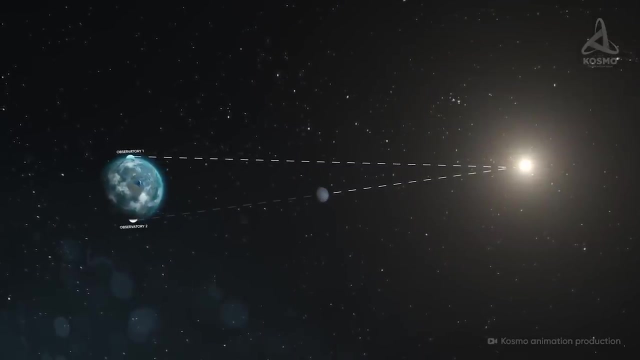 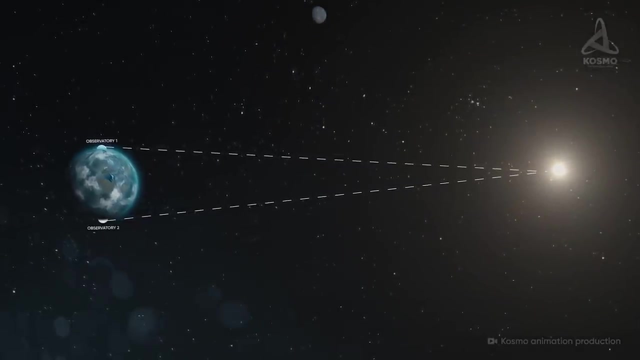 When observed from different angles, the moment of transition will be registered a fraction of a second sooner in one observatory than in another. Referred to as lensing parallax, this effect allows scientists to gauge the distance to a detected object, as well as its mass and dimensions. 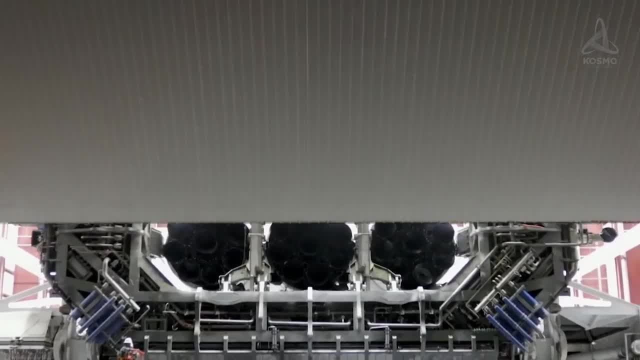 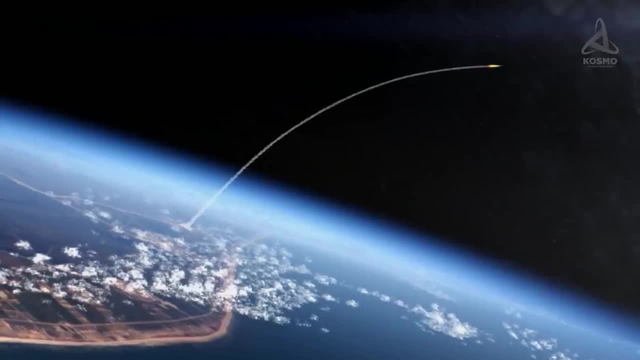 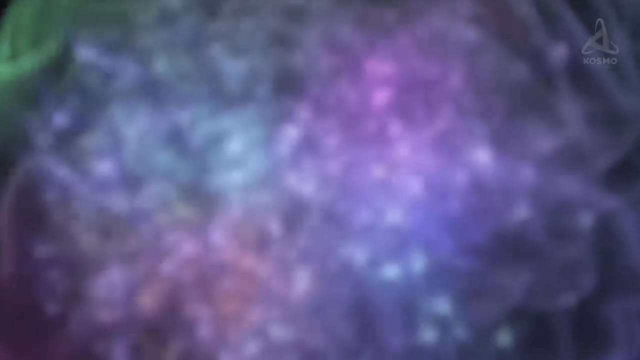 An interplanetary spacecraft is planned to be created within the project. It is supposed to blast off the surface of the Earth as soon as in 2025, alongside a mission to Mars, after which it will enter its own orbit around the Sun. The project will be aided by a specialized 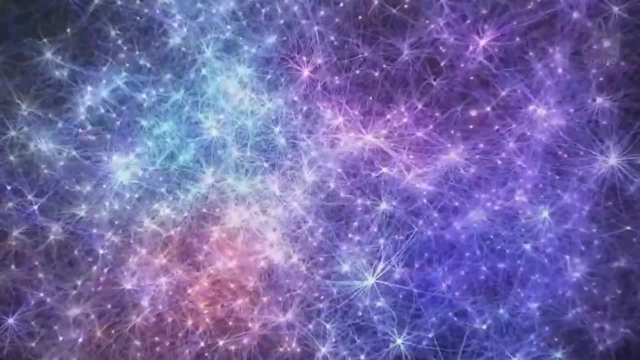 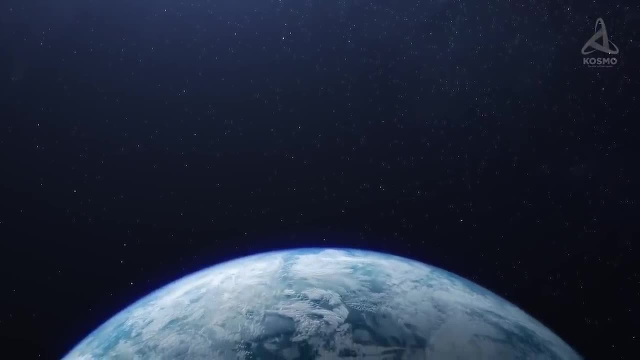 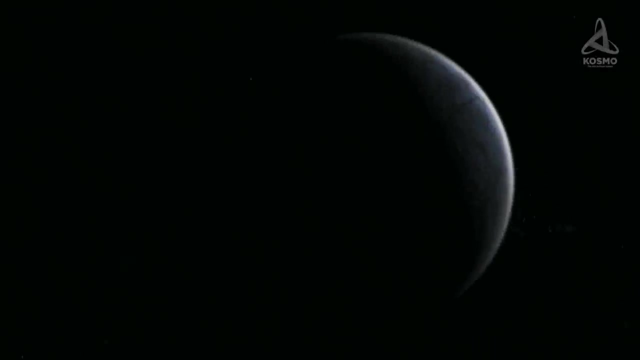 artificial intelligence component whose mission will be to process and analyze collected information. The Cleopatra project will certainly delight us with a wealth of exciting and important information, so there is a lot to look forward to. What is to become of all those rogue worlds out there? 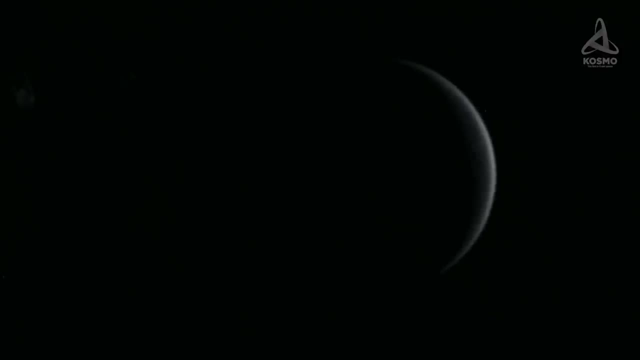 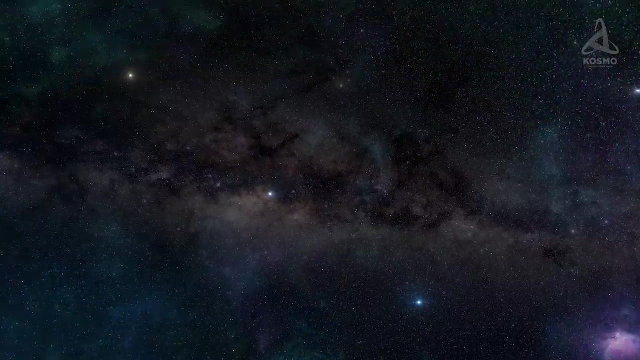 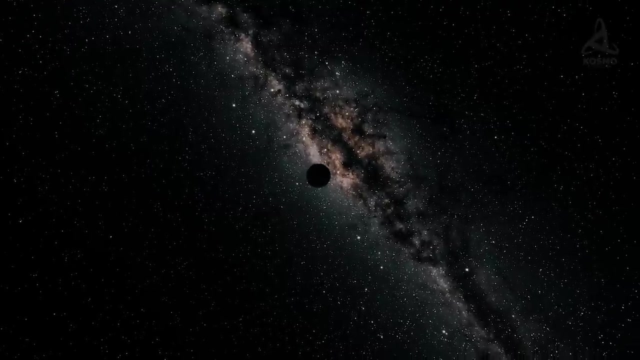 drifting quite by themselves in the dark depths of the Universe. In theory, an orphan planet may be captured by the gravitational field of a star and become part of its planetary system, but this chance is by all accounts minuscule. Most objects like that are destined to wander. 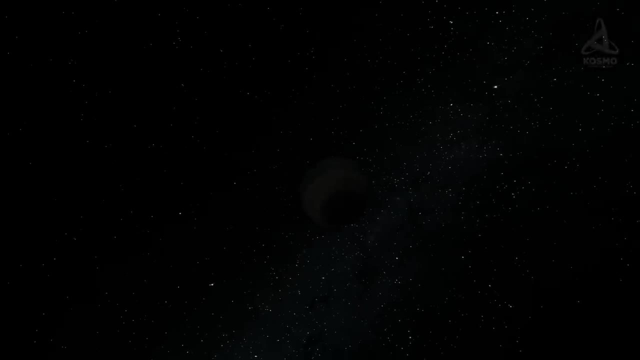 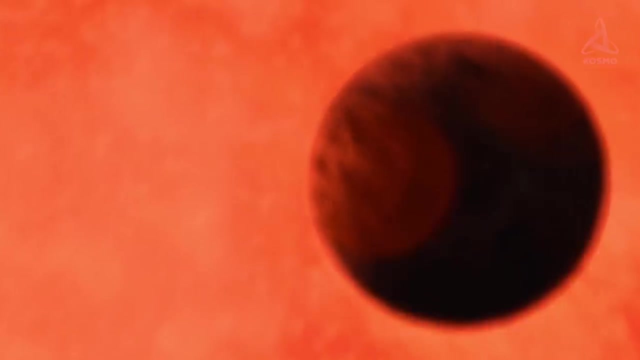 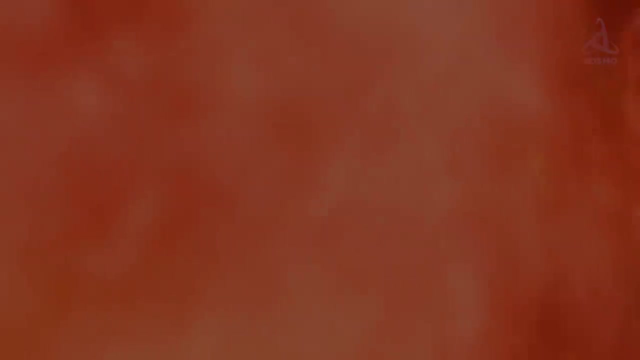 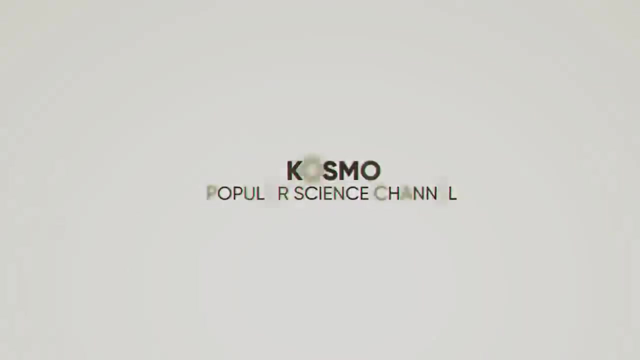 for billions of years through endless expanses of space, while slowly and inevitably cooling off, eventually there to be swallowed up by black holes or else destroyed as a result of a cataclysm in space, never to reveal their secrets to mankind. There are quite a few really scary places in our Universe. 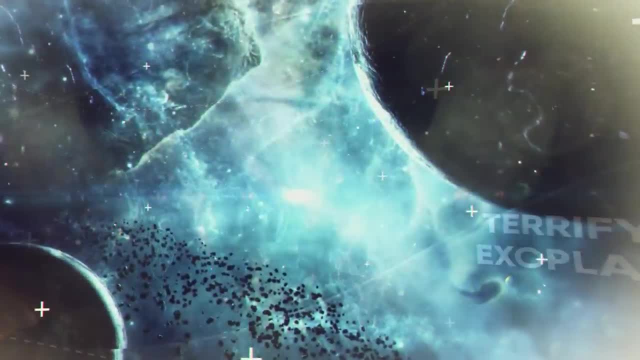 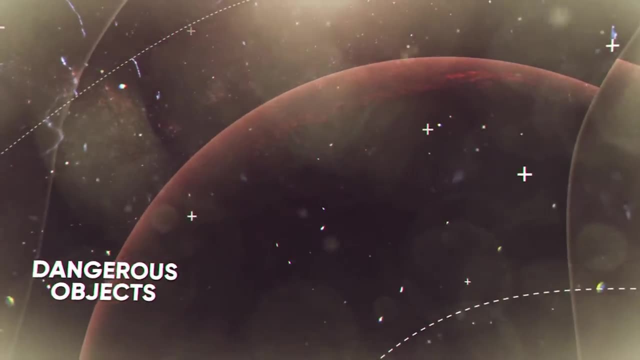 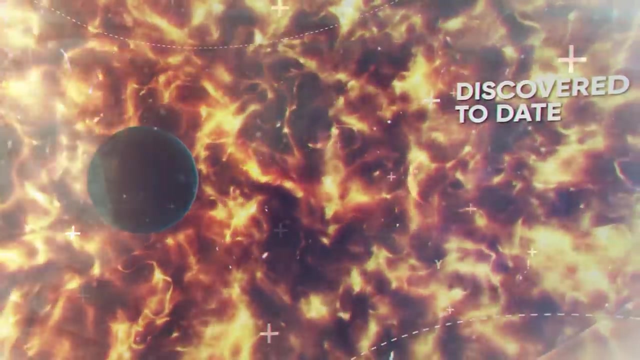 Most of them are cold worlds with no chances of life ever evolving there. But even among all this gloomy diversity, some objects can be singled out that may rightfully be called the most dangerous exoplanets ever discovered. by now And today, I invite you to check out the most incredible ones. 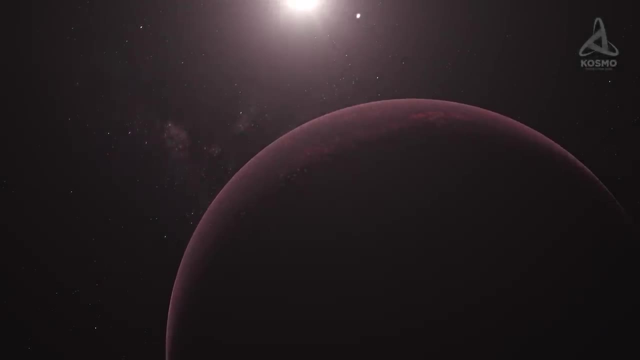 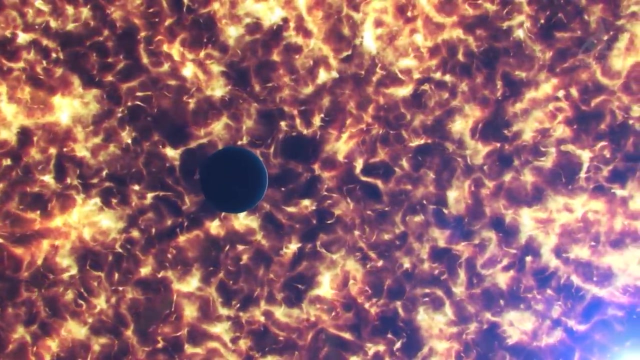 Shortly before Halloween in 2020, NASA compiled a list of the most terrifying worlds. Among others, they included six exoplanets. each of these objects' environments is not just extremely harsh for any living organism, even finding oneself in their comparatively close proximity. 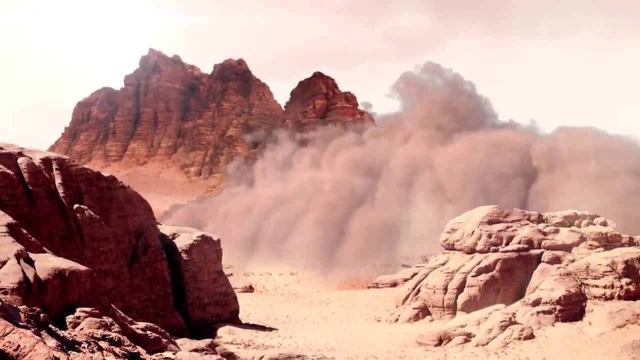 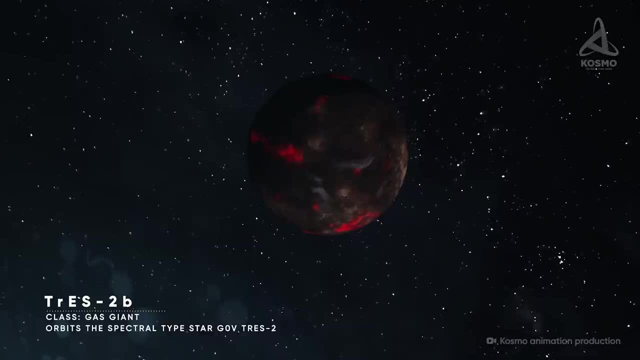 may prove to be fatal. The first object on the list is a black gas giant designation TRES-2b. This celestial object orbits the star TRES-2,, which is a yellow dwarf lying as far as 718 light-years away from us. 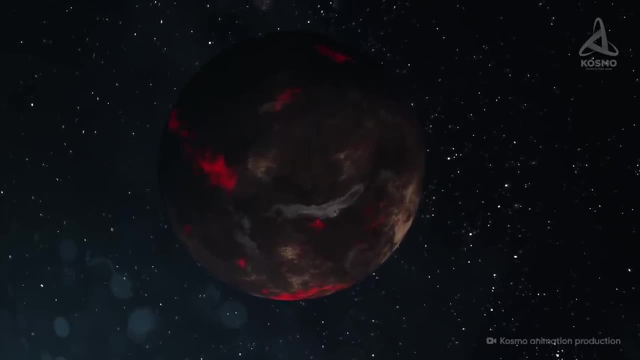 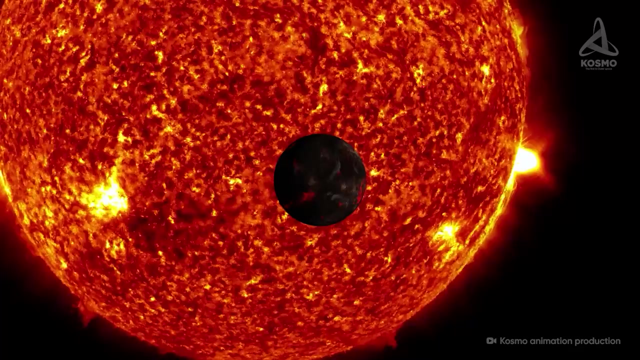 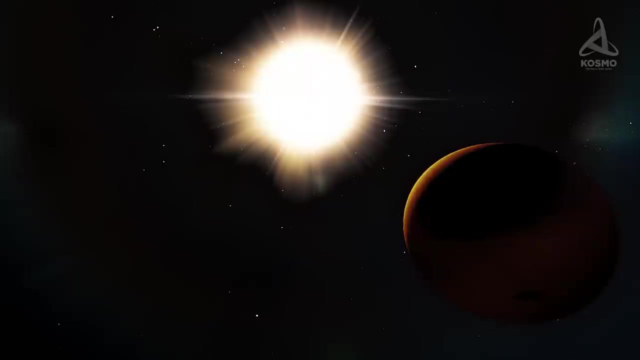 This object is also known as a black gas giant. Let's take a closer look at it. Due to some unique properties of the chemical composition of the surface of TRES-2b, the planet absorbs over 99% of all the light shed on it. 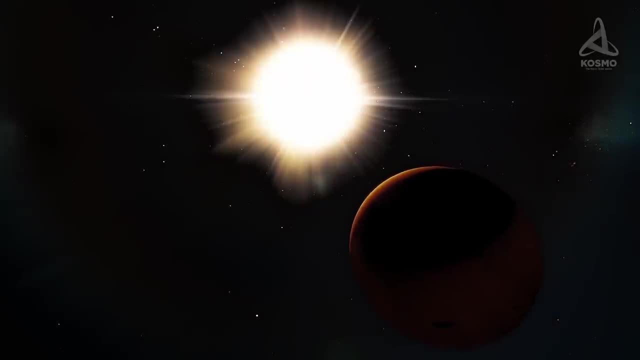 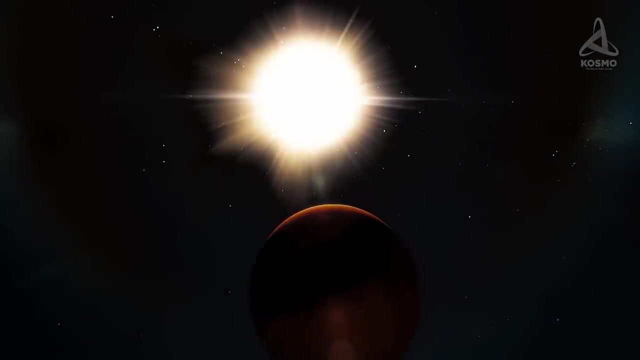 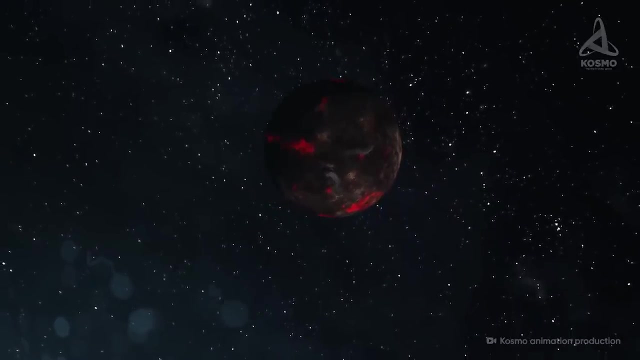 The nature of these properties remains a mystery, and chances are there are some chemical reactions taking place on the surface that we have never registered on any similar object before, And it is these properties that make TRES-2b the darkest exoplanet on the astronomical map of today. 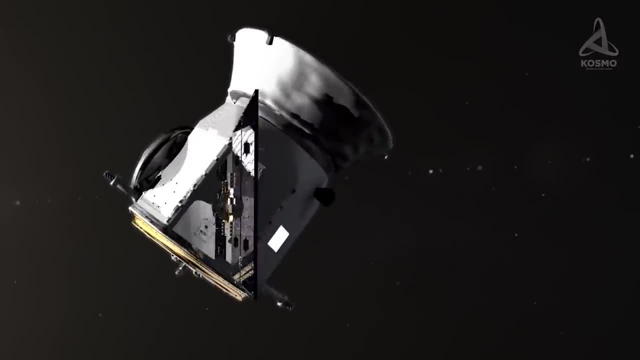 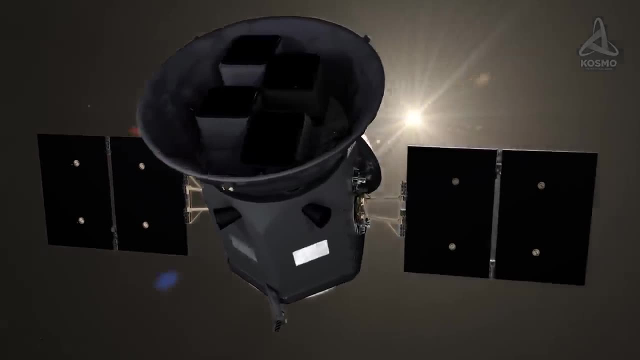 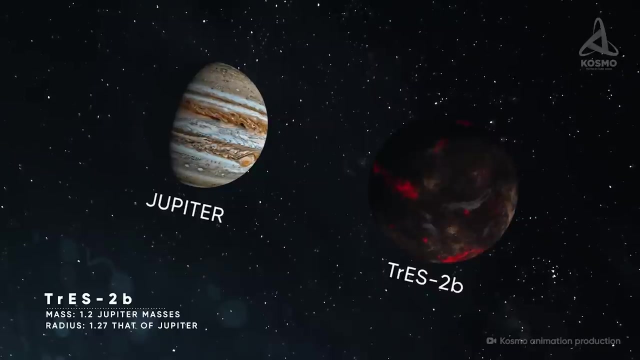 This gas giant was discovered on the 21st of August 2006,, with more details on its characteristics obtained several years later. The mass of TRES-2b is 1.2 Jupiter masses and its radius measures 1.27 times that of Jupiter. 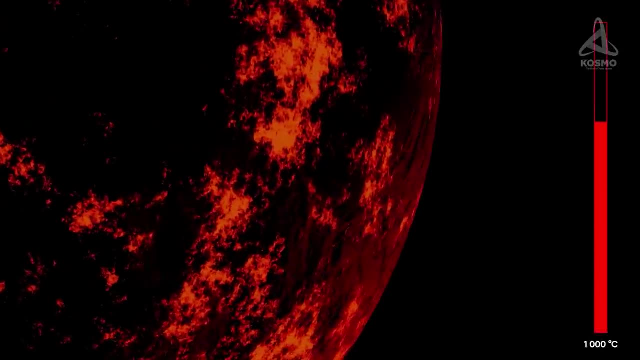 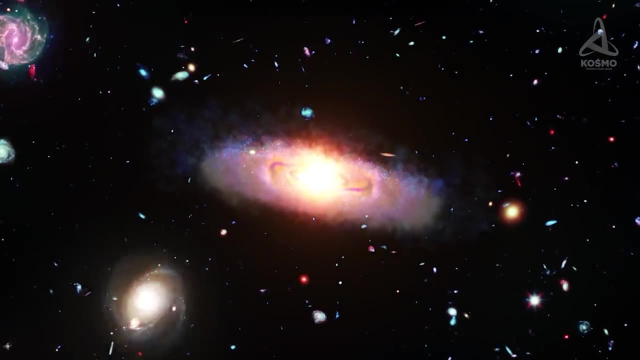 The atmosphere is as scorching as 1000 degrees Celsius, which gives the exoplanet a faint red glow like that of embers. Still, in spite of its gloomy looks, TRES-2b doesn't really qualify to be called. 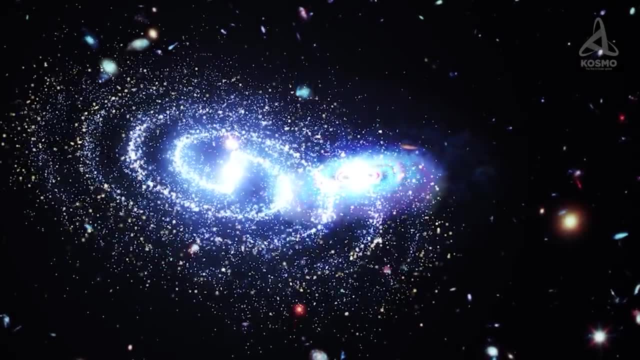 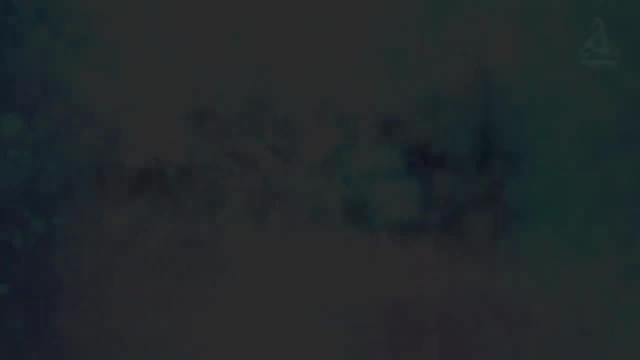 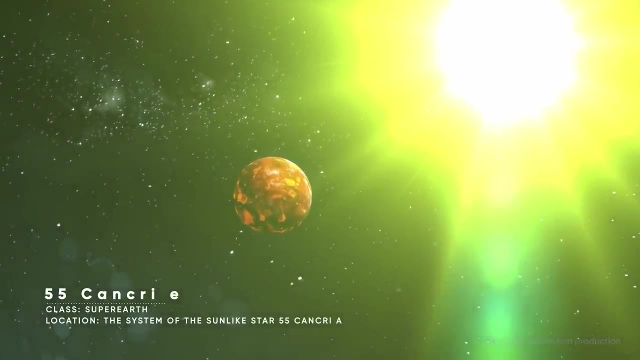 the most dangerous place in the Universe. There are many more objects lurking in space that are more terrifying than that. Let's see some more inhospitable ones. Here is another exoplanet, designation 55 Cancri, e It lies in the system of a sun-like star. 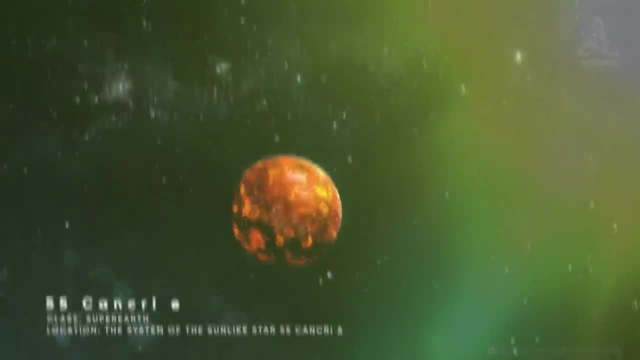 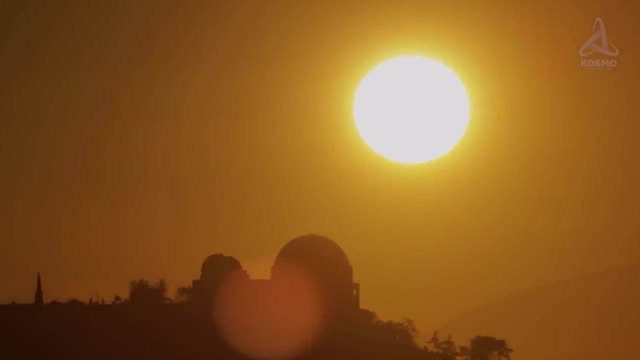 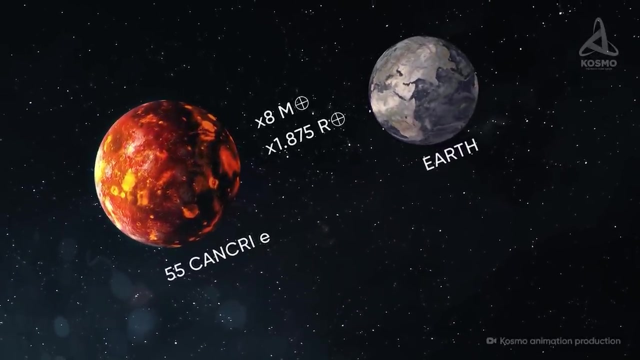 designation 55 Cancri a. This celestial object was discovered on the 30th of August 2004 by the Doppler spectroscopy method. Let's look at it in more detail. The planet's mass equals approximately 8 Earth masses and its radius measures 1.875 that of the Earth. 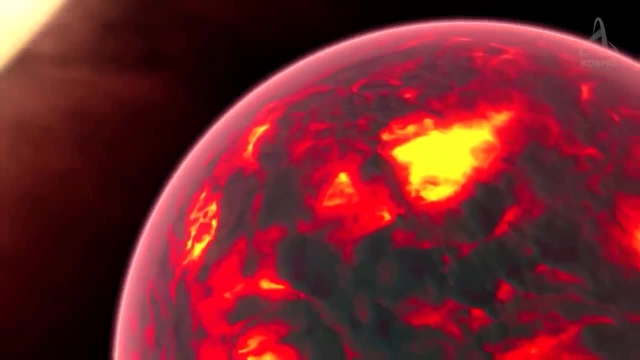 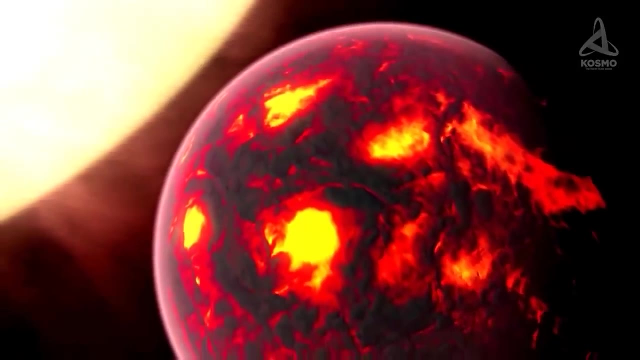 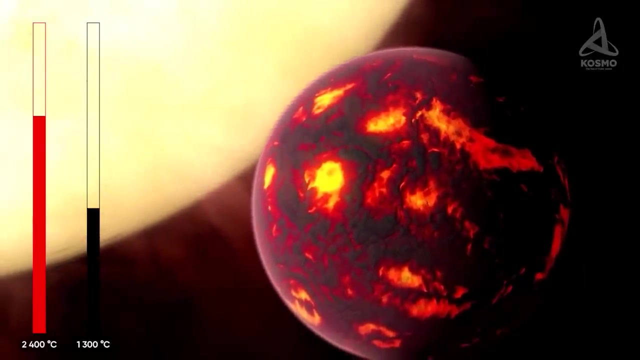 55 Cancri e is tidally locked, and so it is always daytime on one side and nighttime on the other. That is why the side facing the host star is always heated up to a temperature reaching 2400 degrees Celsius, with the temperature on the night side 1300 degrees Celsius. 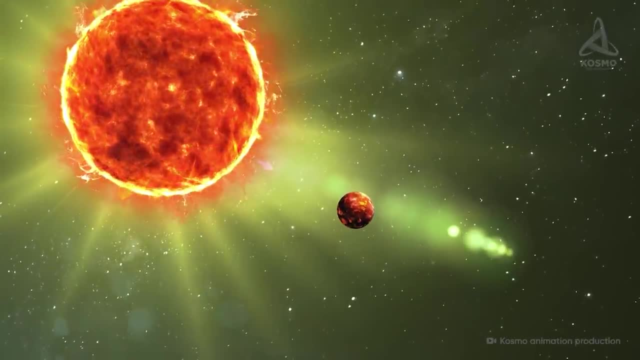 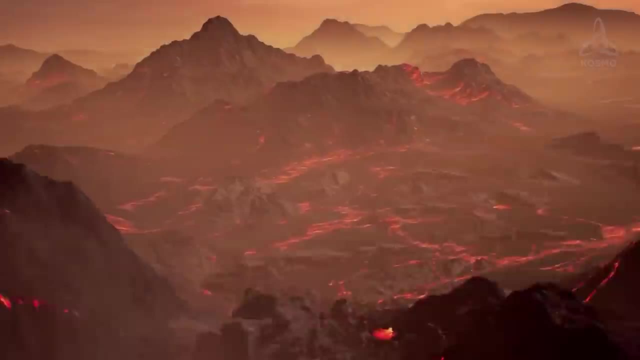 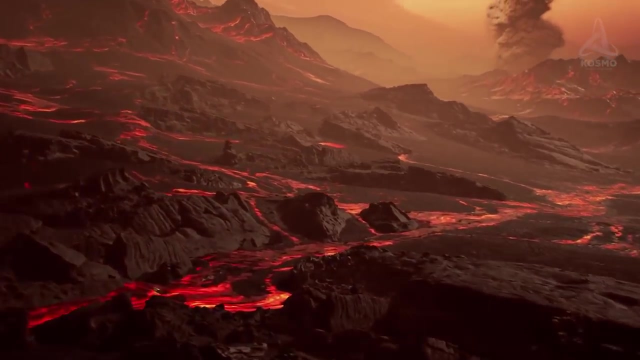 These values are so high because the distance between the planet and its parent star is just 0.0183 astronomical units. Besides, volcanism on 55 Cancri e, which is thought likely to be there, causes dust cloud emissions. These clouds trap heat. 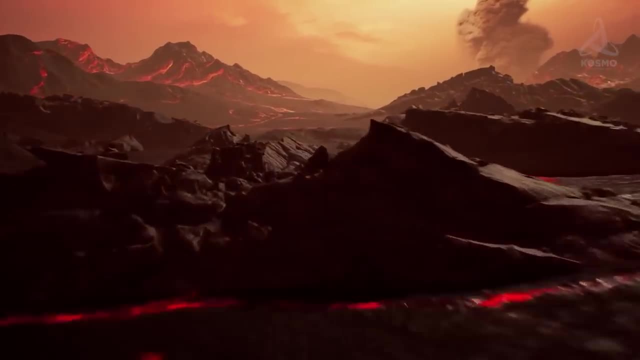 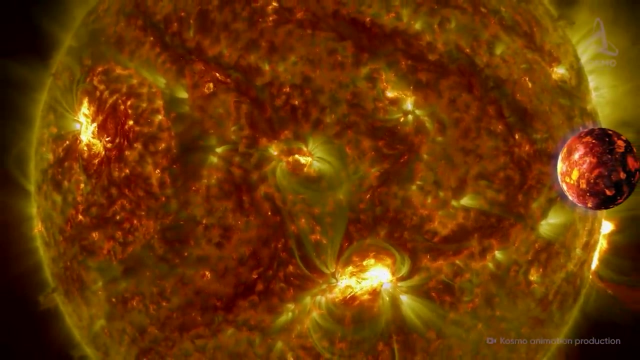 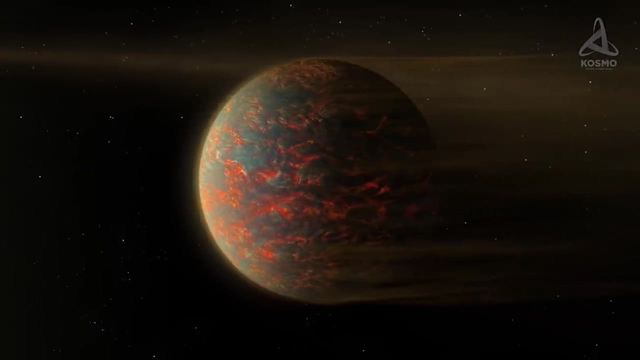 and effectively prevent it from escaping into space. The planet's orbital period is slightly under 18 hours. As for the atmospheric makeup, there is helium and hydrogen registered in it. There are also large amounts of carbon. Incidentally, this element is likely to form thick layers of graphite. 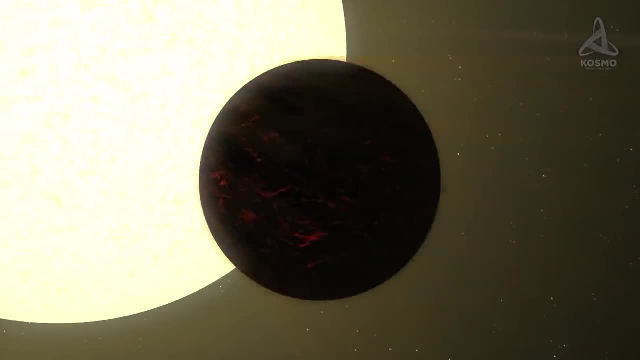 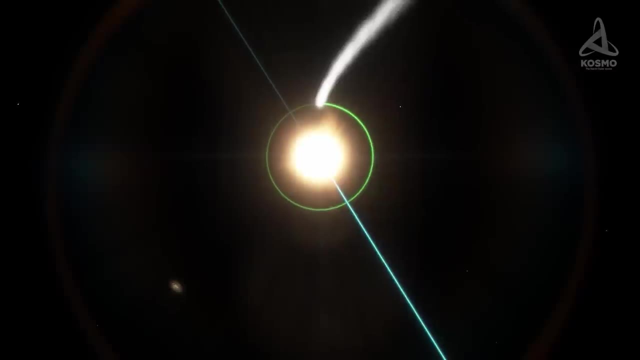 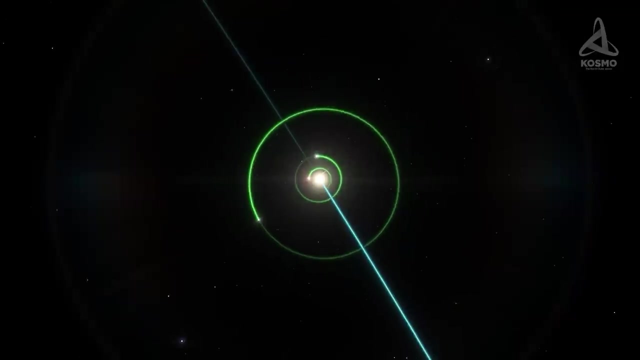 and diamonds in the planet's interior. 55 Cancri e isn't the only object in the planetary system of its host star. There are four other celestial objects orbiting it. The environments on these are by far more hospitable, which is the feature by which the 55 Cancri a system 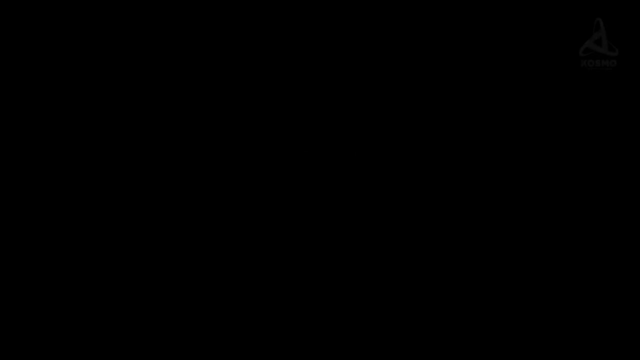 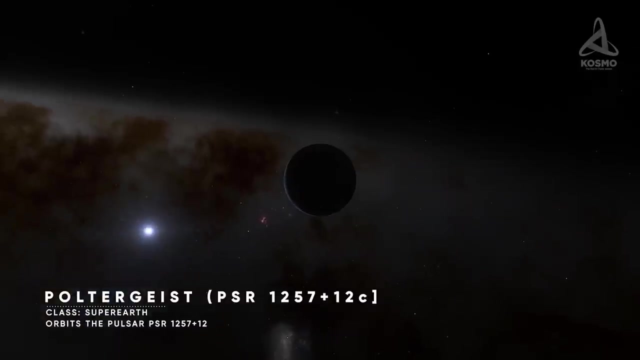 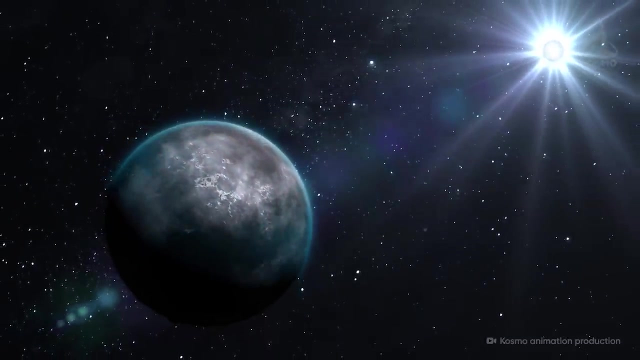 differs from the following object. It is dubbed Poltergeist, or PSR 1257 plus 12c. This is an exoplanet lying in a pulsar system. The celestial object is located just 0.36 astronomical units from the system's center. 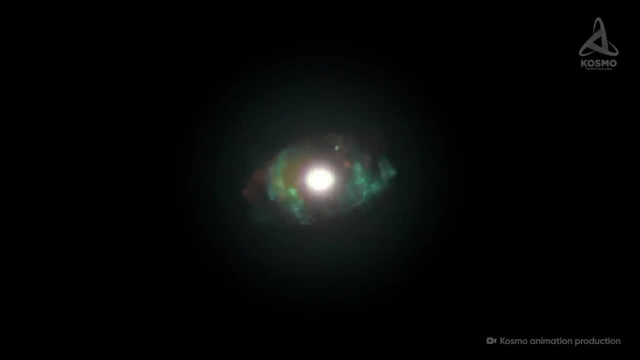 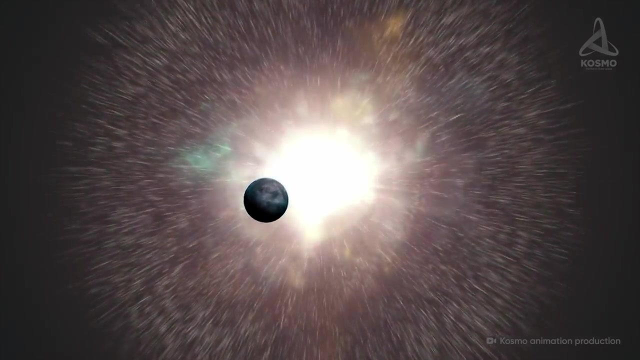 This shows that Poltergeist wouldn't have survived a supernova. that must have taken place before the pulsar had been formed. Consequently, the exoplanet is likely to have formed after this tremendous event, with the material for it coming from the nebula left after the explosion. 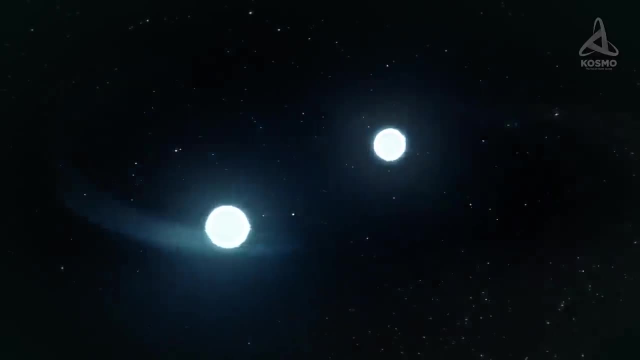 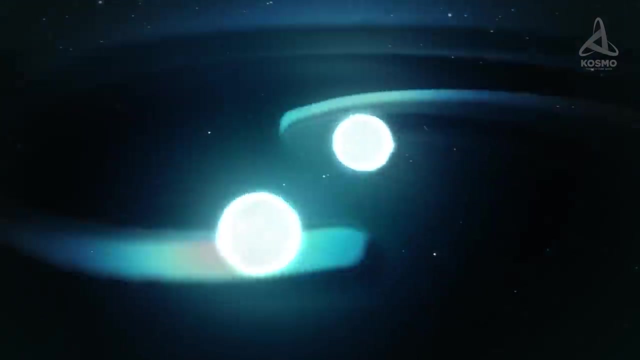 According to another hypothesis, the pulsar may have formed after the merging of two white dwarfs. Unlike with a supernova, this process isn't always accompanied by a powerful blast. Still, as this is the first object of its kind we have discovered, 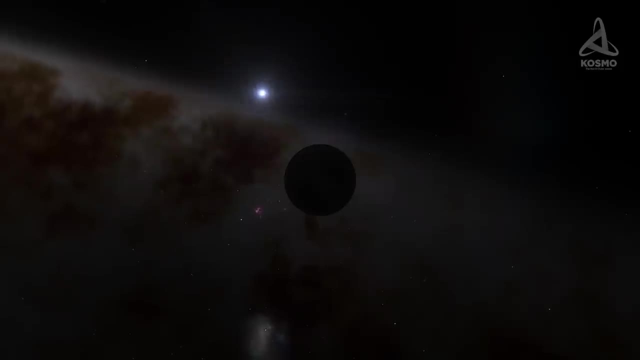 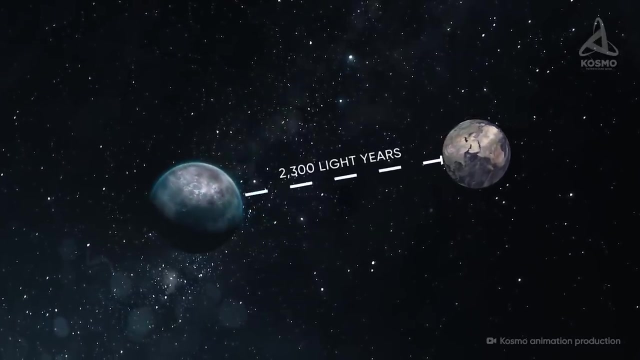 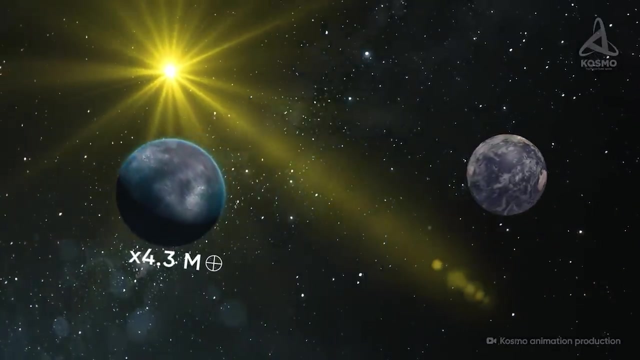 science cannot give a definite answer as to its origins. The system with the celestial object lies 2,300 light years from the Earth. Its mass is approximately four times that of our planet. As for its orbital period, it is around 66 days. 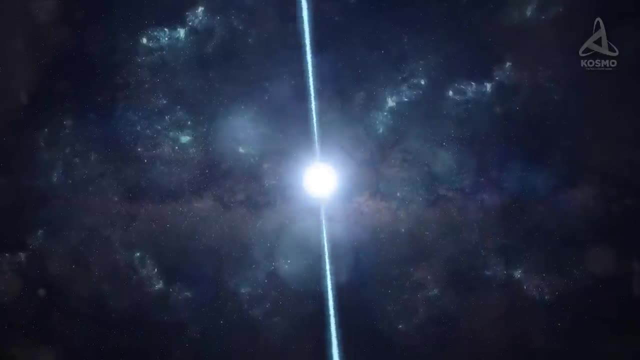 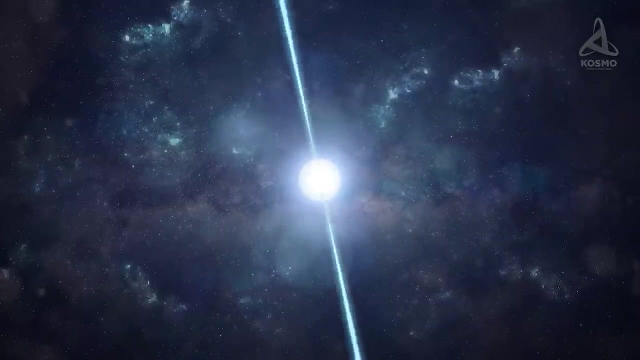 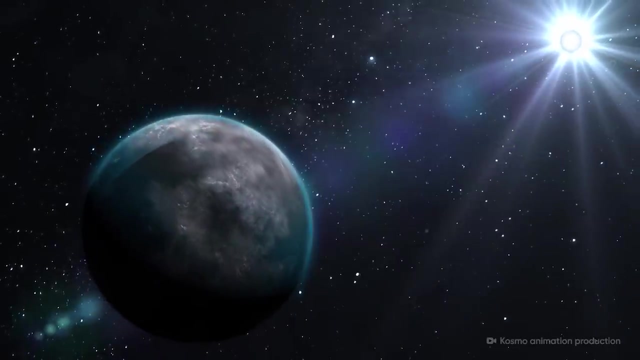 Incidentally, the outstandingly powerful radiation emitted by the pulsar is enough to crumple any spaceship wanting to approach the mysterious exoplanet in its system. Even with all these properties taken into account, Poltergeist does not really qualify as the most dangerous exoplanet known to us. 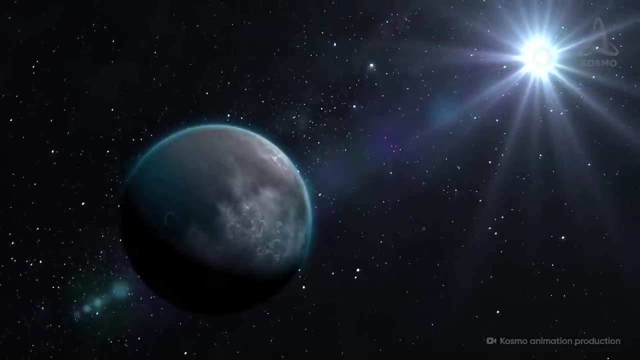 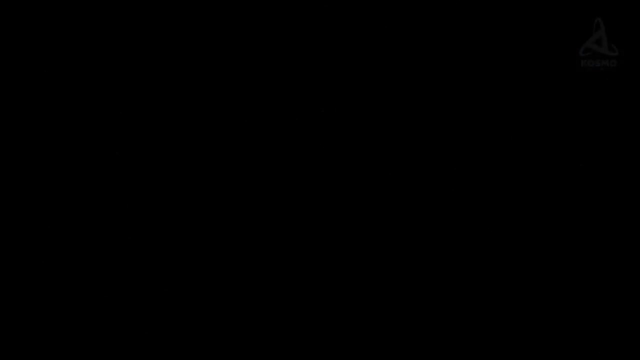 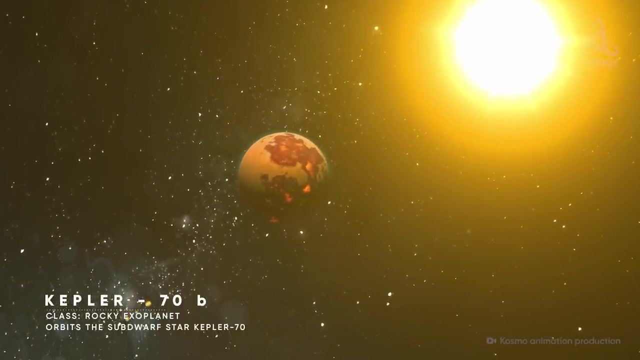 On approaching it. an astronomical body may simply get destroyed, but it would get positively vaporized in close proximity to the following object. The reason for this effect is the extremely high temperature on Kepler-70b, which is the hottest exoplanet known to us. 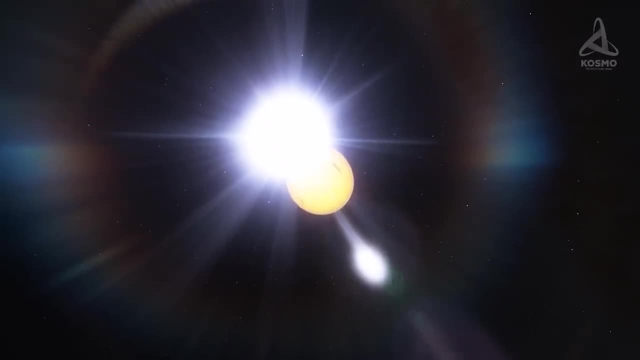 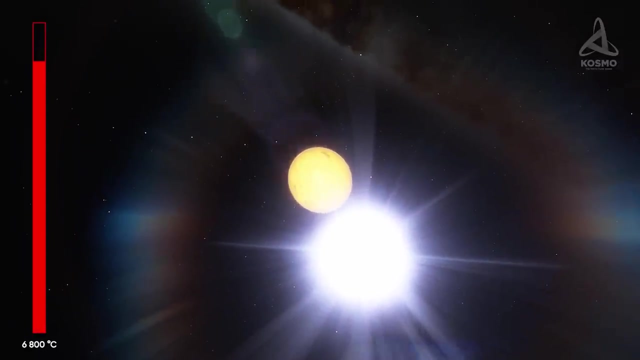 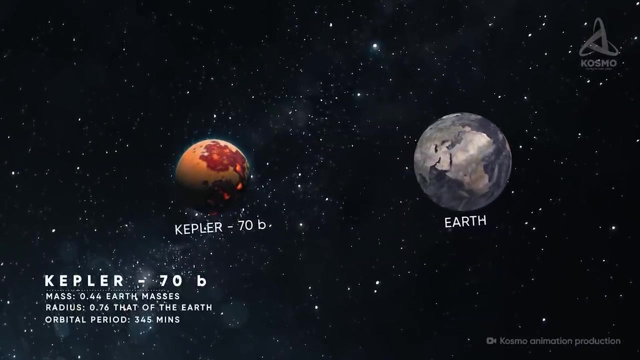 The object orbits the sub-dwarf star Kepler-70.. With a surface temperature higher than that on our Sun, it reaches 6,800 degrees Celsius. The object's mass is about 0.44 Earth masses and its radius measures 0.76 that of the Earth. 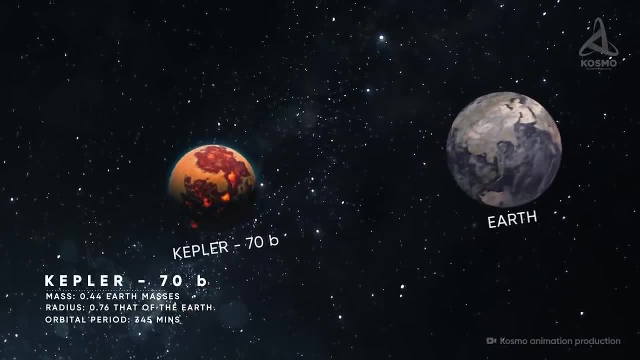 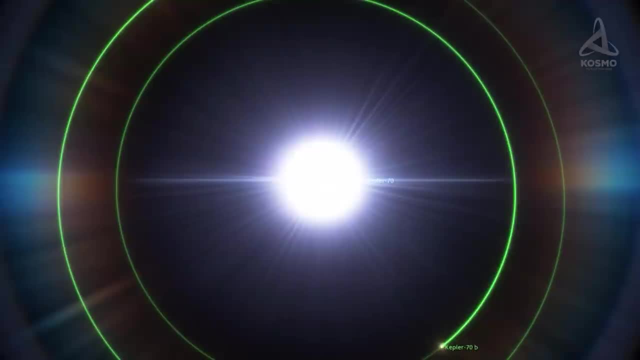 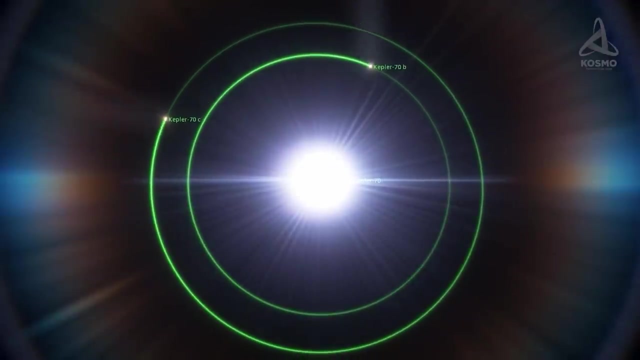 The celestial object's orbital period is 345 minutes, In other words, a day here is less than six hours long. Interestingly, the exoplanet regularly passes another object in the system, Kepler-70c, at a distance of 240,000 kilometers. 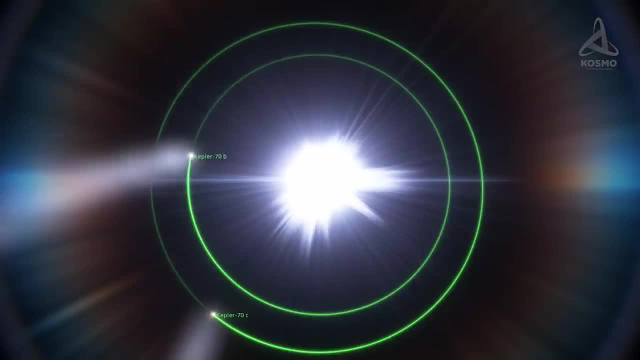 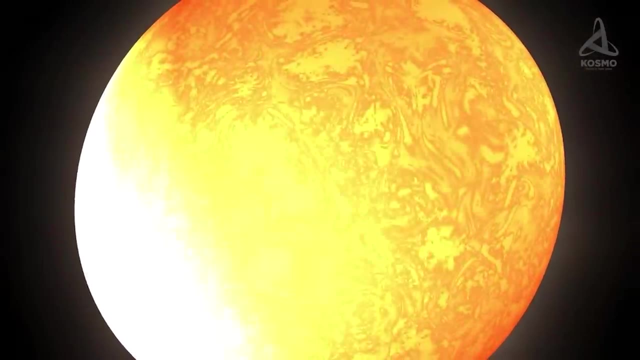 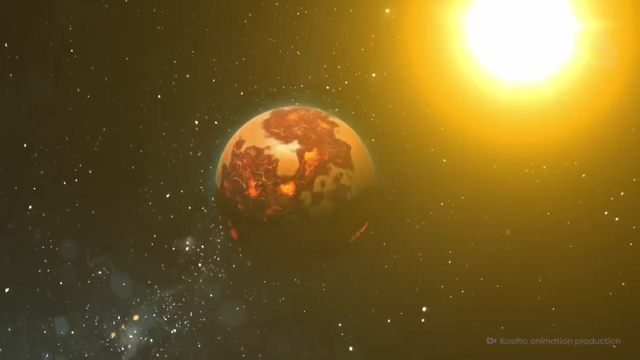 To date, this is the closest that planets in space have been registered to pass each other. The extremely high temperature on Kepler-70b could be accounted for by the fact that this object may once have been part of its parent star. As for giving it the status of an exoplanet, 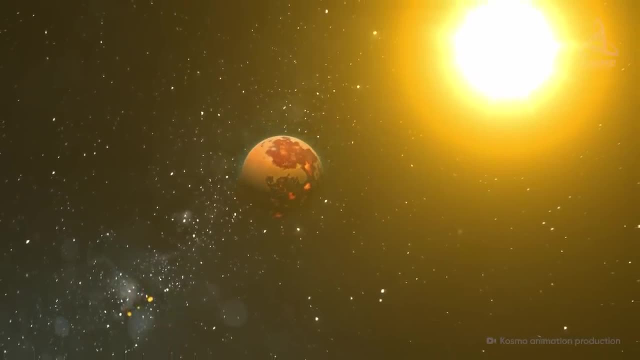 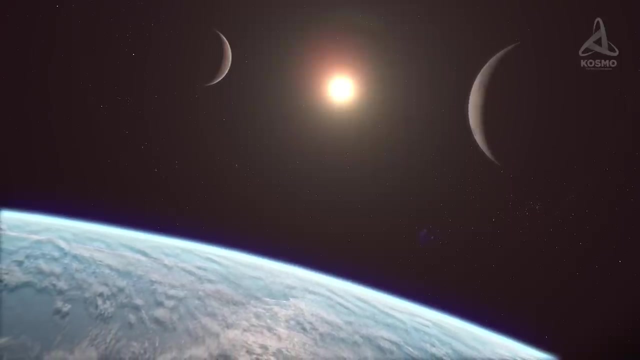 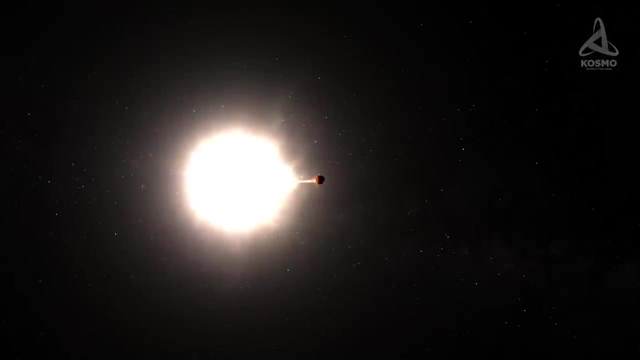 it will take more evidence to confirm that it deserves to be given it, so this remains an open question. It should be mentioned that Kepler-70b is not the only celestial object we know of that interacts with its parent star so closely. Another object in similar conditions. 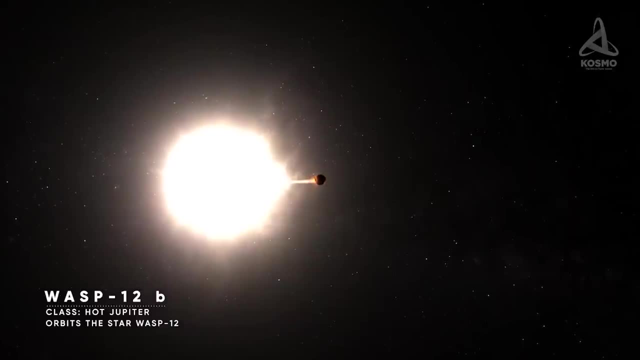 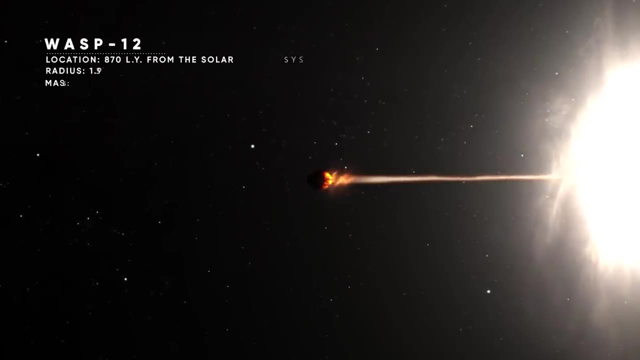 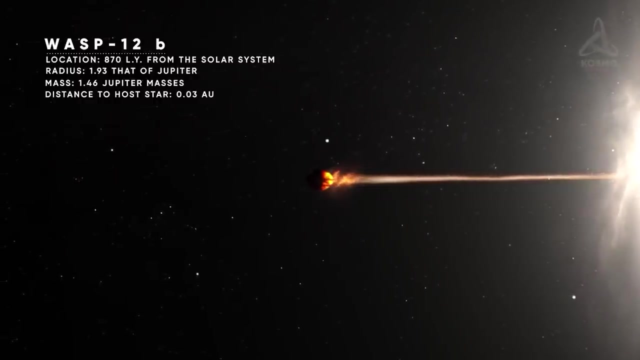 is the exoplanet known as WASP-12b. This celestial body lies 870 light-years away from our system. its radius measures 1.93 times that of Jupiter and its mass equals 1.46 Jupiter masses. WASP-12b. 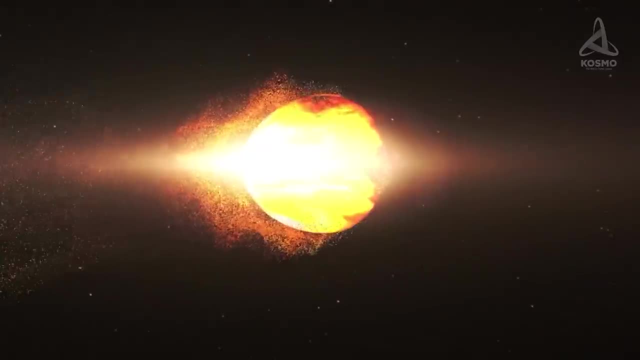 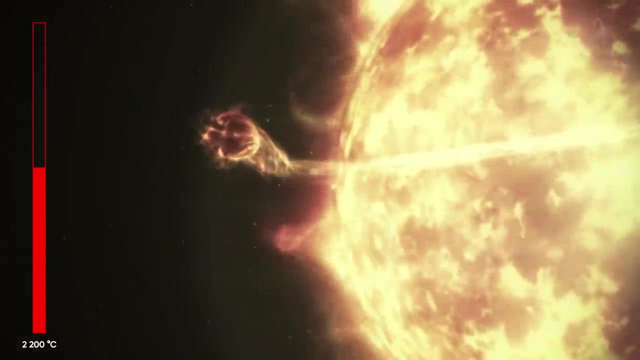 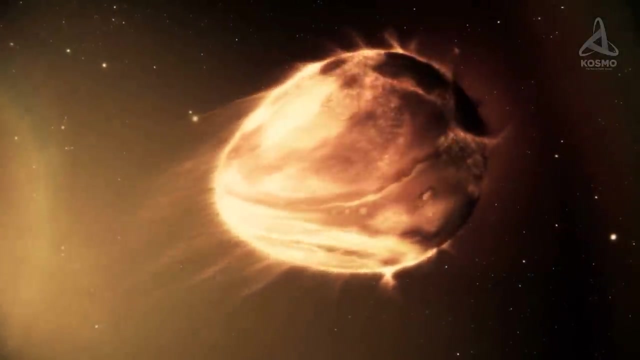 is just 0.03 astronomical units away from its parent star. Due to this close proximity, the exoplanet has a temperature reaching as much as 2,200 degrees Celsius. The host star's extremely powerful gravitation slowly absorbs WASP-12b. 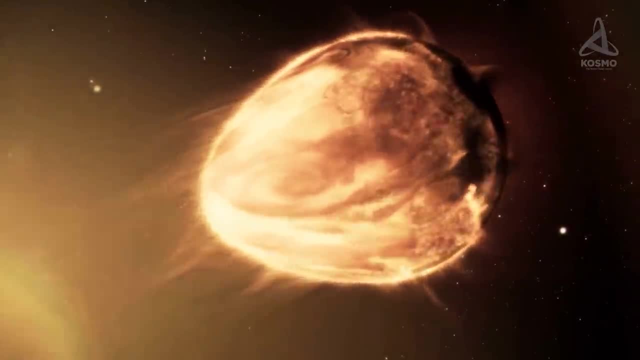 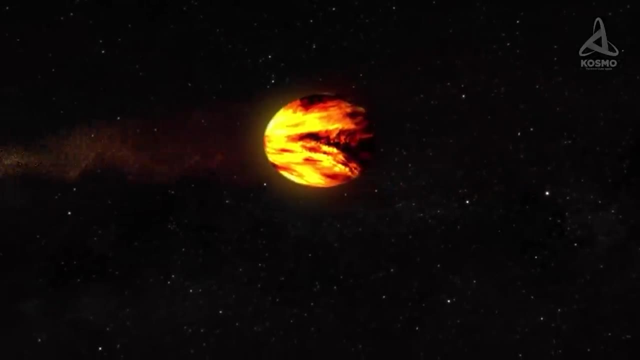 Eventually, in approximately 10 million years' time, the exoplanet is expected to be destroyed completely. Bearing all this in mind, we will probably never delve any deeper into the nature of this exoplanet. It would appear that studying worlds of this kind 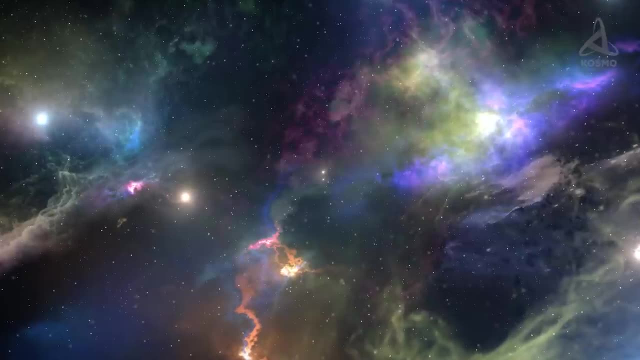 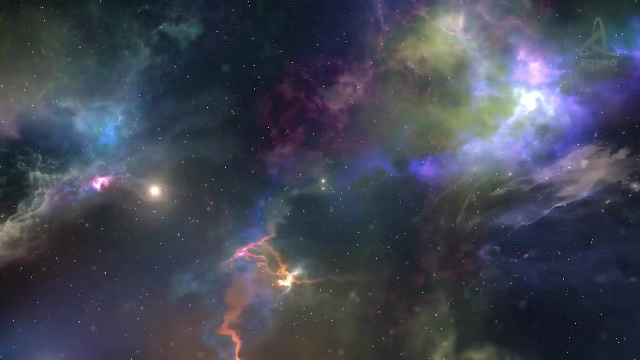 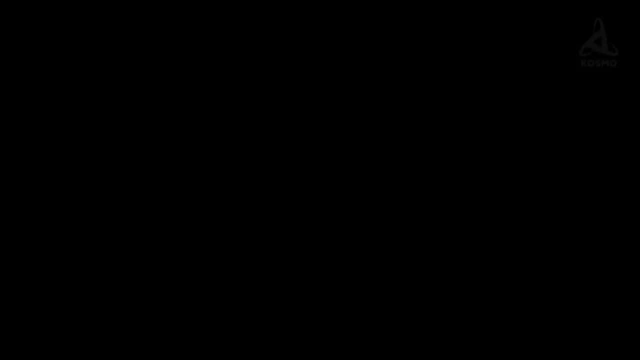 cannot be high on scientists' list of priorities. However, some of these objects may happen to have some really unique features. Seemingly quite plain and ordinary worlds like that may conceal many more dangers than would appear at first glance. When flying past the celestial body. 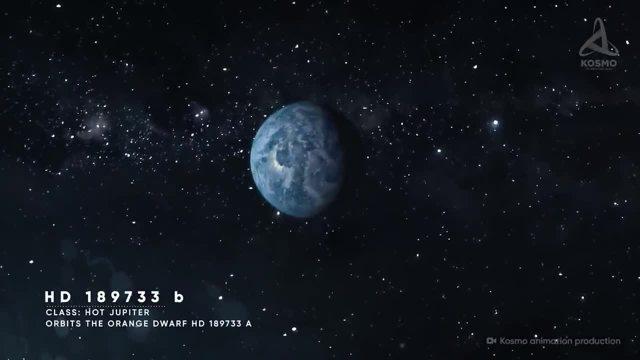 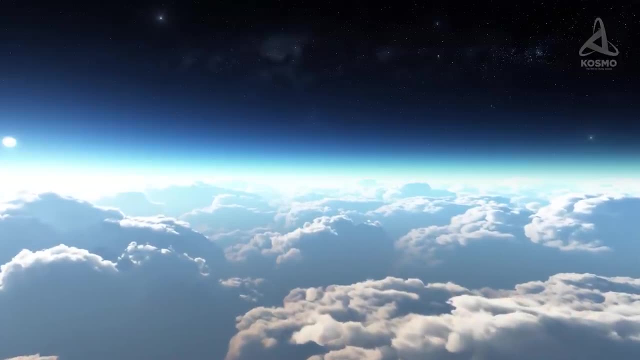 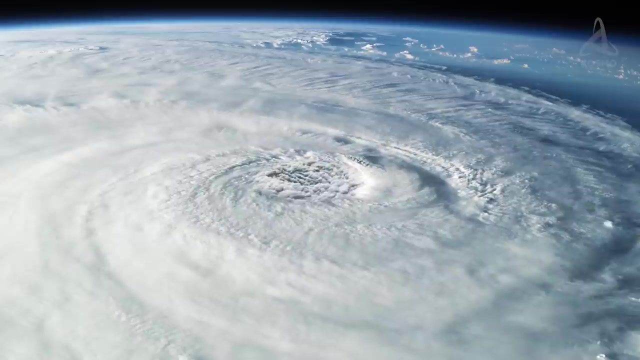 one might complacently think it a safe planet, as it resembles our Earth by its looks. But if one were to get as low as the level of its atmosphere, one would be exposed to some life-threatening dangers. For a start, the object's winds carry particles of silicate. 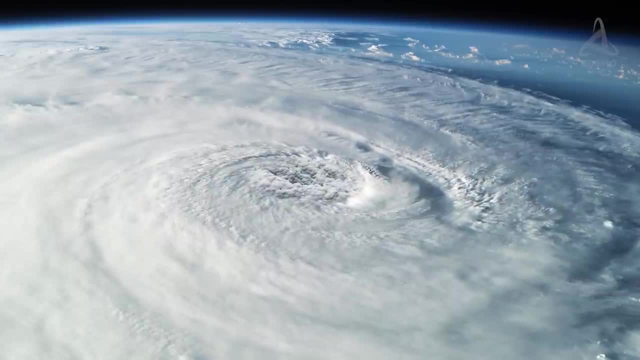 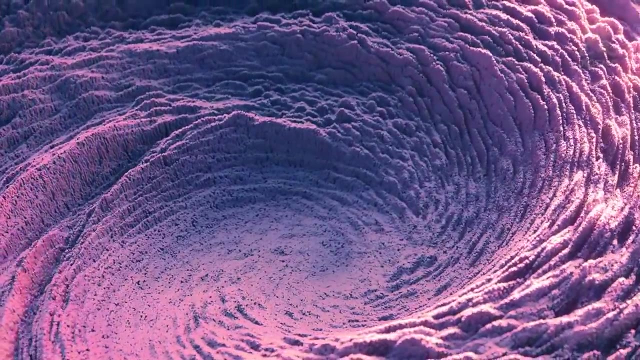 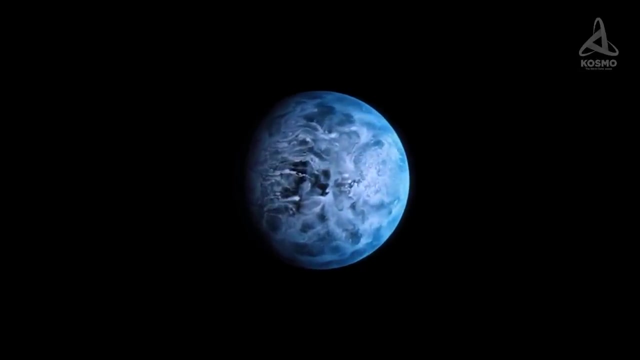 and develop velocities of 8,700 km per hour. Besides, the rains on this planet cause frequent precipitation of molten glass. The reasons for such hazardous weather conditions are extremely high temperatures and the atmosphere's peculiar chemical composition. Speaking about the exoplanet's orbital period, 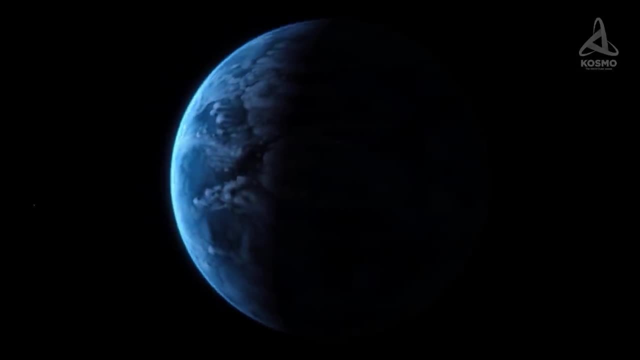 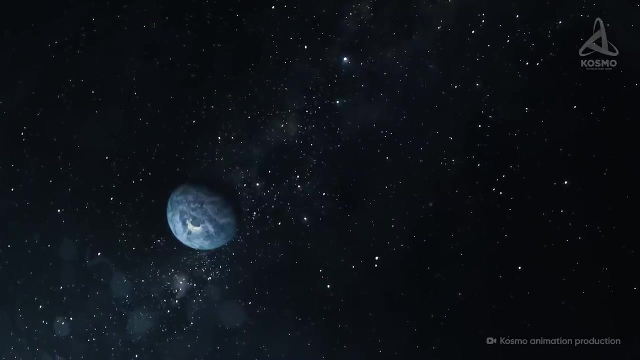 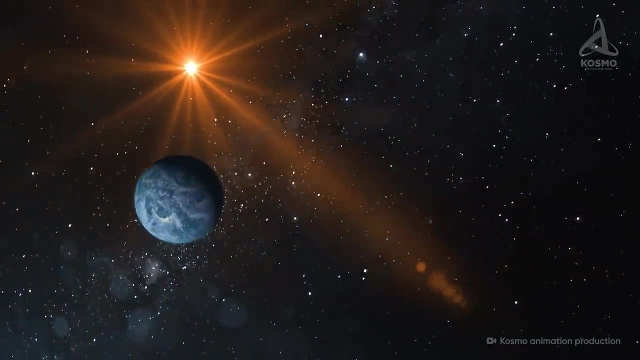 it is approximately 2.5 days and it is highly likely that the object is tidally locked to its parent star. As usual, a quick overview of its main characteristics. HD 189733 b is a bright blue gas giant orbiting an orange dwarf in the constellation Vulpecula. 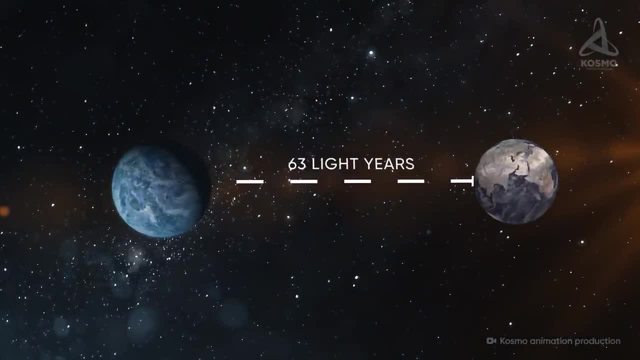 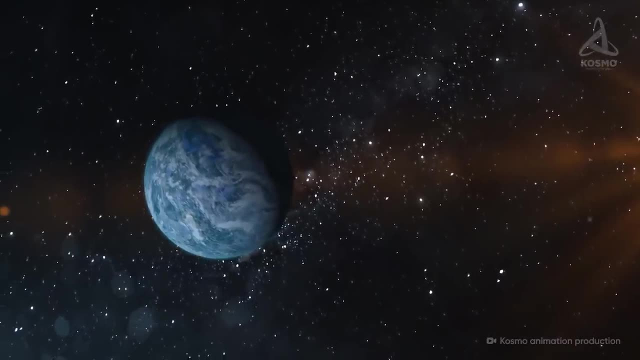 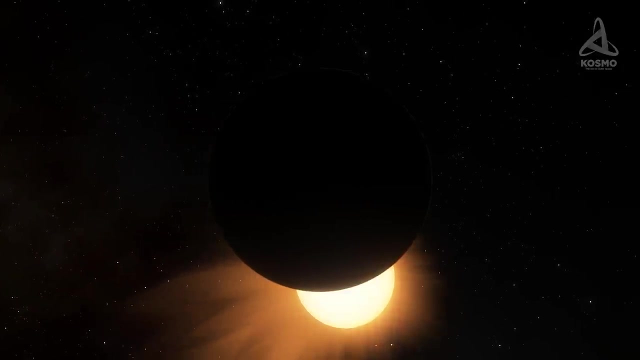 It lies just 63 light-years away from our system. The object's diameter is 1.1 times that of Jupiter and as for its mass, it is 113% that of Jupiter. Interestingly, the distance between HD 189733 b and its star. 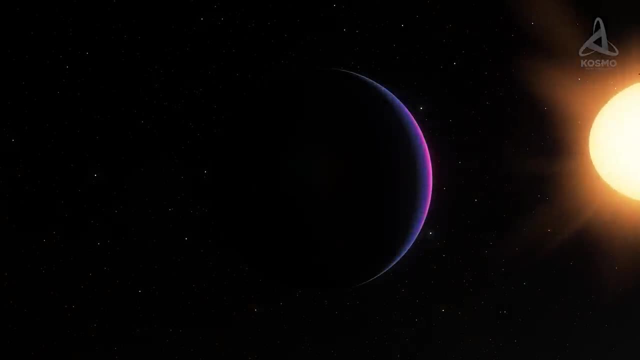 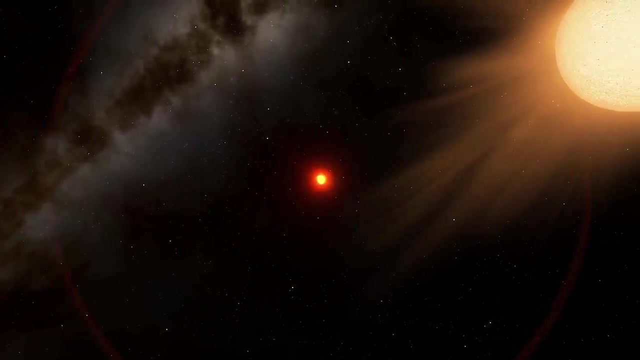 is 30 times less than the distance between the Earth and the Sun and equals approximately 5 million km. Due to its close proximity to the parent star, it has a constant surface temperature of as high as around 930 °C on the day side. 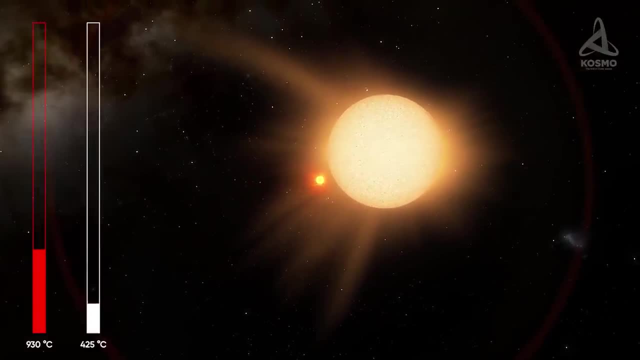 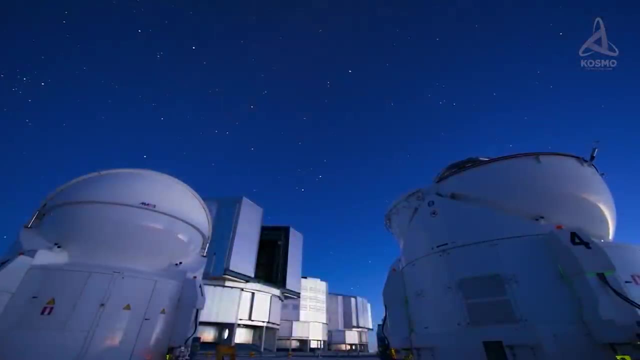 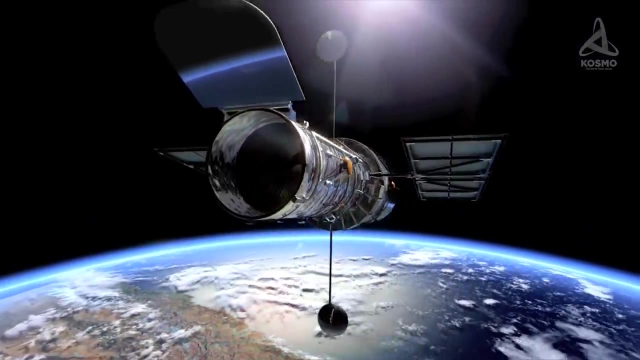 with the temperature on the night side never dropping below 425 °C. Immediately on being discovered, the celestial body became a subject of investigations in 2007,. thanks to data obtained by the Hubble telescope, scientists found out that HD 189733 b has a foggy atmosphere. 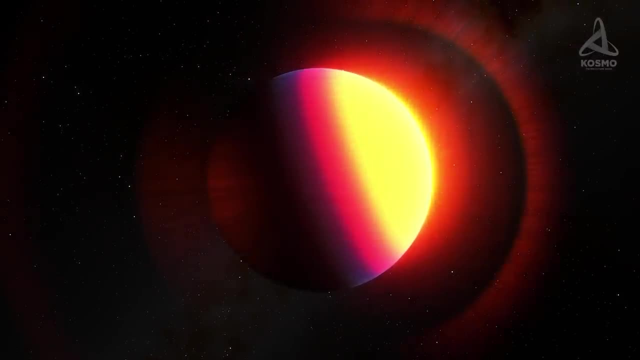 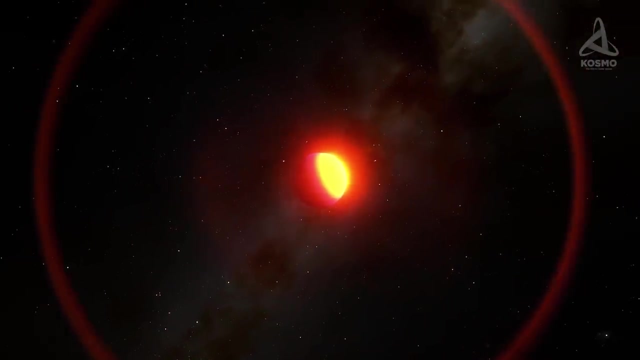 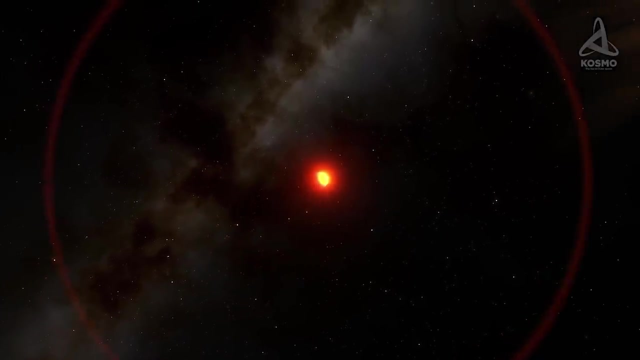 Interestingly, when the planet transits between the observer on the Earth and its star, its atmosphere assumes a reddish hue. This effect could possibly be caused by the haze in the atmosphere. According to preliminary estimates, it consists of particles of iron silicates and aluminium oxide. 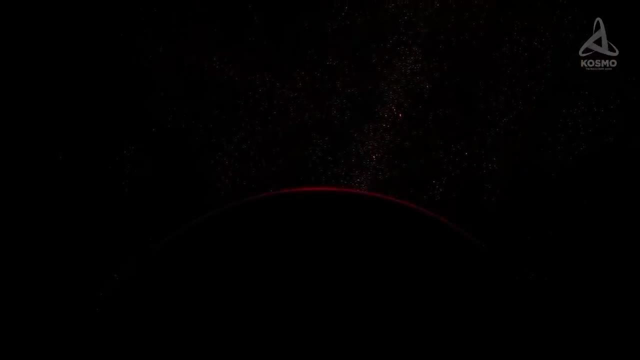 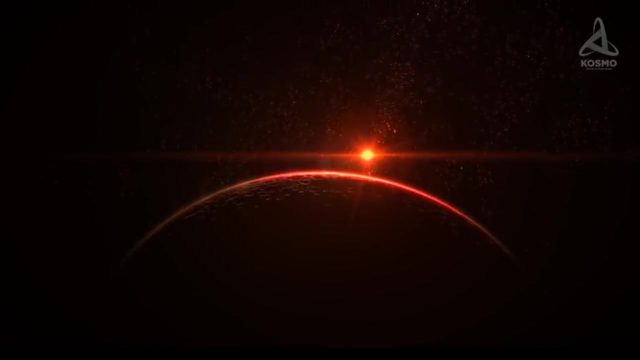 Apart from that, the information beamed back by the Hubble telescope helped scientists establish that the planet's atmosphere contains water vapour, neutral oxygen and an organic methane compound. Additional investigations revealed the presence of carbon monoxide on the day side of the planet. 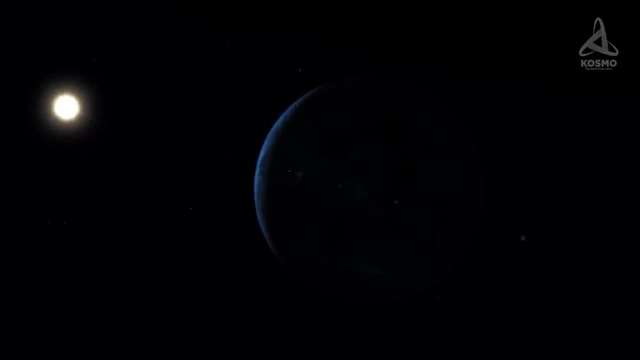 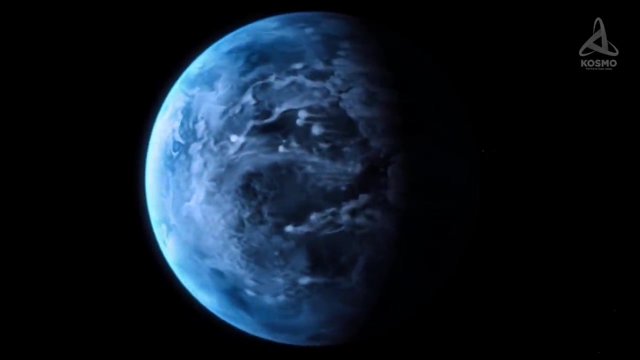 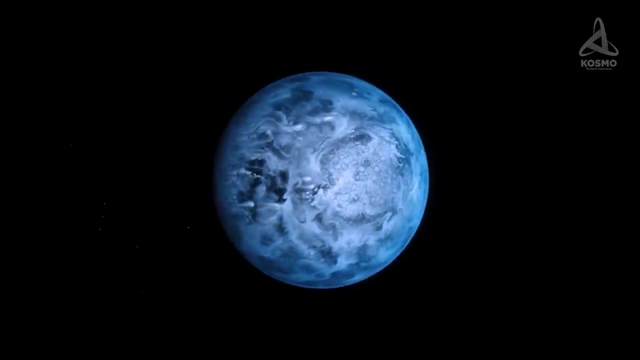 What prompted most questions, however, was the results of investigations revealing traces of methane of an unusual variety in the planet's atmosphere. This chemical element was shown to be the carbon monoxide. It is shown to be in a peculiar fluorescent state when it emits electromagnetic radiation in the infrared range. 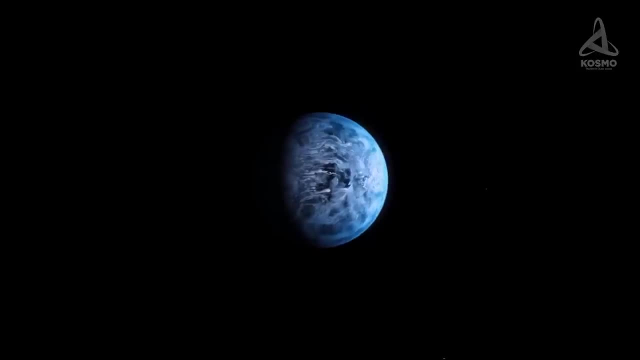 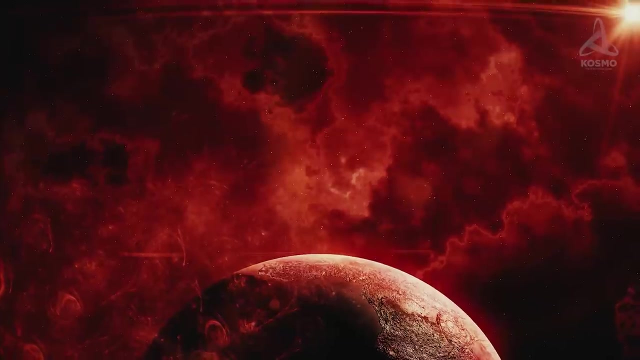 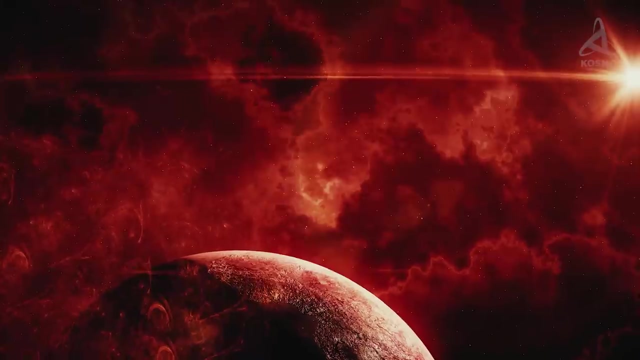 This state of the substance is indicative of some unknown activity in the atmosphere of the exoplanet, which still remains to be found out. This is quite a clear-cut example of a situation when investigating an object like an exoplanet with an exceptionally harsh environment. 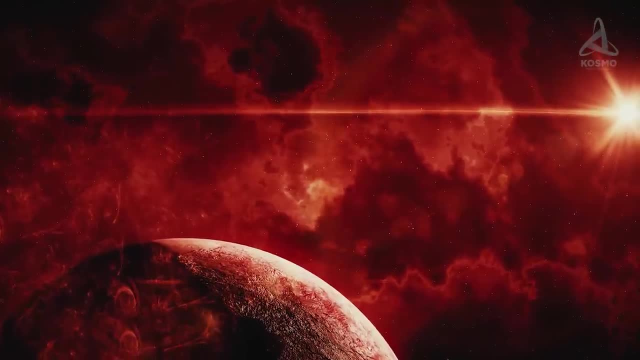 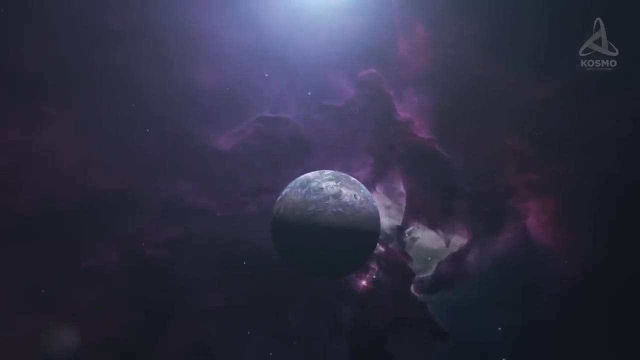 may yield unexpected results about some processes taking place there. that will be a valuable contribution to science, And, as the process of studying these worlds continues, they will remain no other than horror planets to us, as well as a solid reminder that we are more than just lucky. 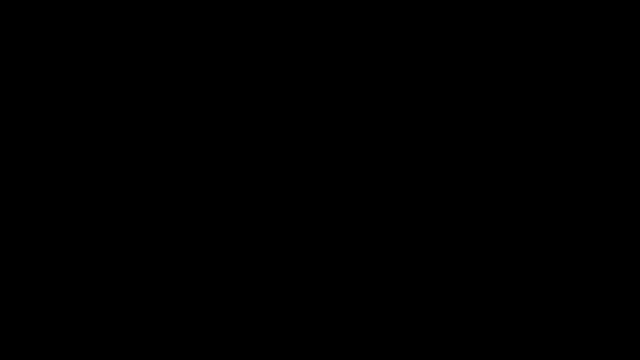 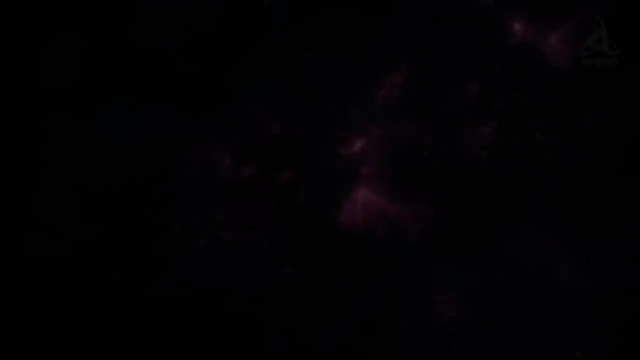 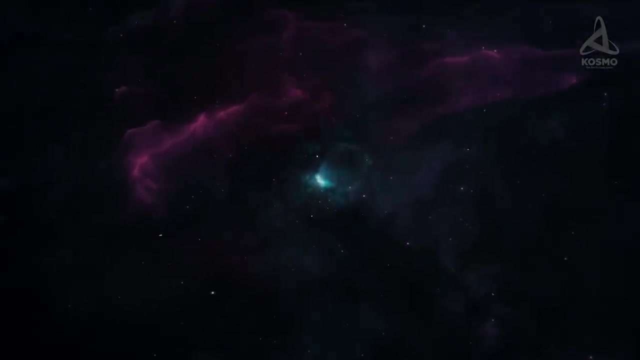 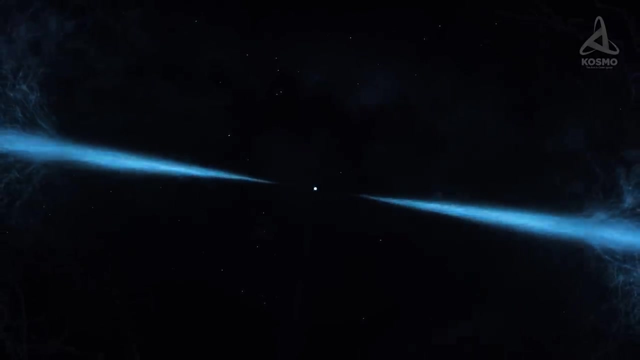 to be the dwellers of our Earth. Earlier in one of our previous videos, we have already taken a look at some terrifying and lethally dangerous worlds discovered in the vast expanses of space, With some of them extremely hot. others are located close to insanely powerful sources of radiation. 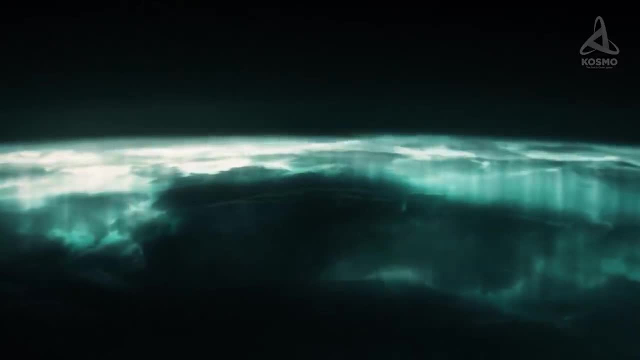 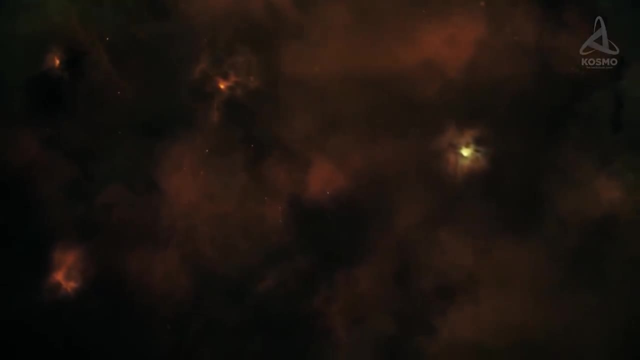 and yet other ones are peculiar for some bizarre features on their surfaces. However, we haven't quite exhausted our list of the most horrifying planets, and now it's time to see some more. Our first stop is 202 light-years away from the Earth. 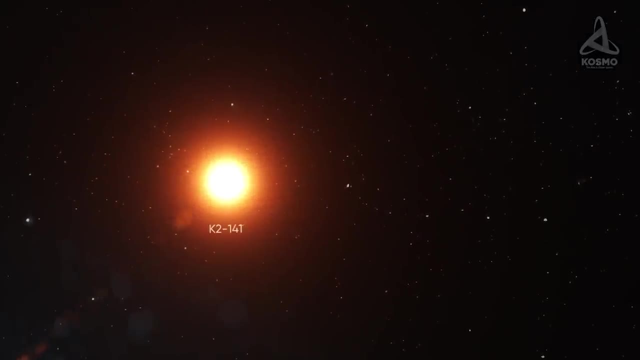 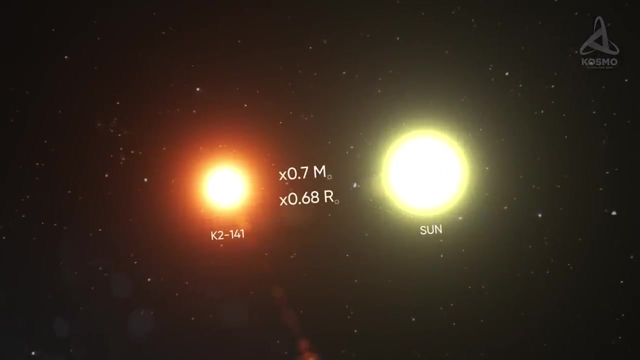 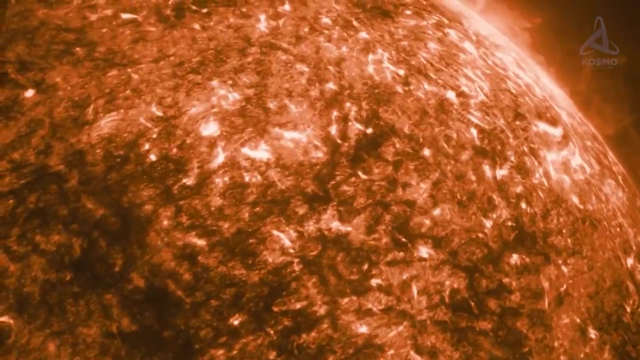 destination: K2-141,, an orange dwarf. Its mass is roughly 0.7 that of the Sun and its radius measures 68% that of our host star. With these parameters almost perfectly proportional, the star's temperature reaches 4,600 Kelvin. 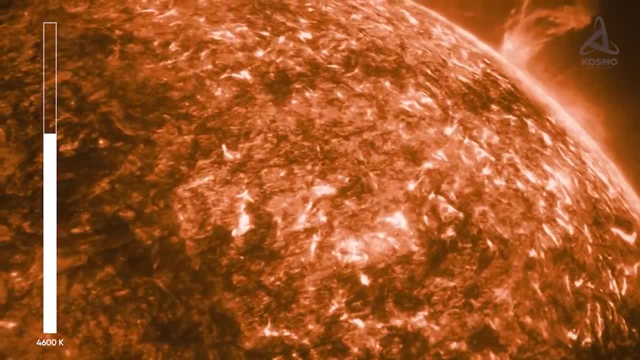 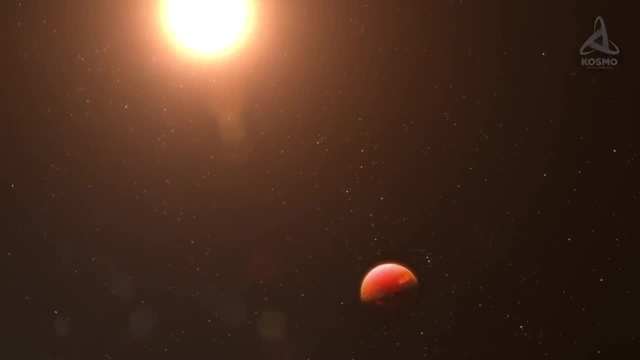 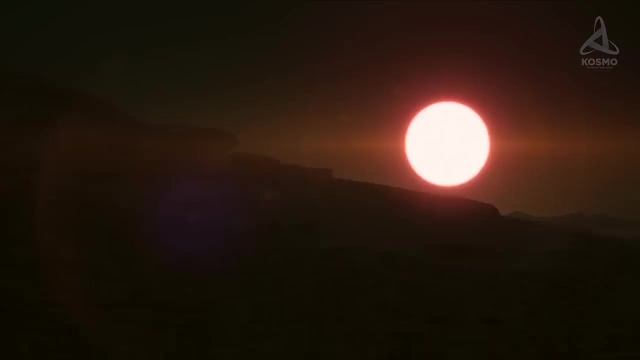 which is about 20% less than that of the Sun. And now to the planet in question. just 0.007 astronomical units away from its star, there lies a really bizarre world designation: K2-141b. This rocky exoplanet is five times as massive as the Earth. 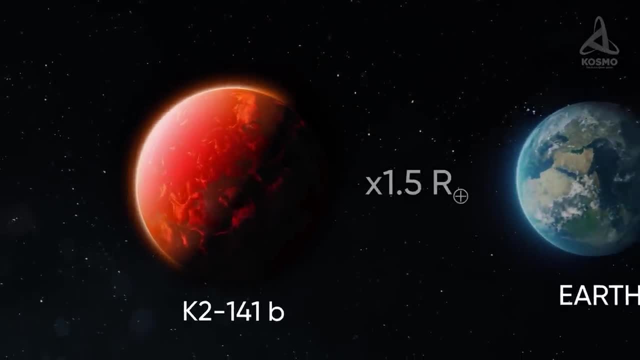 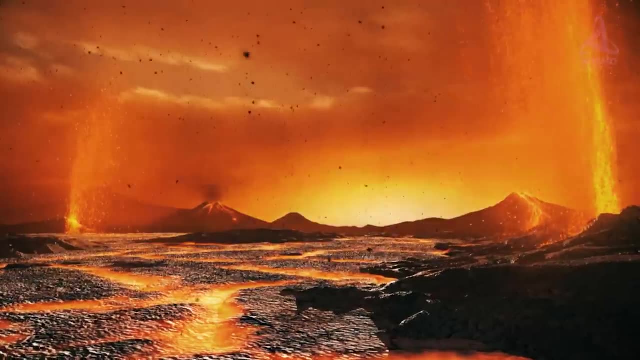 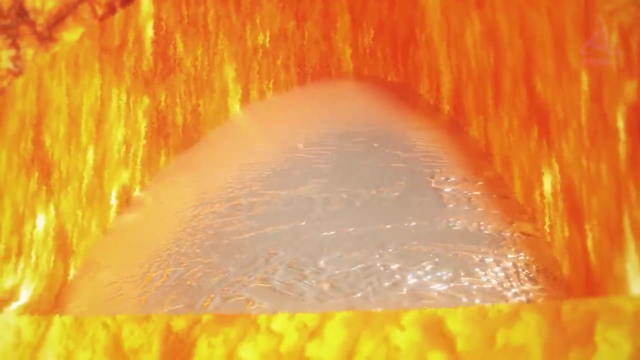 with its radius 1.5 times as big as that of our Earth. All this gives us grounds to assume that the gravity on the planet's surface is at least twice as strong as that on our planet. The heavy metallic core, meanwhile, accounts for 20 to 50% of the planet's overall mass. 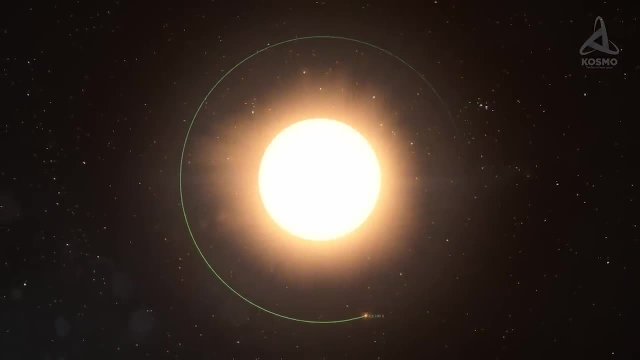 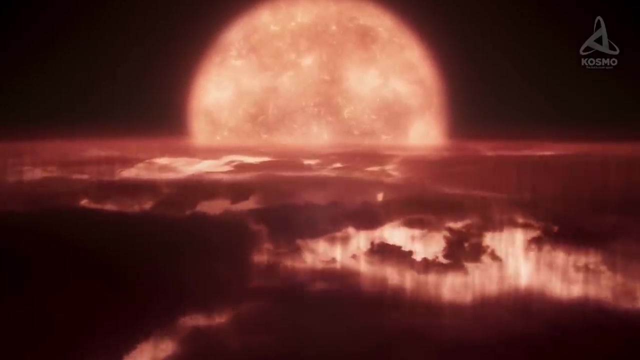 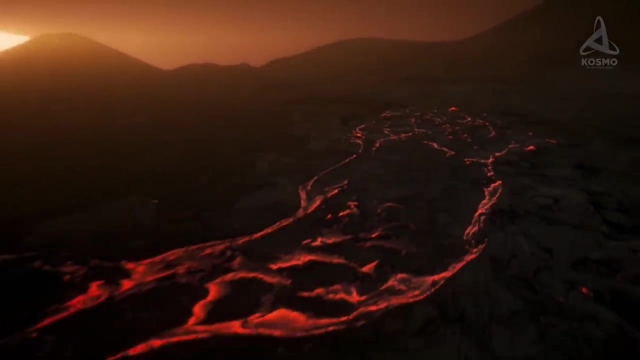 It takes the celestial body about six and a half hours to complete a full orbit around its parent star. Being extremely close, it is tidally locked to it, That is, it faces the star with one and the same side at all times. Observations show that the temperature on the planet's day side 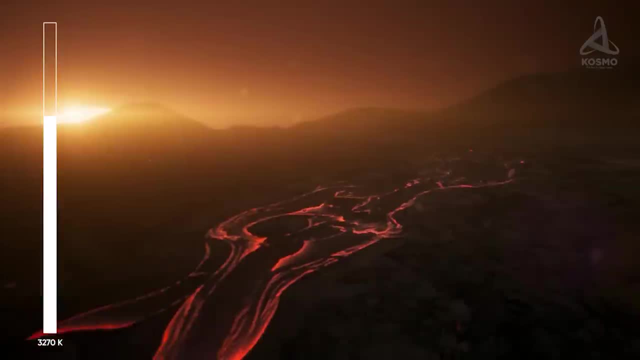 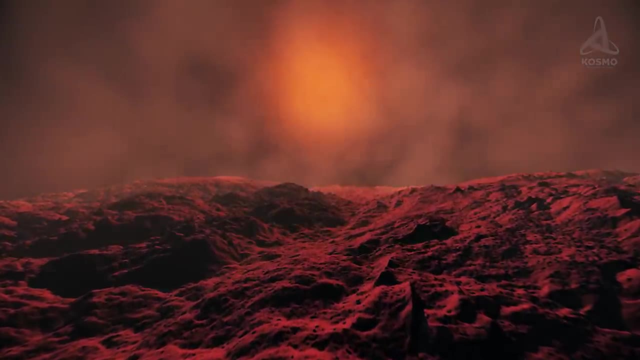 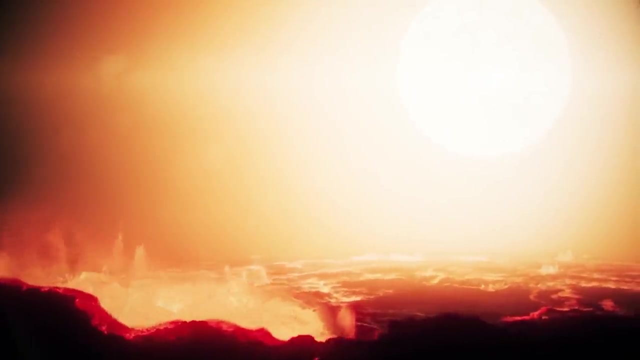 reaches 3,270 Kelvin or 3,000 degrees Celsius. This is enough not only to melt most rocks and metals, but also to effectively evaporate them. The day side of the planet is assumed to be covered with a lava ocean that never ceases to boil. 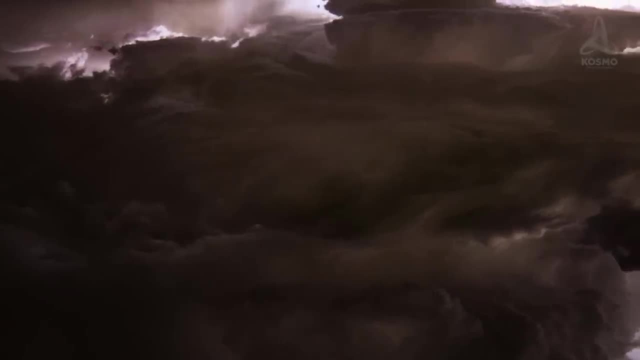 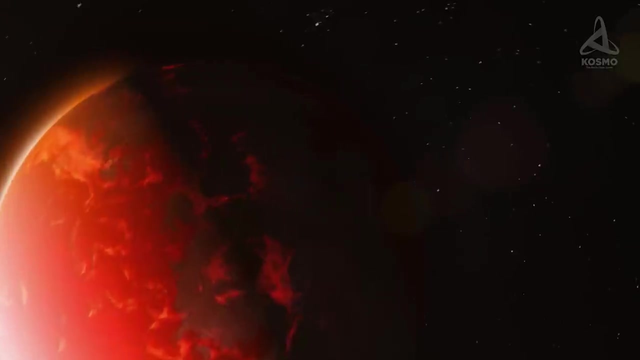 The atmosphere is thought to be rather exotic, made up of steams of heavy metals and silicates. By contrast, the planet's night side is incredibly freezing. According to estimates, the temperature of most of its area is tens of times lower than that on the day side. 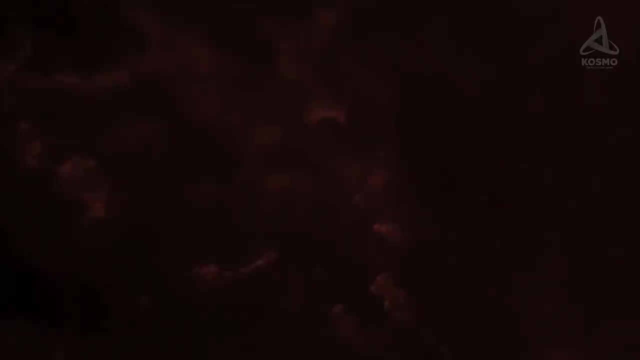 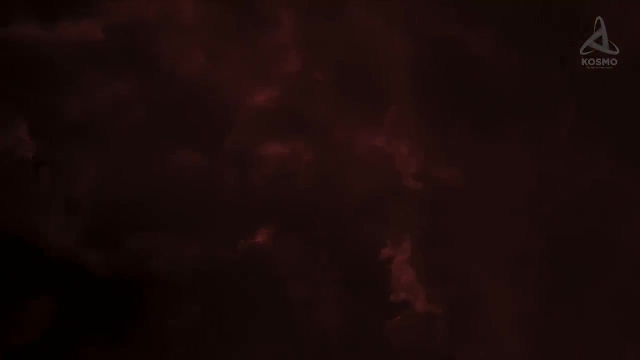 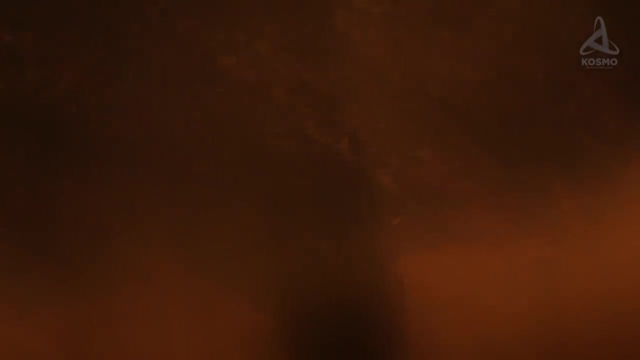 and, on balance, its values are supposed to be sub-zero. Mathematical modeling shows that this sharp temperature contrast gives rise to exceptionally strong winds whose speed reaches 1.75 kilometers per second. This is roughly five times the speed of sound, which means that the surface of K2-141b. 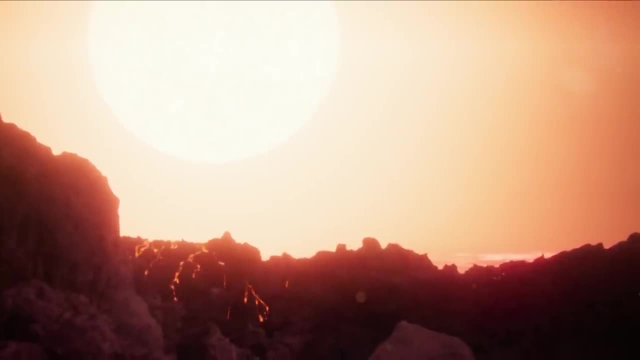 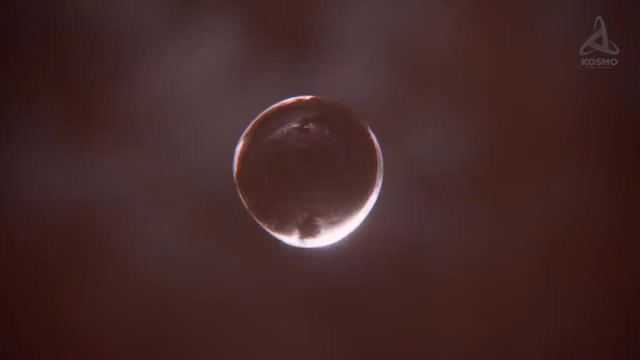 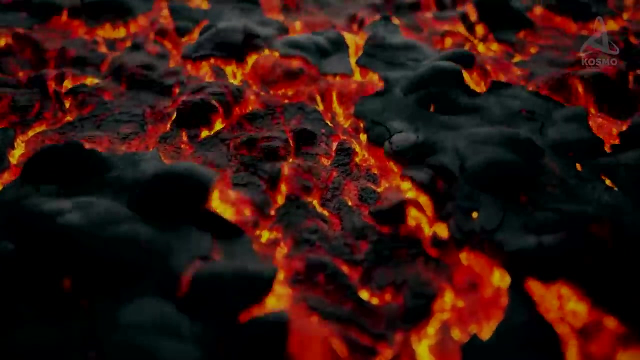 is continuously shaken by exceptionally powerful, deafening rumbling. It is assumed that on reaching the night side, atmospheric streams condense and precipitate on its surface in the form of fiery rain. This forms lava rivers and eventually this molten metal makes its way back into a magma ocean. 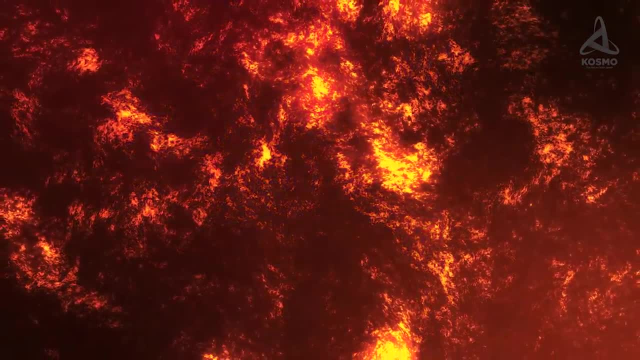 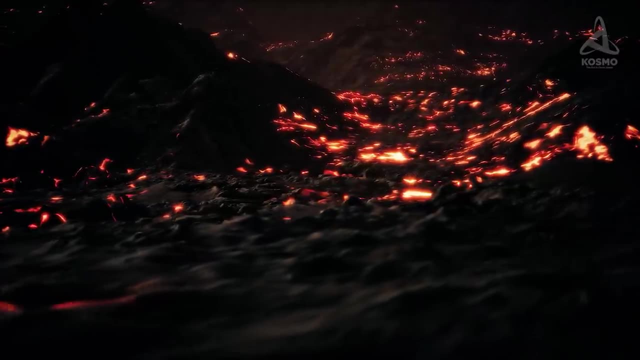 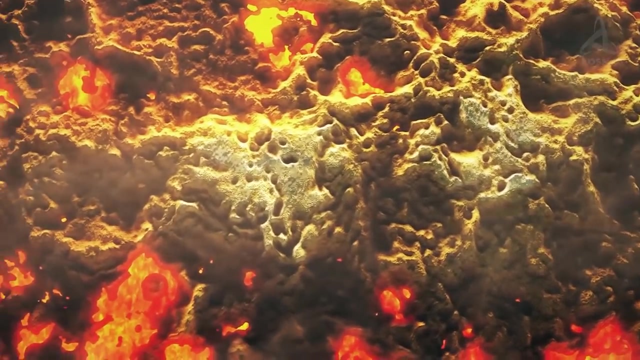 to evaporate again later on and to continue this incredible fiery circulation. However, this infernal cycle affects only a relatively small part of the planet's night side. The thing is that masses of evaporated elements from the day side simply don't make it to the main part of the night side. 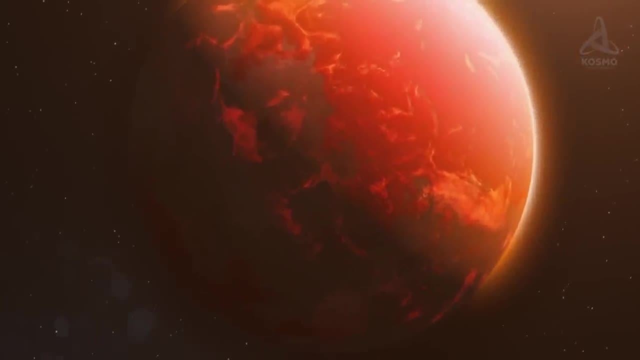 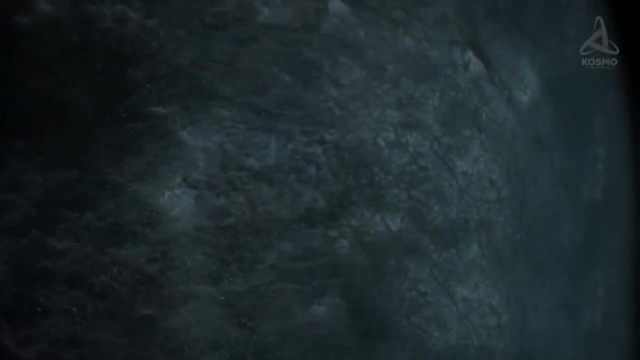 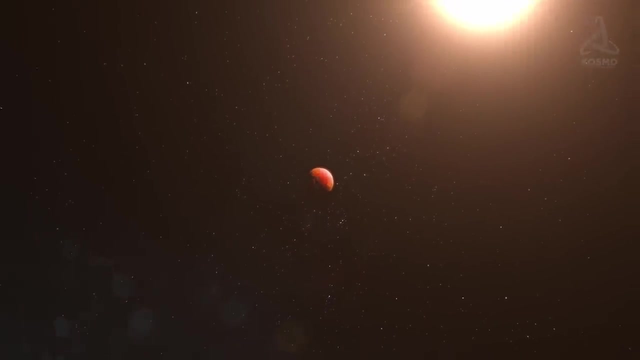 and precipitate somewhere on the border. That is why the central part of the night side is likely to be a freezing desert bound with layers of solid rocks. Remarkably, K2-141b is far from being the hottest planet that we know of. 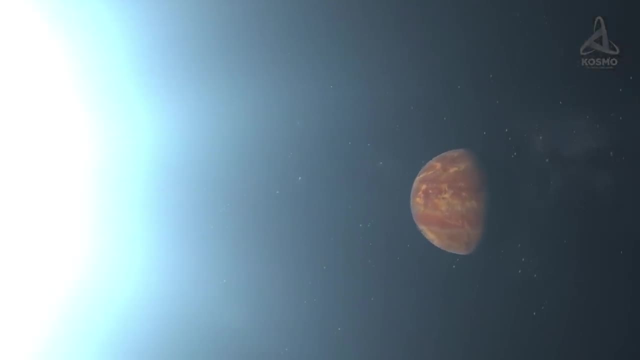 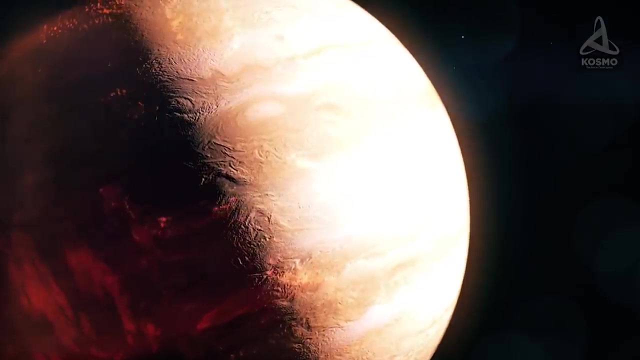 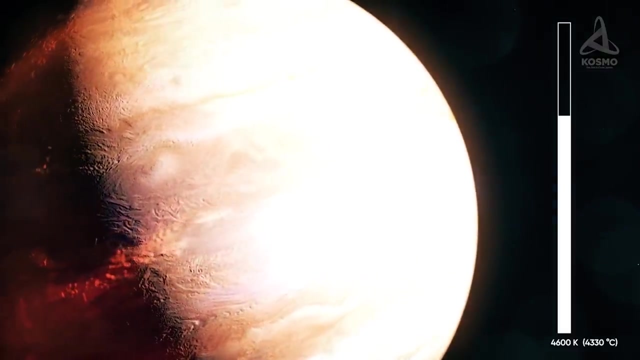 For example, there is an object referred to as KELT-9b lying 670 light-years away from the Earth. Its surface is as hot as 4,600 Kelvin, which is approximately 4,330 degrees Celsius. Just to compare, 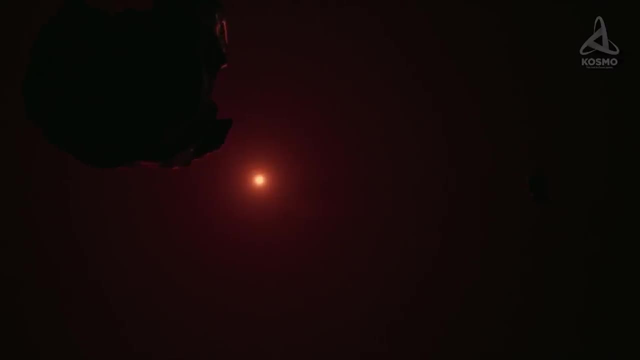 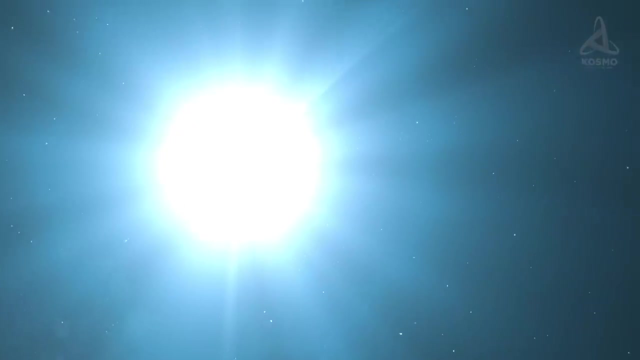 the outer layers of almost all red dwarfs, for example, are much cooler, which means that, in terms of temperature, this exoplanet is quite a match to stars. Its parent star designation, KELT-9,, is of a whitish-blue color. 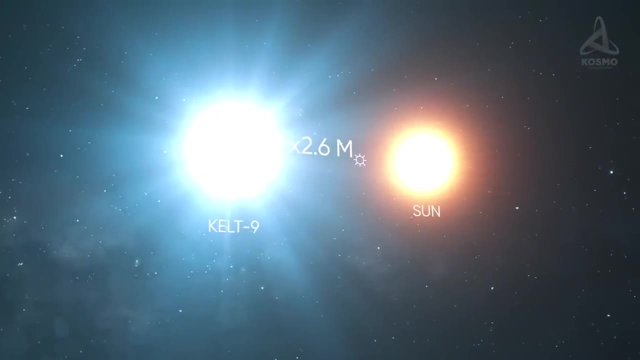 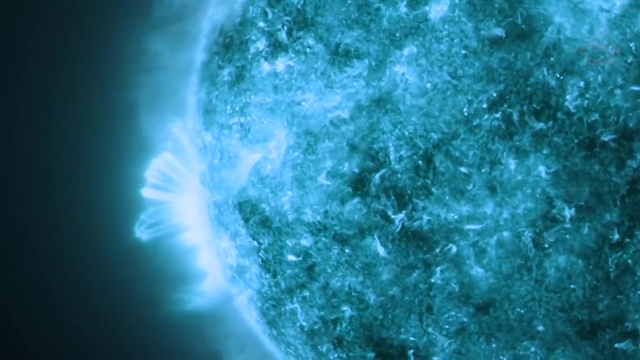 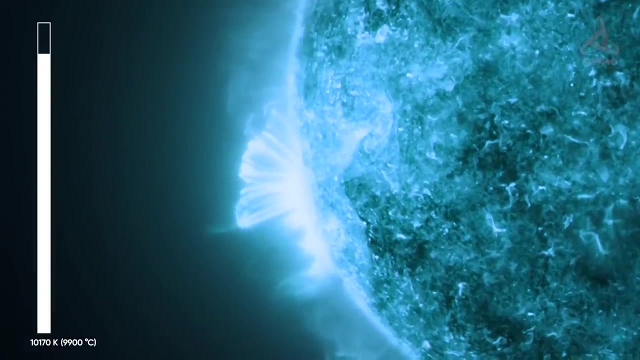 and has a mass 2.6 times that of the Sun. As for its diameter, it is 2.3 times that of our star. The surface temperature of KELT-9 is rather high, at approximately 10,170 Kelvin, or a staggering 9,900 degrees Celsius. 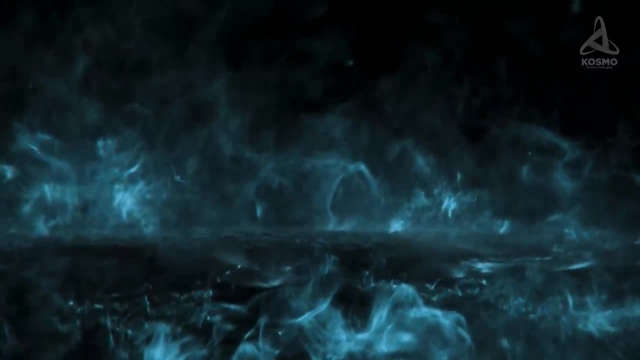 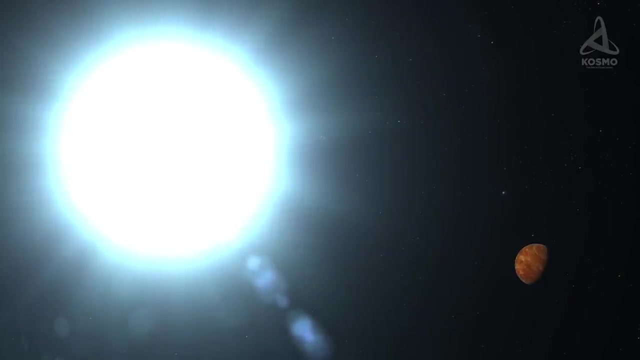 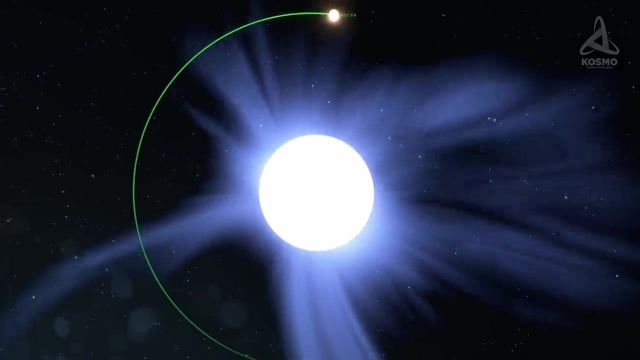 This largely accounts for the extreme conditions on KELT-9b, which lies quite close, by Just 0.035 astronomical units away from its parent star. the planet completes a full orbit around its system's center roughly every one and a half days. 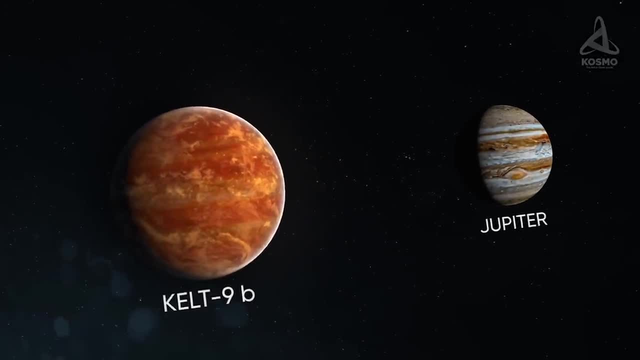 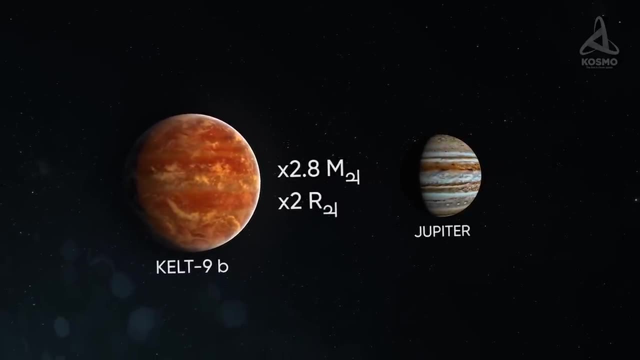 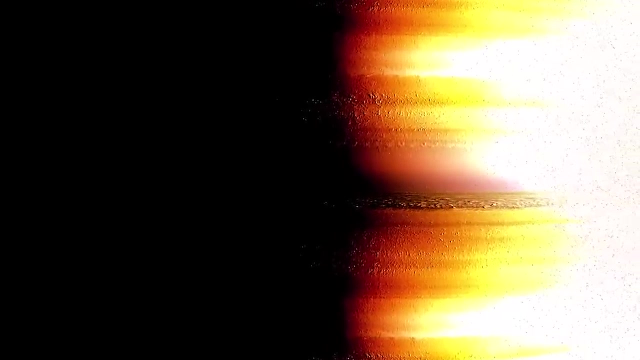 KELT-9b is a hot gas giant. Compared to Jupiter, its mass is 2.8 times as big and its radius measures roughly twice as much as that of the largest planet in our system. Based on today's notions about the composition of this type of planets, 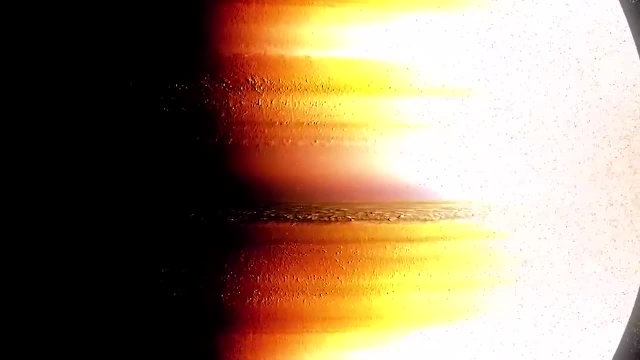 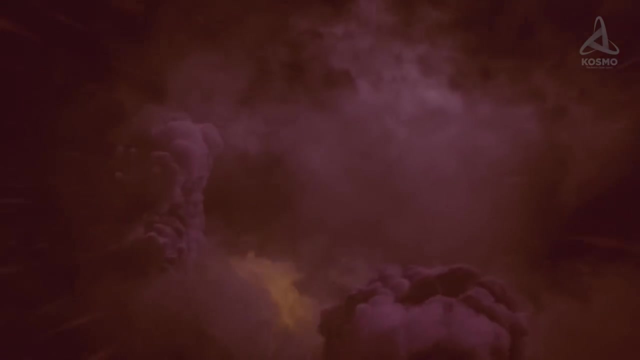 the inner part of KELT-9b's atmosphere is supposed to be even hotter. Estimates allow for this value to reach as much as 11,000 Kelvin on account of heavy metal ionization. With this figure so exceptionally big, it appears that the planet's atmosphere should contain vaporized iron and titanium. alongside the elements we are used to in an atmosphere's composition, such as hydrogen or helium, Its close proximity to the parent star and the extremely high temperature cause the planet to gradually lose its atmosphere By and by a powerful stellar wind blows it off into space. 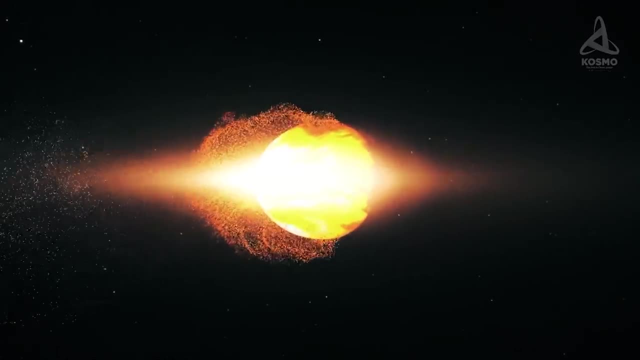 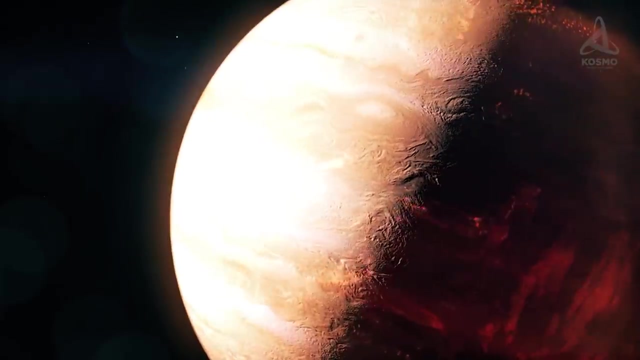 which is why the object is shrouded in a cloud of rarefied gas. This material will eventually be attracted and absorbed by the star. Interestingly, according to some estimates, the exoplanet loses up to 68 Earth masses every billion years. 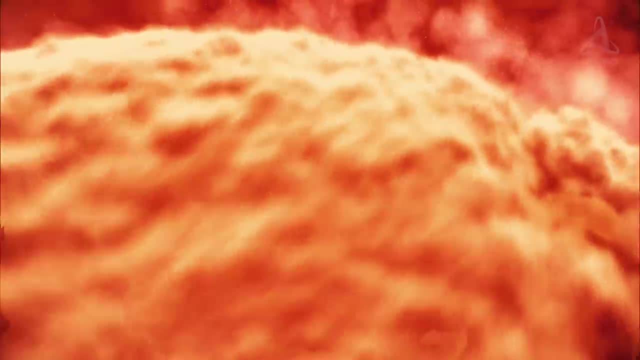 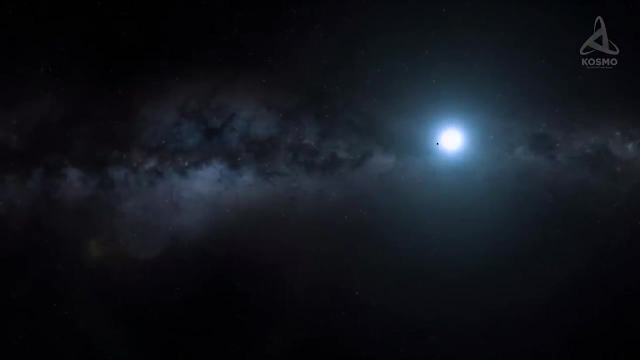 Theoretically, in a long while, KELT-9b may well get stripped of all of its atmosphere and transform itself into a Thonian planet. However, its parent star is likely to hit the final stage of its life cycle long before that. 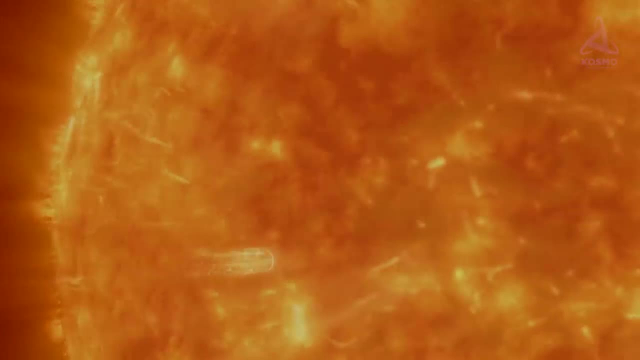 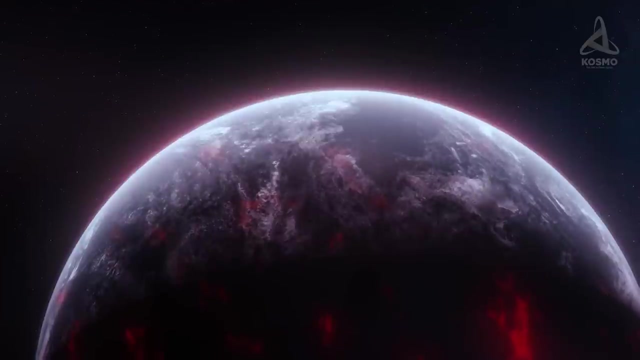 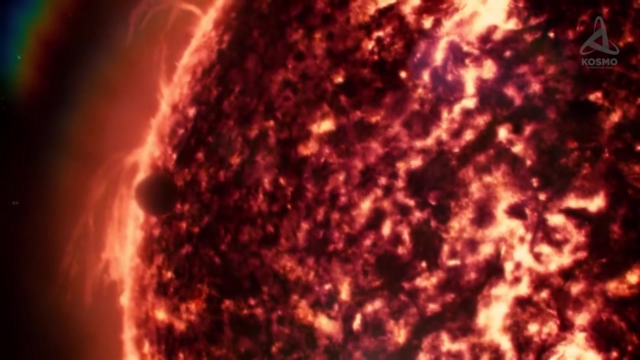 swallowing up and destroying all the celestial objects within its reach. The space objects we have just looked at are a living proof, as it were, of the fact that stars can destroy the planets close to them and not just warm them up. But, incidentally, there are celestial objects out there in the Universe. 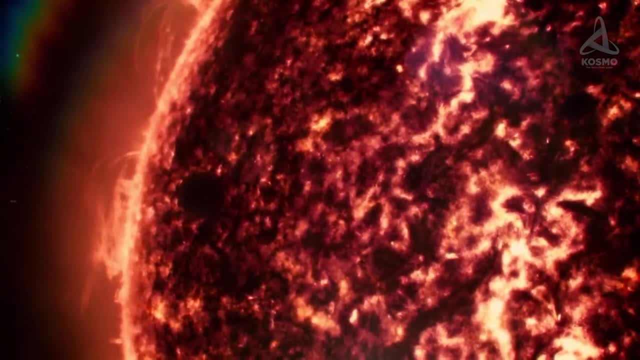 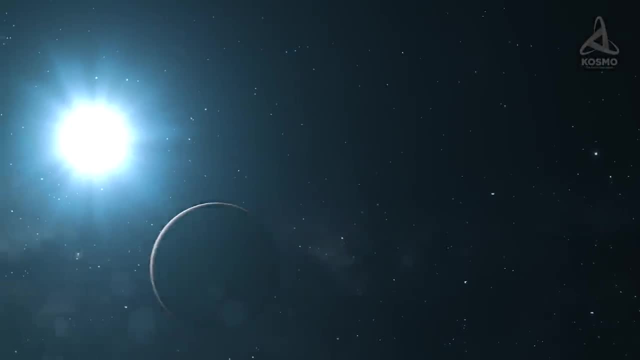 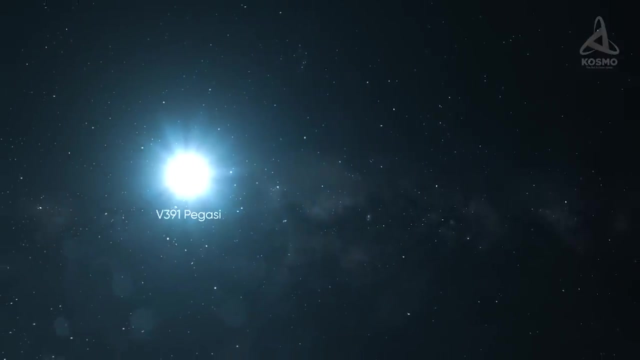 that have experienced their parent star's wrath in full measure. One of such objects lies 4570 light-years away from the Earth, in the environs of a small star designation V391 Pegasi. Now, this star is a white dwarf whose mass is twice as little as that of the Sun. 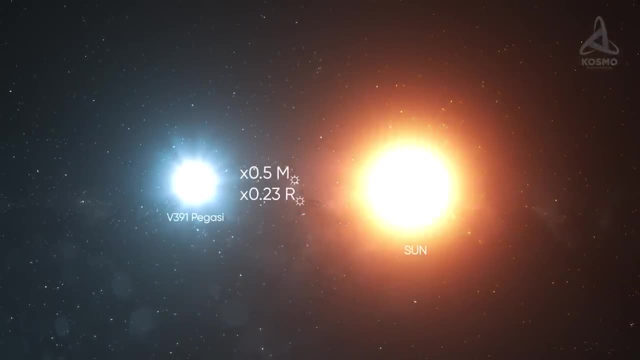 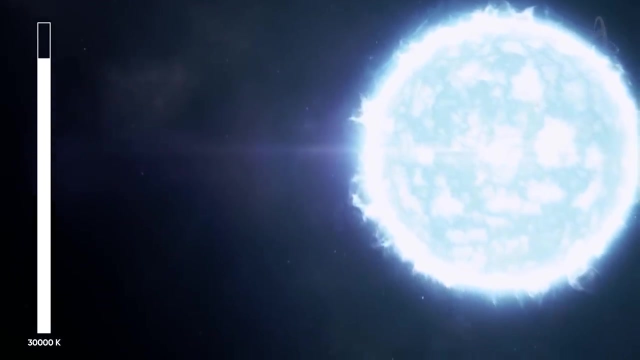 and whose radius is approximately 23% that of our parent star. The temperature of this celestial object is unbelievably high, at almost 30,000 Kelvin. All thermonuclear energy and all thermonuclear reactions in its interior would have run their course a long while ago. 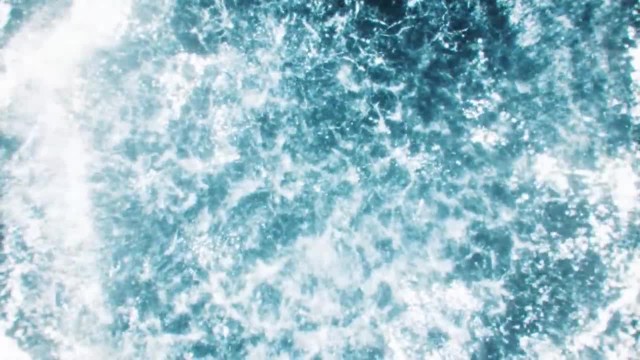 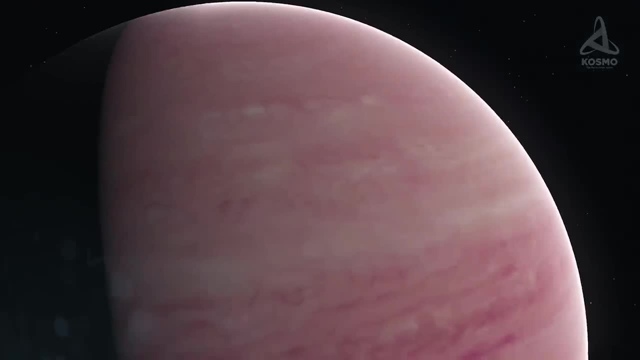 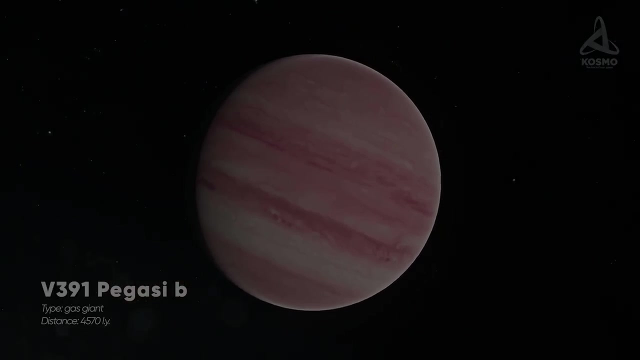 Up ahead are hundreds of billions of years of slow cooling, with the white dwarf eventually transforming into a black one. The planet we will look at, referred to as V391 Pegasi b, is in this ordinary star's environs. Its lot is exceptionally amazing. 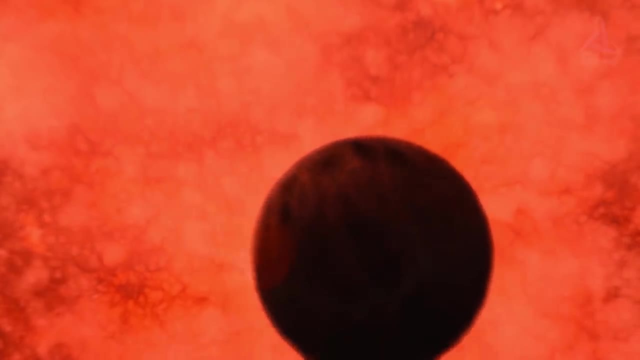 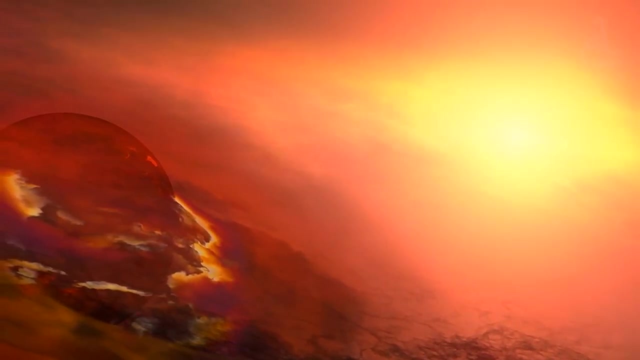 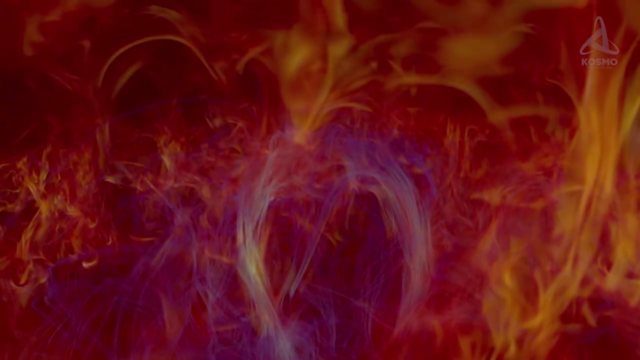 According to mathematical modeling, the planet not only survived its progenitor star shedding its outer layers, but actually found itself almost within this star for some time. It is assumed that when the system's star V391 Pegasi transformed into a red giant, its outer layers extremely rarefied by then. 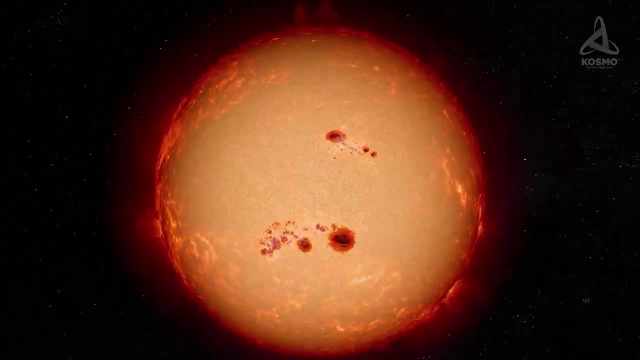 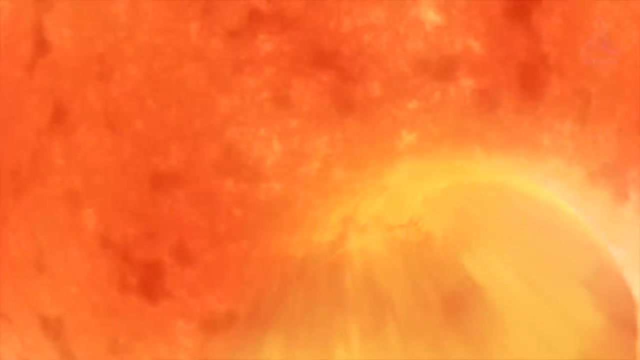 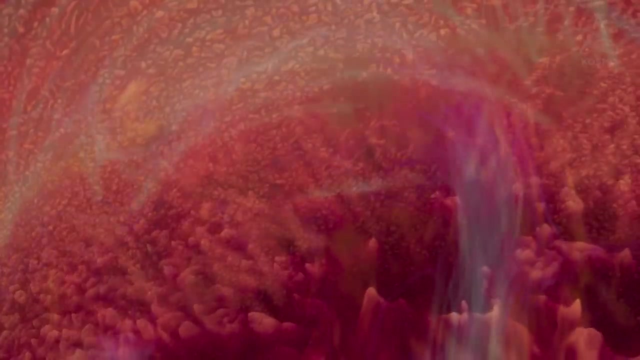 were almost brushing the planet's orbit. Their density became dozens of times lower than the atmospheric air were used to, which means that the celestial objects devoured by the dying star remained whole for a while and didn't get destroyed at once. It goes without saying that they would have been losing their speed. 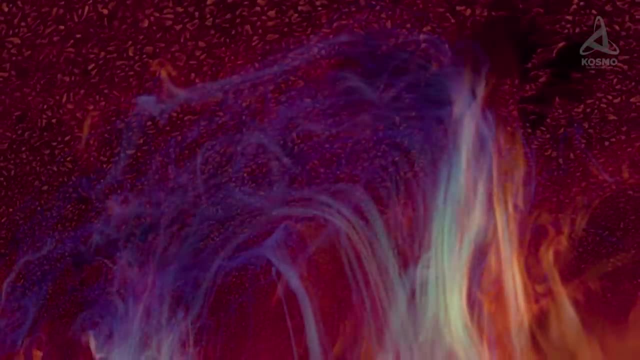 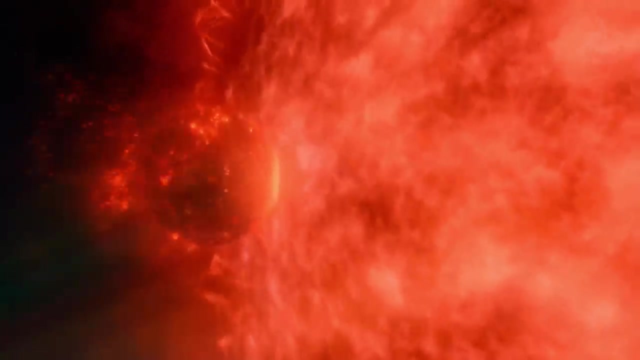 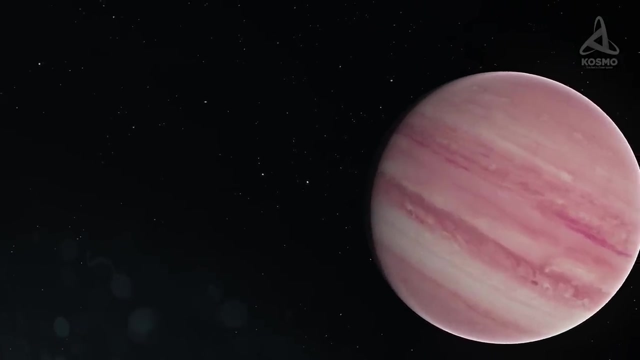 and dropped into the star's hotter and denser layers. Still, V391 Pegasi shed its outer layers sooner than V391 Pegasi b, melted and ceased to exist as a whole object. At the moment, the exoplanet appears to be a gas giant. 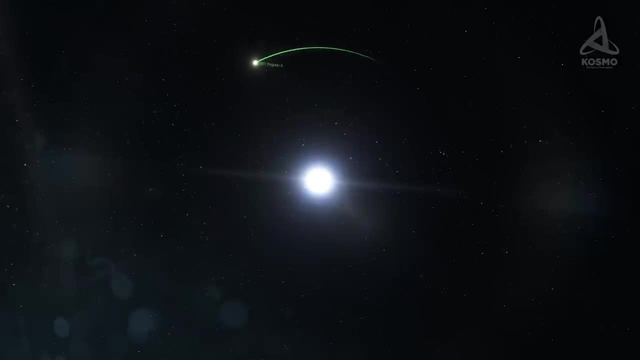 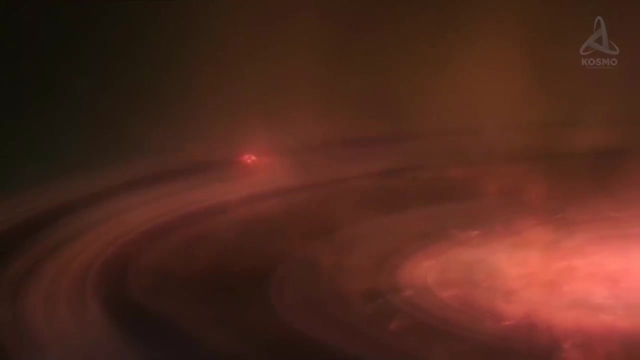 three times as massive as Jupiter. Its orbit passes 1.7 astronomical units away from its parent star, and it takes the planet approximately 1170 Earth days to complete a full orbit around its system center. It is still not entirely clear how this astronomical body managed to preserve such a big mass. 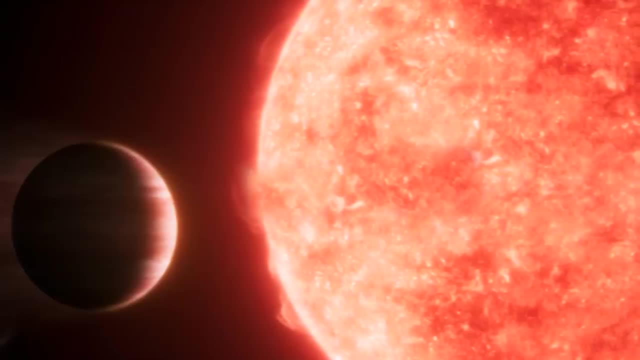 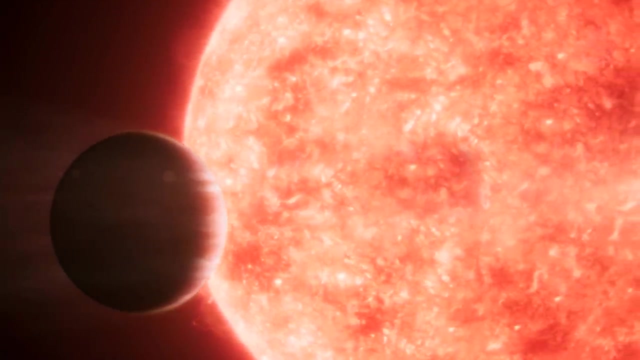 after its collision with the scorching hot layers of the star. Their influence was supposed to have destroyed the object's atmosphere completely. However, there is no doubt that the host star's collapse brought about some dramatic changes, both in terms of the exoplanet's orbit. 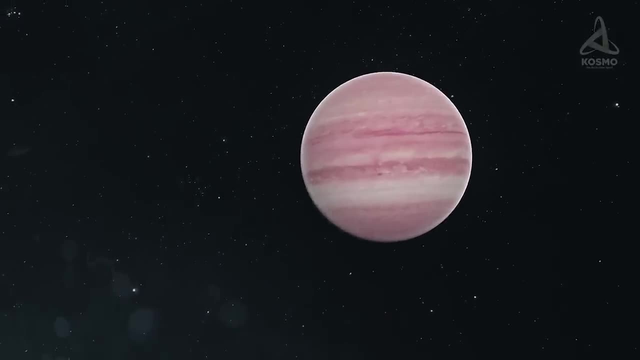 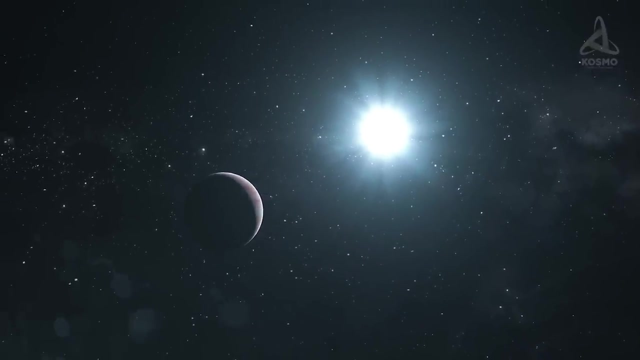 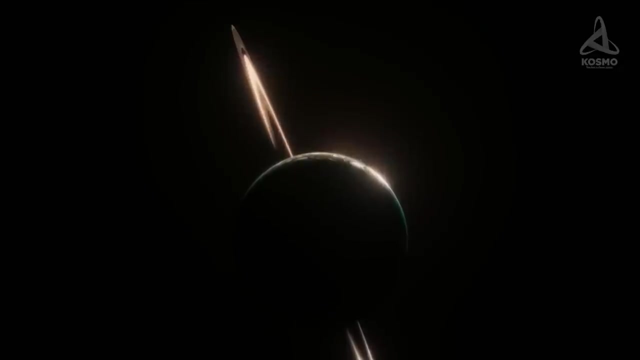 and its parameters. That is why it is hardly possible for us to ever find out what V391 Pegasi b was like before immersing in a sea of raging plasma. Space expanses can seal uncountable astronomical objects with the most bizarre properties. 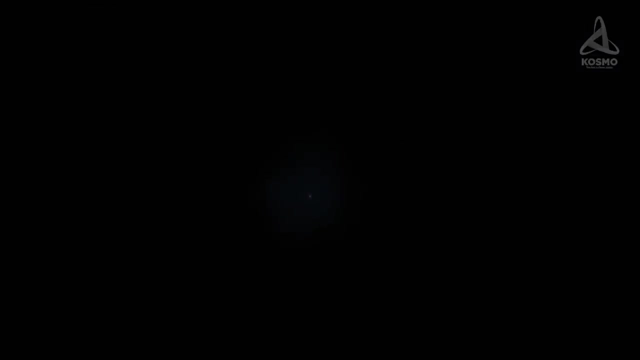 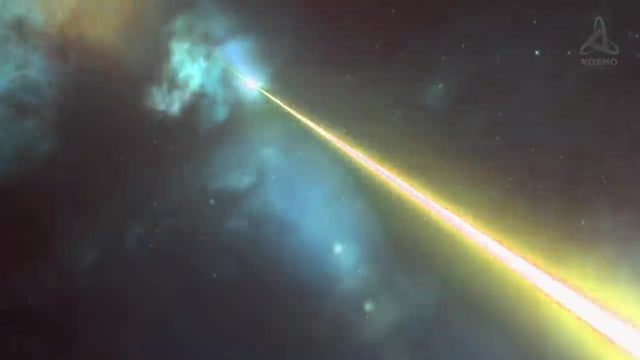 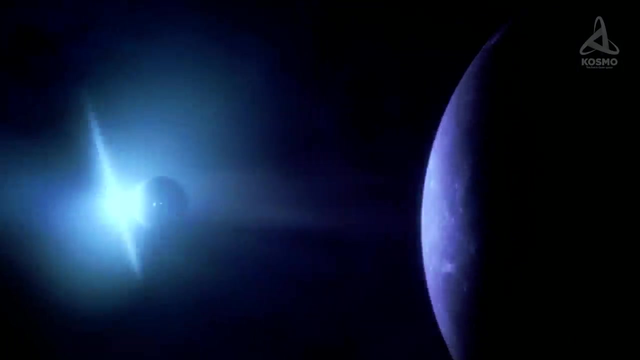 Some of them are almost totally invisible through regular telescopes, but can be detected by looking at radio wavelengths when exploring space. An example of such like celestial objects is pulsars, neutron stars spinning on their axes at a mind-boggling speed. These object spectra are peculiar. 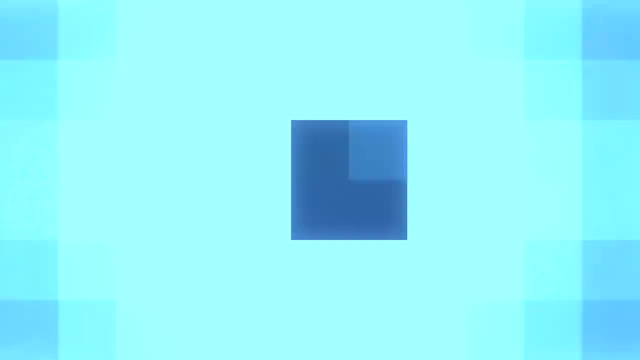 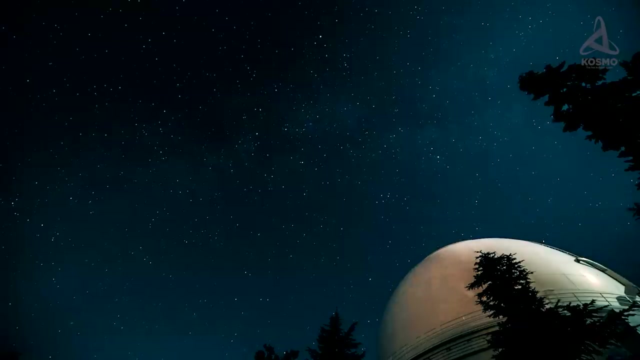 for exceptionally fast and regular pulsations. That is why it is quite easy to detect another celestial body transiting between a radiation source like that and an observer on the Earth. This is precisely the way our next object of interest was discovered, But first we'll be looking at a pulsar. which lies around 4000 light-years away from the Earth. This neutron star boasts quite a long name. Here it is on the screen, And now let's check out its remarkable features. The pulsar's diameter is just a measly 20 km. 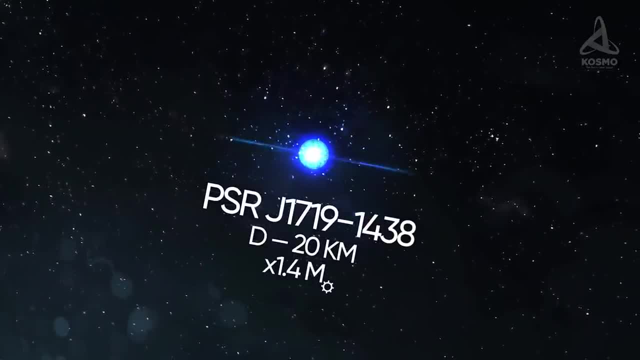 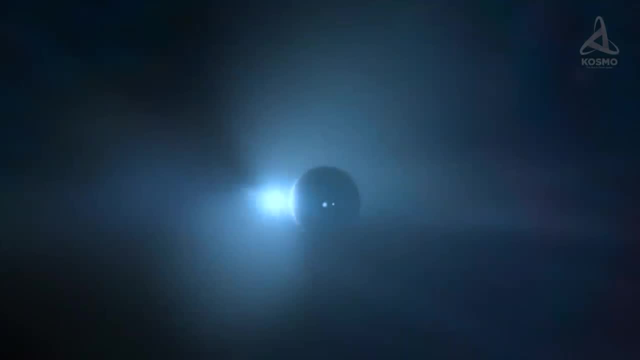 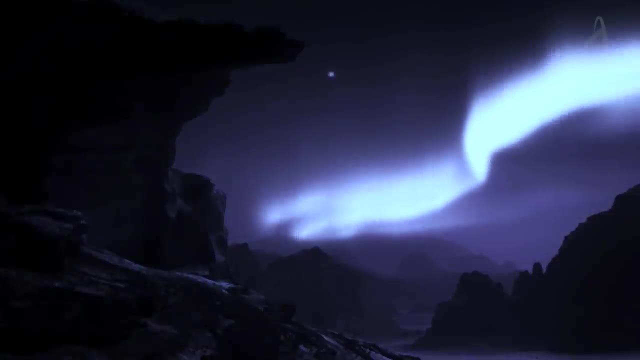 and its mass is approximately 1.4 that of the Sun. The object spins at an incredible rate, with roughly 10,000 rotations a minute, while continuously emitting powerful electromagnetic radiation impulses. Now the surface of the Earth, the exoplanet, our next object of interest. 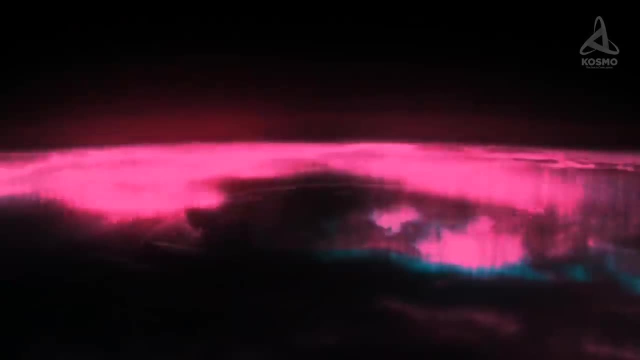 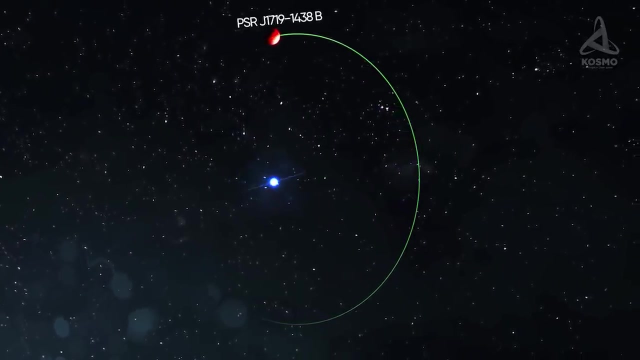 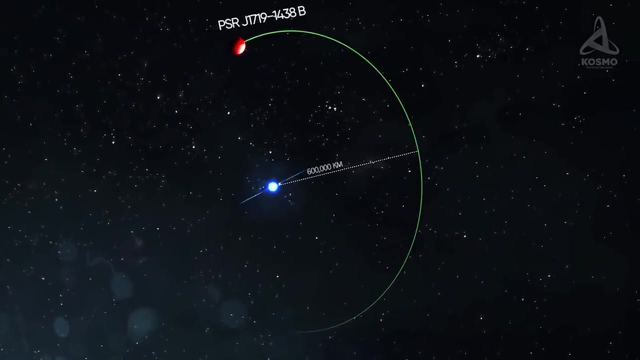 is continuously exposed to these waves of lethal radiation, which makes it a hostile and forbidding place. It takes this planet just two hours to complete a full orbit around its system center, and the distance to the pulsar is smaller than the Sun's radius, just 600,000 km or 0.004 astronomical units. 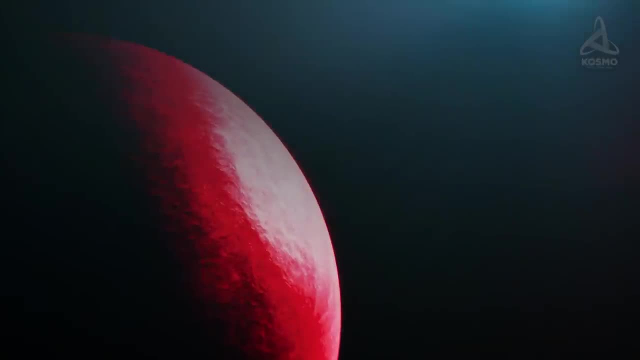 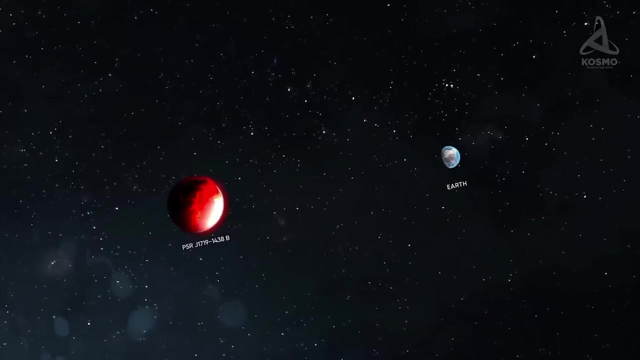 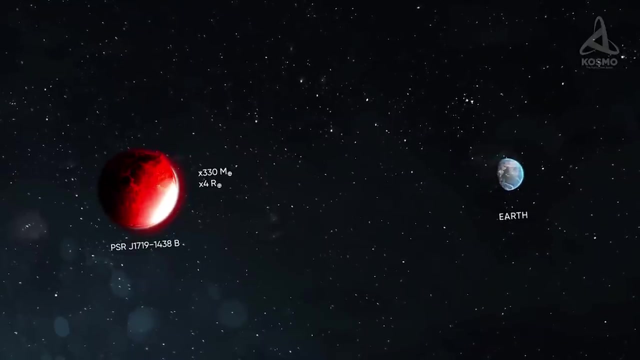 Incidentally, the celestial body's surface is bound by eternal cold and space, as its parent star just barely emits thermal energy. The object's mass is around 330 that of the Earth, while its radius is 4 times that of our planet. This makes gravity on its surface. as much as 20 times stronger than on the Earth. Estimates show the planet's average density to be about 23 g per cubic centimeter, which is more than most chemical compounds we know. The planet is thought to be made up, for the most part. 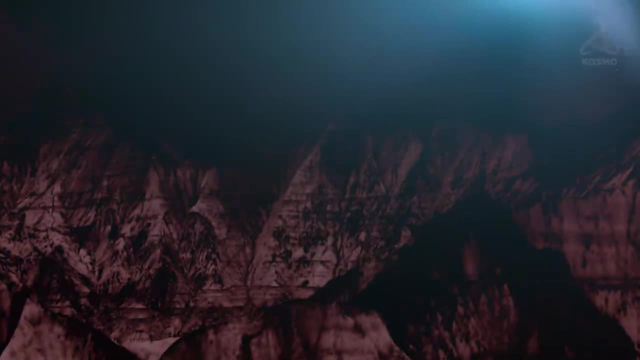 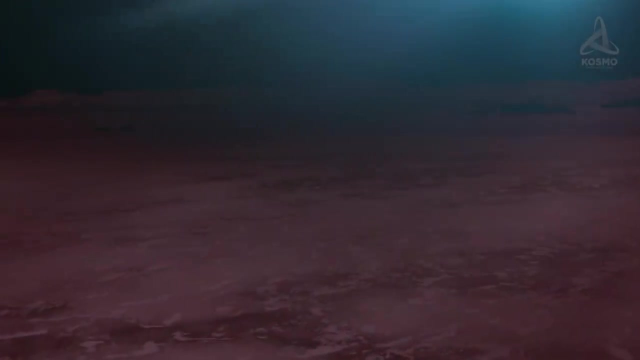 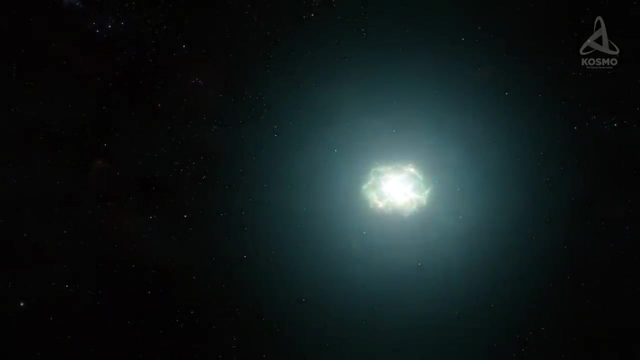 of crystallized carbon under a lot of pressure. Besides, the object's upper layers contain some oxygen which is probably chemically bound with carbon. It is highly doubtful that a celestial body located so close to a star could possibly have survived a supernova event. 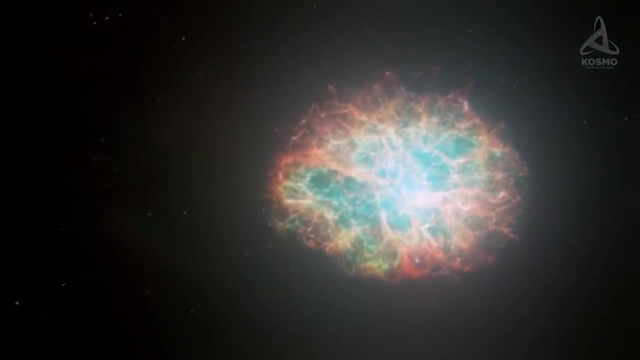 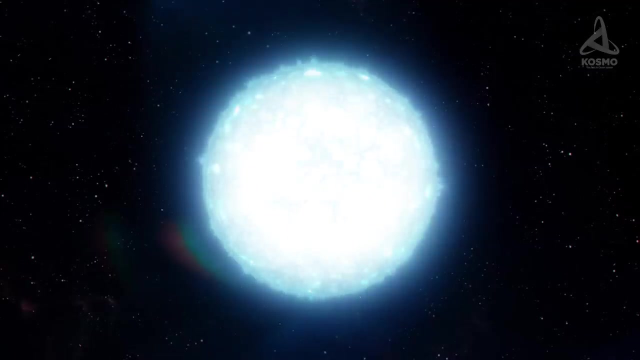 It is more realistic to assume that the exoplanet formed after the progenitor star had come to the end of its life cycle and had transformed itself into a pulsar. The exoplanet could be a piece of debris left over from a white dwarf. 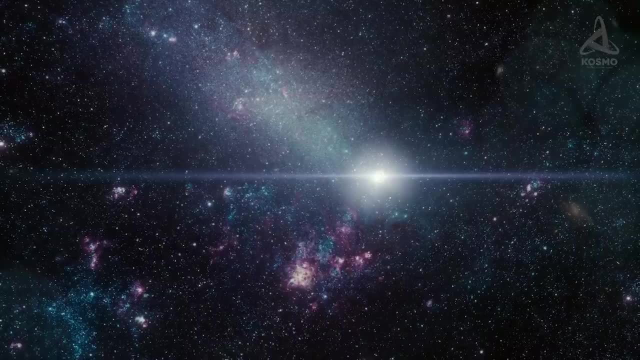 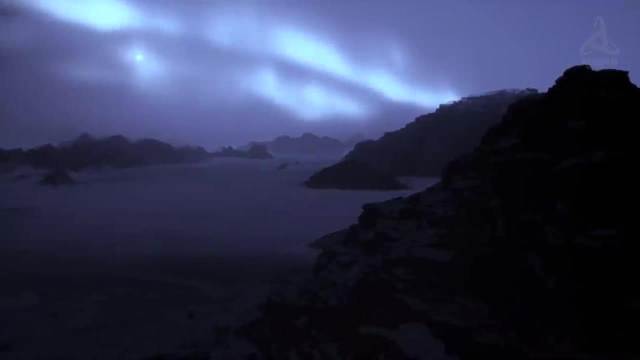 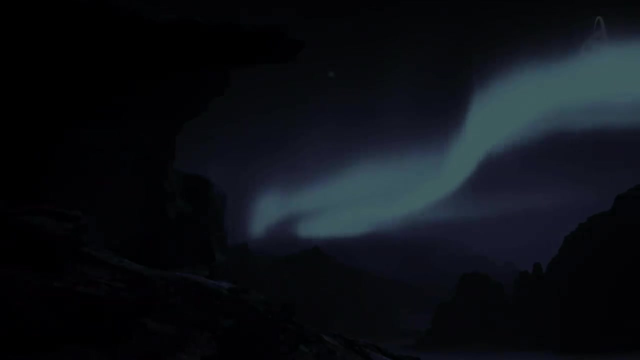 whose material would have dispersed for the most part. This makes classifying the exoplanet an especially difficult task. Still, whatever it is, this world remains one of the most dangerous and hostile ones, lurking in the depths of the cosmos, Amazingly, even having covered thousands. 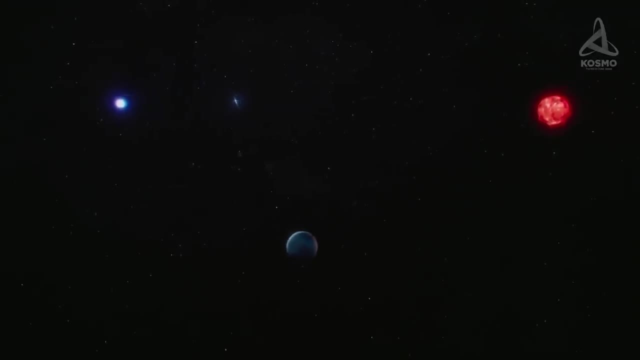 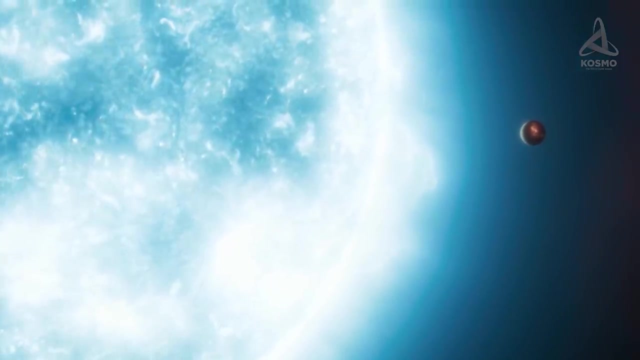 of light years. we have made acquaintance of only a miniscule portion of the endless diversity of our galaxy's exoplanets. Hundreds of billions of other worlds still remain concealed from observation. However, every day we find out more about the Universe.